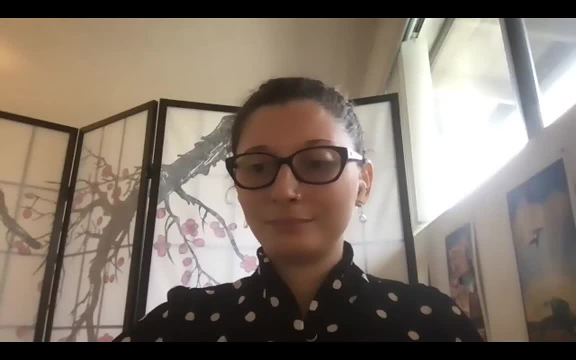 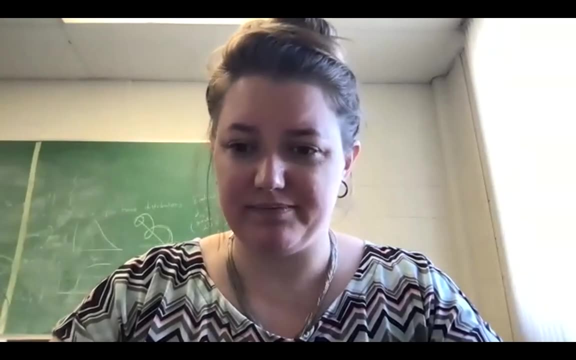 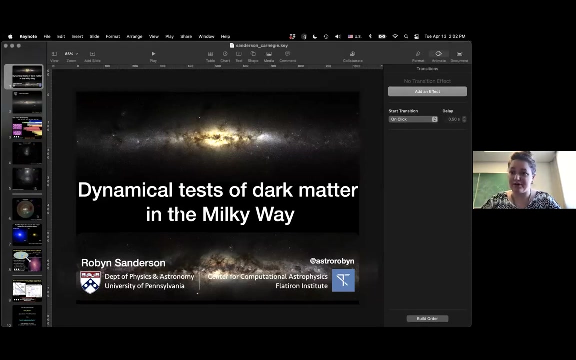 So please take it away, Robin. Thank you, Ivana. All right, Here we go. So I know it's awkward to ask questions during colloquia on Zoom, so I'm going to try to pause after each sort of third of this talk. 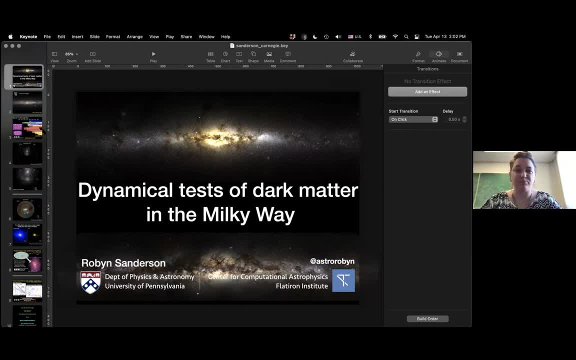 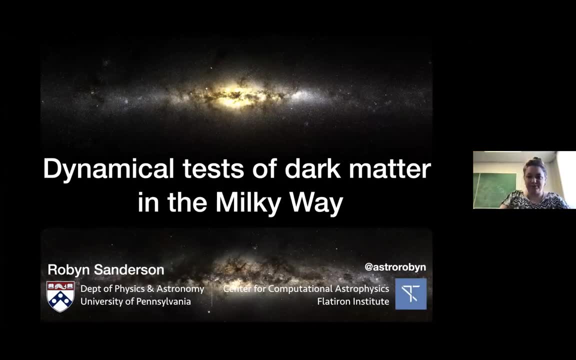 But, Ivana, if you see any clarifying questions, come up, just flag me and I'll stop. Will do All right. So today I'm going to talk about what we can learn about dark matter from the Milky Way through galaxy dynamics. 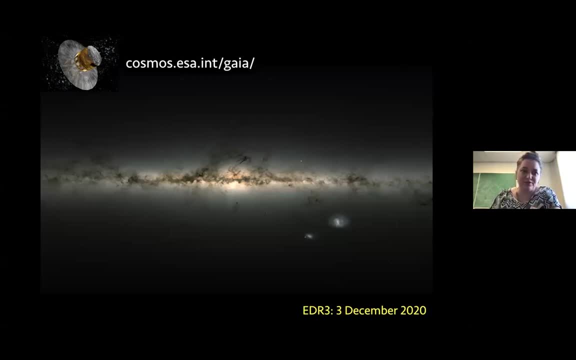 And the situation that we're in today really is a renaissance in this field because of the Gaia mission, which I don't think I really have to describe to this audience. Gaia has been conducting for some years now an astrometric survey of the galaxy. 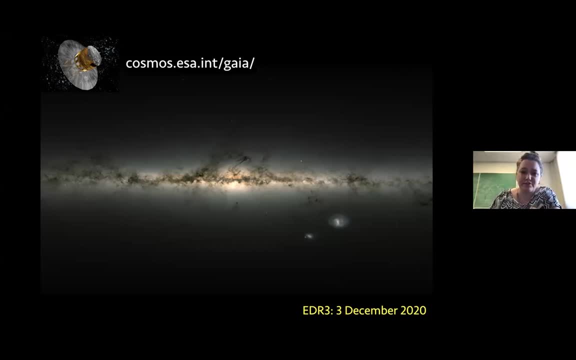 It has observed over a billion stars, all of which went into making the map that you see here, And And It's about to release its third data release sometime in the next year or two, depending on pandemic things, But has been upgrading its ability to measure the proper motions and parallaxes to stars in a volume and with a precision that's a thousand times better, literally, than the data set that we had before. 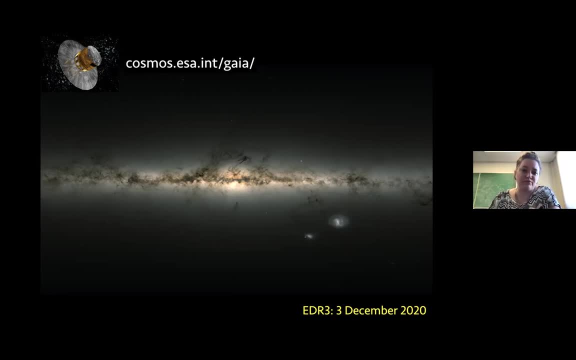 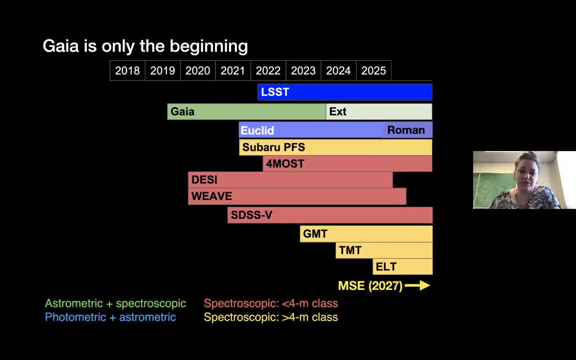 And that's really sparked a revolution in our understanding Of the dynamical state or states of our galaxy. And Gaia is really only the beginning of this new window that we're opening on our, on our Milky Way and on the characteristics of its stars. 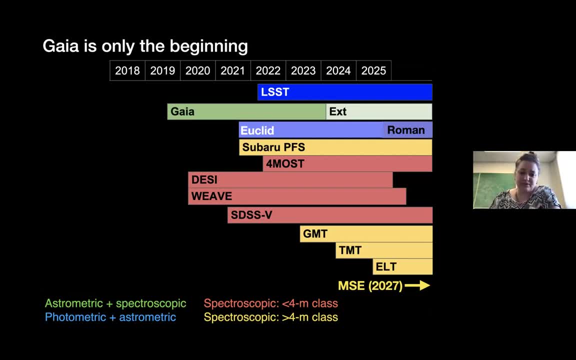 LSST, Euclid, many sort of four meter spectroscopic surveys and eventually some new large telescopes with spectrographs on them are all looking to get underway with a slightly different approach, But we do need to reflect upon a slightly delayed timeline compared to this thing that I'm showing you here. 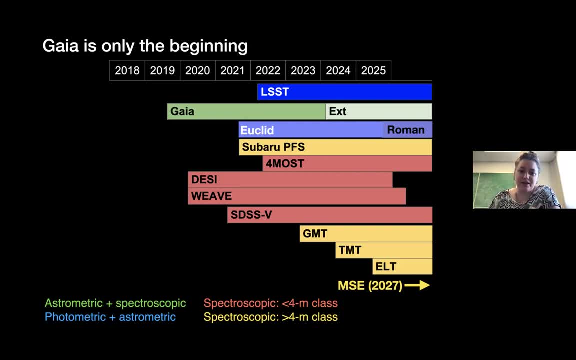 Again thanks to the pandemic. but many of these will, in the foreground of what they might be targeting for their main programs, be capturing the phase based distribution of Milky Way stars and also information about their chemical compositions. So I think it's not crazy that in another nine years we're going to have six dimensional phase based information. 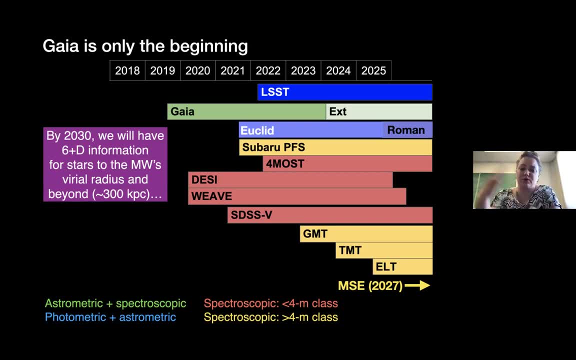 plus abundances for stars all the way to the Milky Way's virile radius and probably beyond. And as we improve our space-based capabilities with the Roman Space Telescope, which isn't even on this timeline, we'll be able to make resolved stellar maps, not just of Andromeda the beautiful. 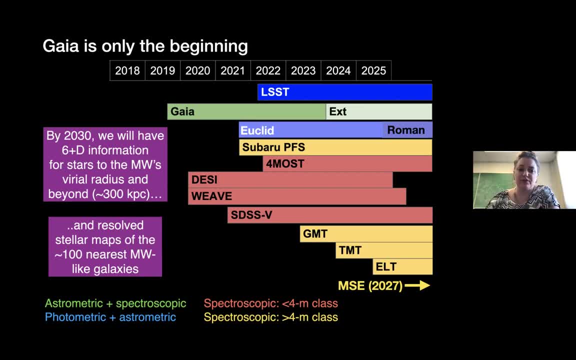 work that's been done there, but similar maps for up to 100 nearby Milky Way-like galaxies, And so we're really transitioning from a detailed information in phase space only from a handful of stars near the sun to a full galaxy view over the next decade, And we're going to be 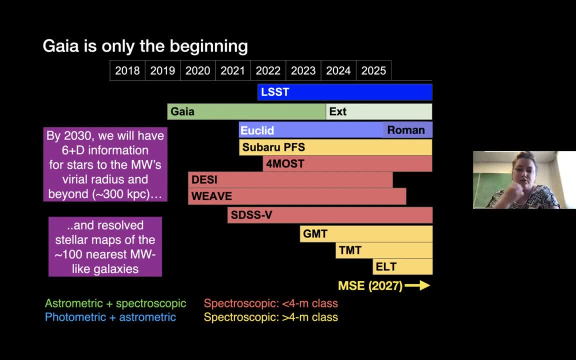 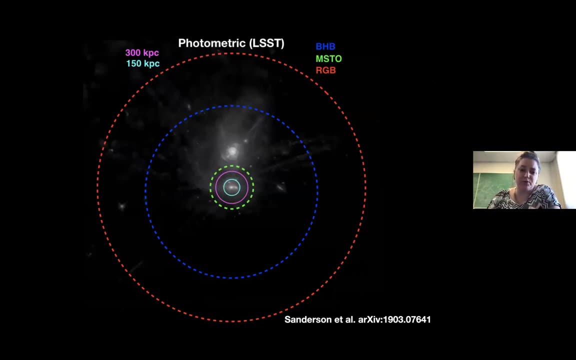 able to connect it, using resolved stellar maps, to the population of galaxies of which the Milky Way is a member. So I just want to show you what that looks like in a few different stellar tracers in terms of volumes. So, LSST, I've superimposed these here on an image generated from one of our cosmological 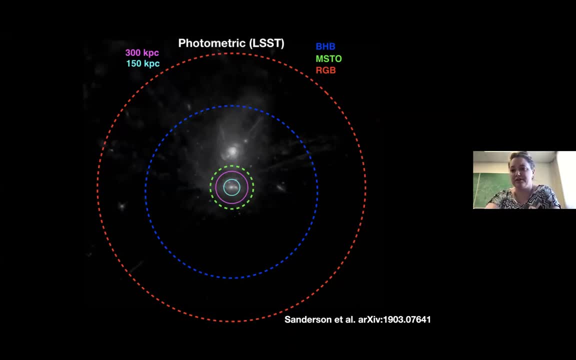 simulations of a pair of galaxies like the Milky Way and Andromeda, And in this image they're separated by about the physical distance that that pair is in our galaxy. But of course we don't have this outer view, And so these circles sort of show how far you can see different. 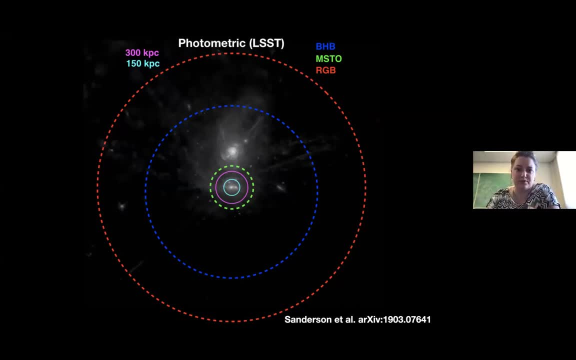 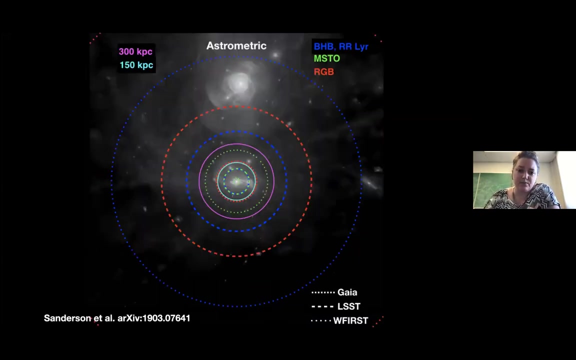 tracer stars using different instruments. So LSST will be able to see RGB stars all through the local group And we'll see main sequence stars out to the edges of the of the Milky Way's virial radius. A lot of missions are going to get various qualities of astrometry over the next decade or 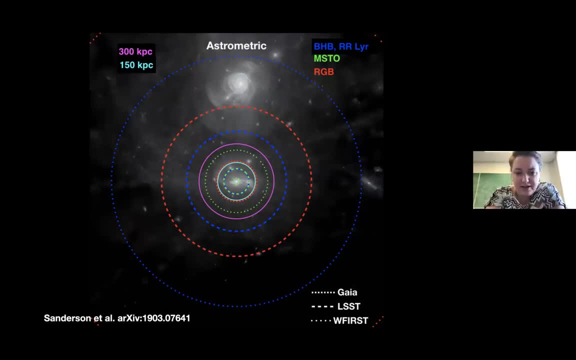 so If you focus on the dashed lines in the center of this, those are sort of the distance to which Gaia measures proper motions for RGB stars here. Can you see my pointer? Yes, I can see. Okay, good, So RGB RLIRY and main sequence turnoff: LSST is going to get pretty high quality. 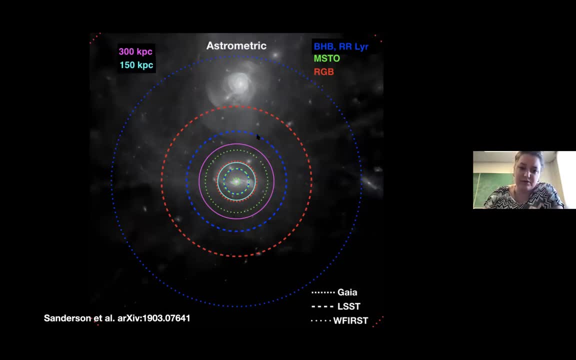 proper motions, based on some work that's been done with current surveys to optimize the ability to do ground-based astrometry, And we'll see RLIRY way out here And RGB will be able to see RGB stars even further with usable proper motion data And finally, the now Roman satellite. when 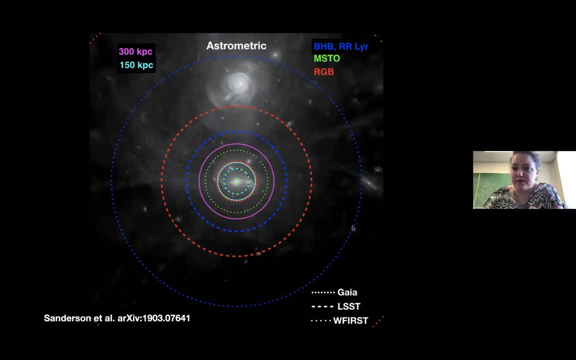 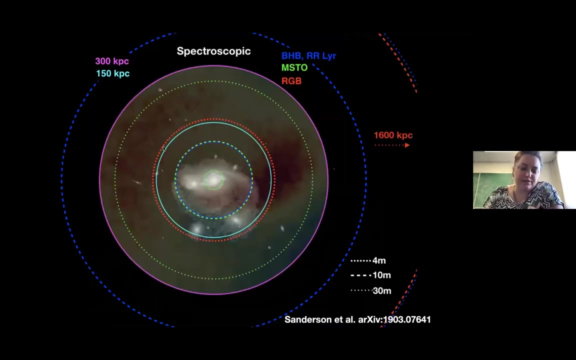 it launches will be doing a survey of a big chunk of the sky for for weak lensing purposes, But in the foregrounds we'll be able to pick up proper motions of Milky Way stars out to very large distances. And finally, in terms of spectroscopy, the missing. 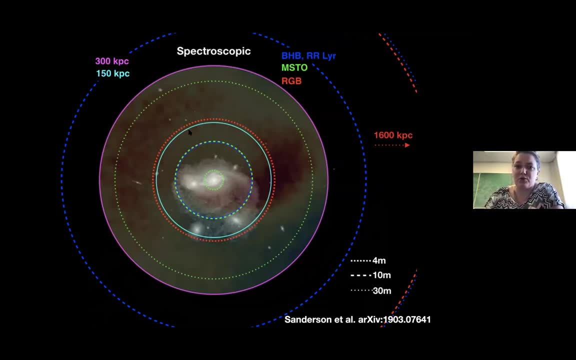 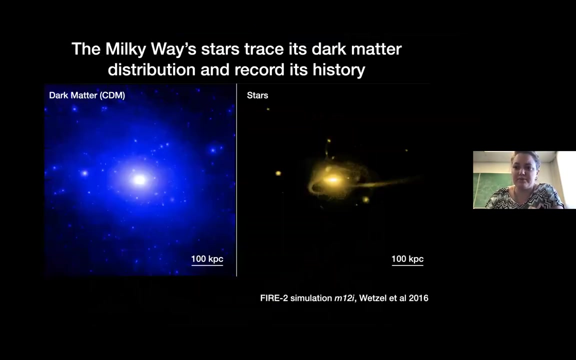 components that aren't established either by photometry or astrometry. the missing components in this picture are also going to extend to much larger distances as the decade goes on, And so this picture is going to get a lot more complete and more connected in its cosmological context than we've been able to see before. So the reason I care about this 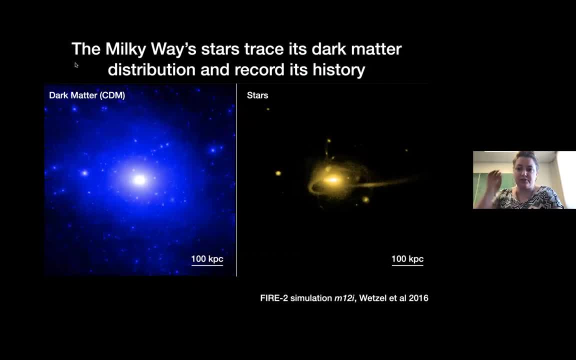 is that the Milky Way's stars are our best tracer of its dark matter distribution and of the history of our galaxy, which is equally sensitive to the type of dark matter that we have in the universe, or at least in our galaxy. And so here's a snapshot from one of the simulations. 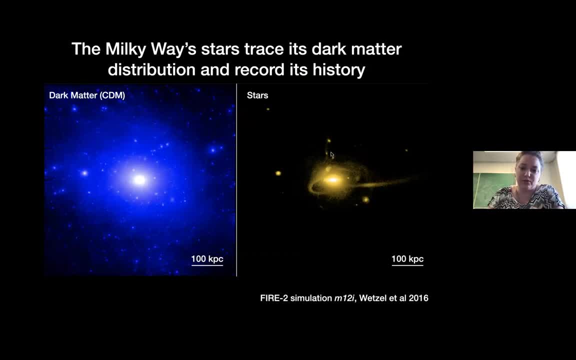 that I work with from the FIRE-2 collaboration. So this is a Milky Way mass system that was formed from cosmological initial conditions and run to the present day, And here in the picture you can see that the Milky Way's stars are our best tracer of its dark matter distribution. 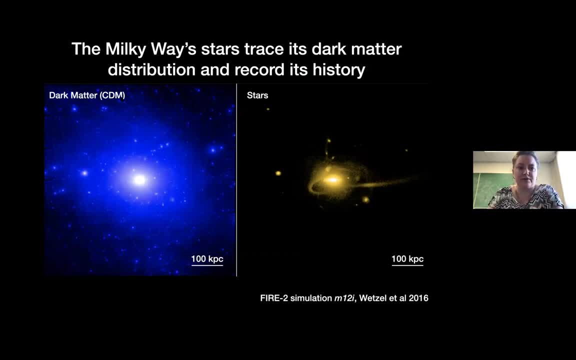 In blue you see the dark matter, which in this particular run is a cold dark matter model, And in yellow- here you see the density of stars in the same simulation. So you'll notice that it's a biased tracer of the dark matter, but that some stars are definitely more useful. 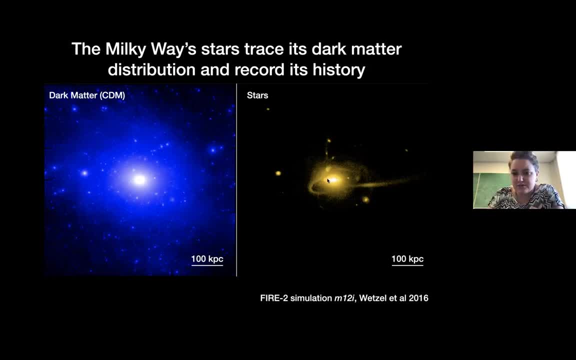 than others. So in the center of this you see the disk here, But at larger distances, where it's mostly dark matter, if you compare the two, you see individual sort of point-like tracers in the bound satellite galaxies you see here And then also tidal streams that are unique. 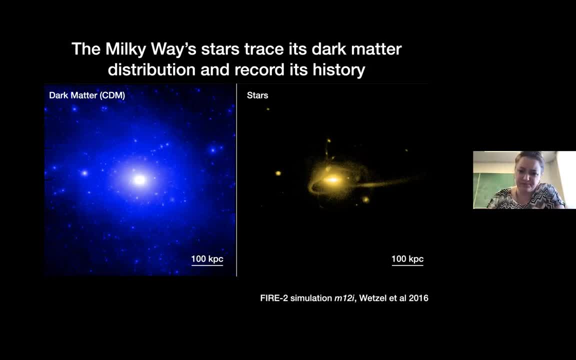 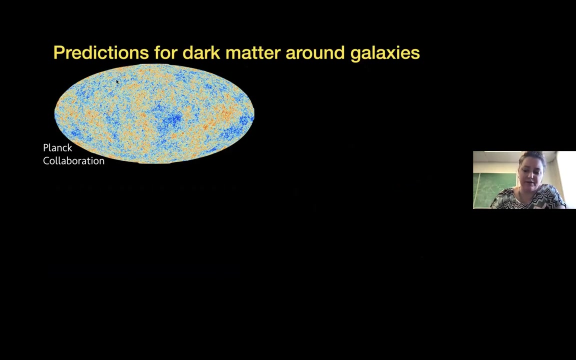 and extremely useful at probing these outskirts. Since they're stars we can associate all with the same progenitor, galaxy or globular cluster, And we therefore know that they must be on similar orbits to one another to start off with, And so So, to give you a little bit more background about how you get from this to this, it's basically 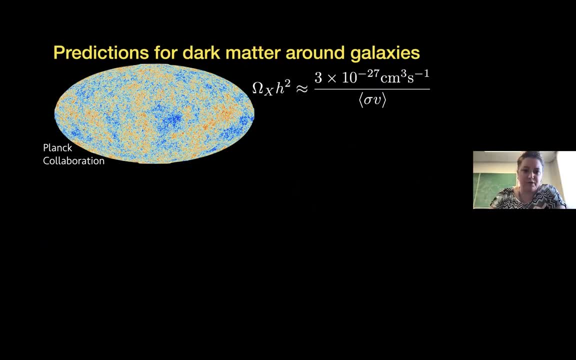 at the lowest level, a big initial value problem. So you pick your initial conditions, which Planck has and other such missions have kindly measured for us. You pick your dark matter model that sets about how much dark matter you have and any interactions that it has. 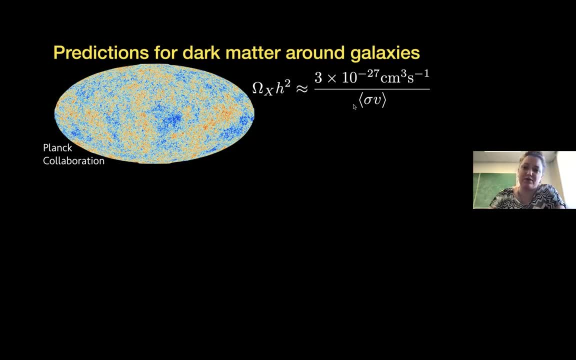 in the dark matter model. And then you pick your dark matter model that sets about how in the late times, So in cold dark matter, the cross-section of interactions between dark matter particles just sets the amount and then is ignored in the late universe because those 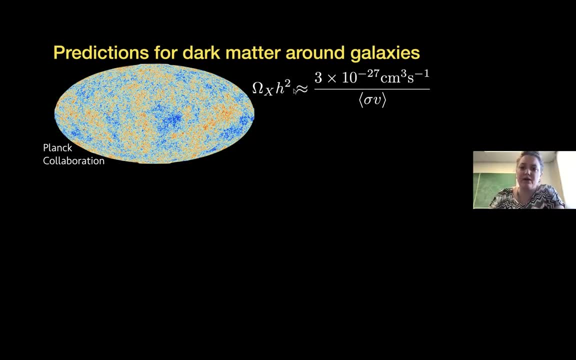 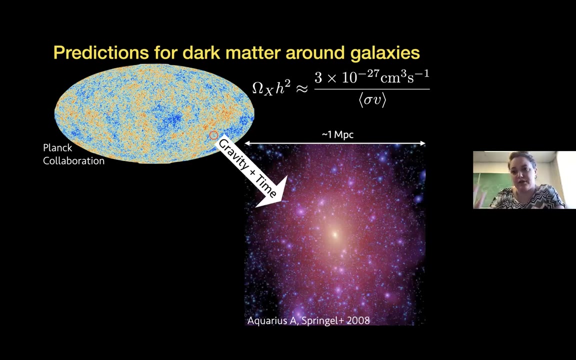 interactions are not very common, But in other models that's not necessarily the case. Then you pick some region of this map and populate it with your n-body particles. You add gravity and time and you get a prediction for what the dark matter distribution should look like. 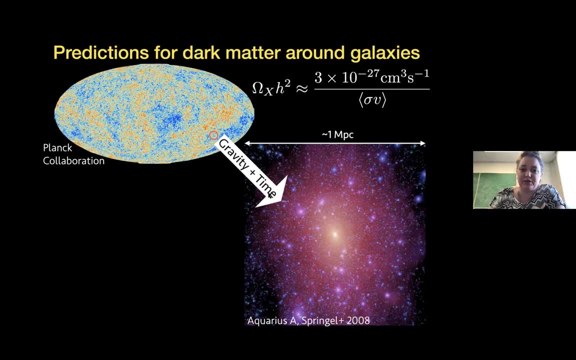 I didn't include in here anything about the stars or gas content, because the simplest version of this problem is just to simulate the dark matter itself as collisionless particles. This view of the Aquarius simulation, which just did that for Milky Way mass galaxy sort. 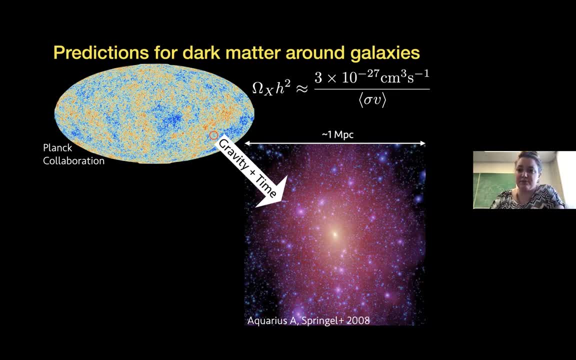 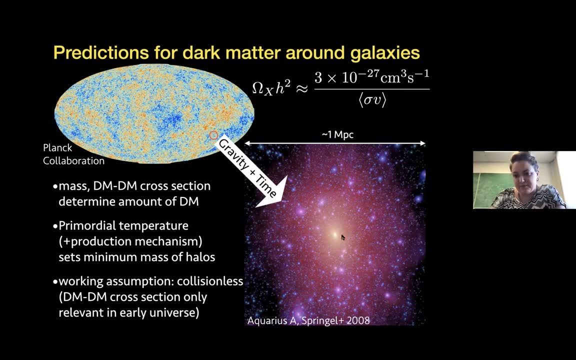 of summarizes some of the different predictions that this type of work can give. You can see here that it predicts that the main halo, which is this large thing, is triaxial, not completely spherically symmetric. It has a very dense core and then you see lots of other little blobs that are sort of self-similar copies of this at smaller mass scales, with a dense center, outskirts that fall away. 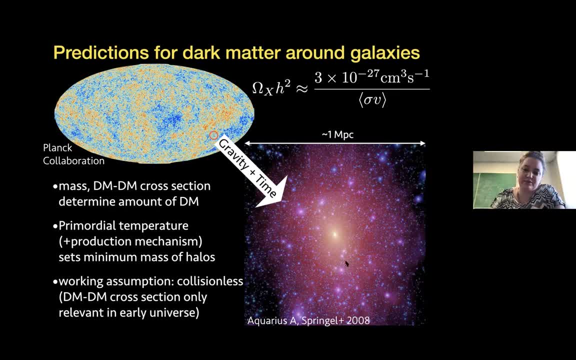 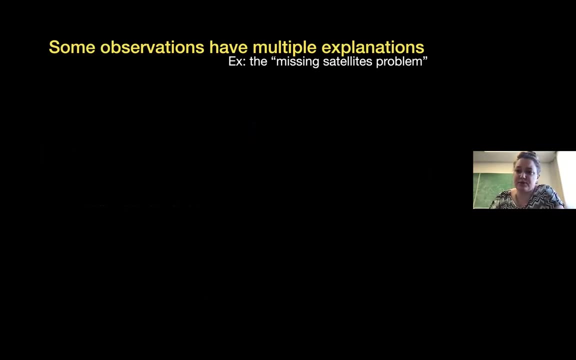 And the structures that you see here come on many, many different mass scales and size scales, And so those generic predictions are what we start with when we try to compare with what we observe in the Milky Way. But some of the observations that we make when we try to make that comparison can have multiple explanations that impinge upon our ability to determine properties of the dark matter. 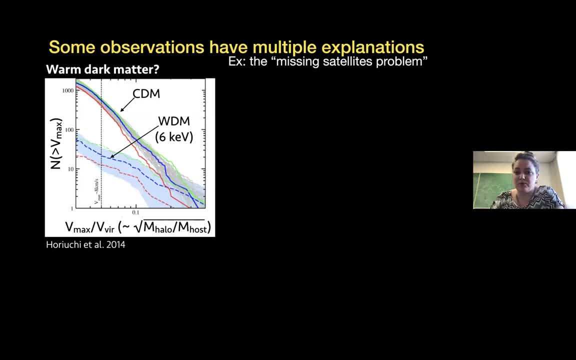 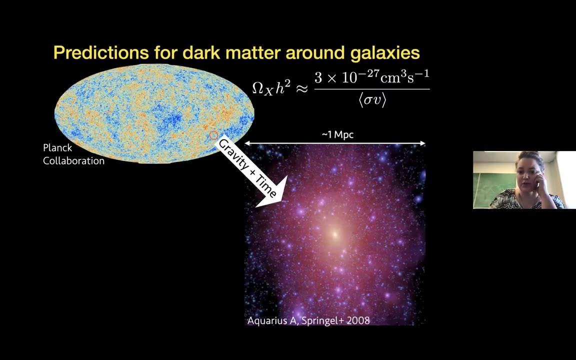 So an example is the so-called missing satellites problem, which now most people would agree has been sorted, But it's a nice illustration of why This is a difficult question to answer. So we see far fewer actual satellite galaxies in the Milky Way than you can see little blobs of dark matter in this image from the simulation. 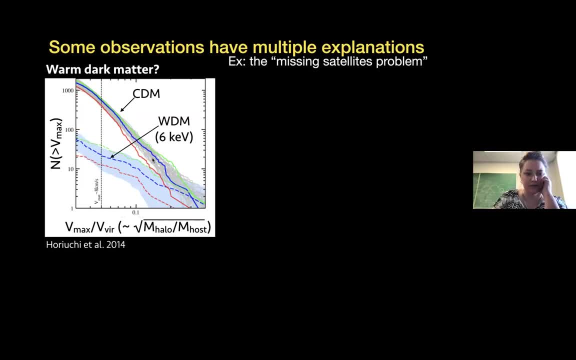 So these lines on the top here are the prediction of how many subhalos- you know little substructures in the Milky Way's main dark matter halo- you expect to have as a function, sort of a square root of their masses. And since we don't see all of these lit up, 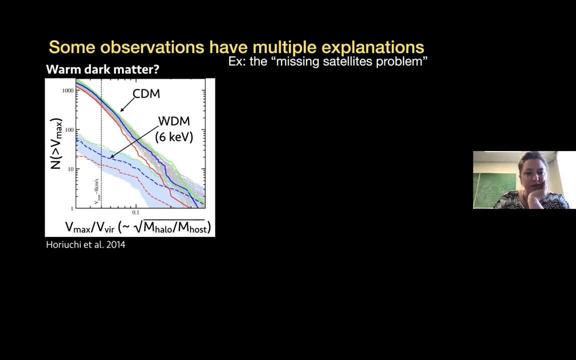 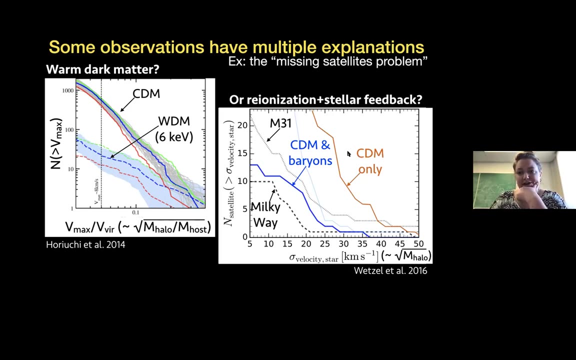 stars, you can. you can change the dark matter model by adding some primordial temperature to it and that cuts off a lot of the structures and small masses and starts to reconcile with the number of things we actually see. Alternatively, you can add stars and gas to your simulation and then a combination of reionization energy and feedback from star formation can give you the same overall effect. 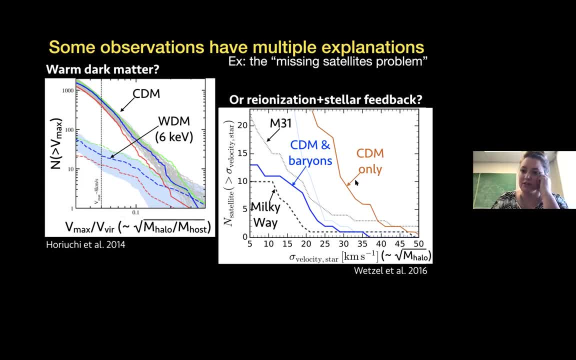 in the sense that now you still have all those halos. it's just that most of them don't light up with stars because they don't form enough stars, either Because they're so small they can't hold on to their gas during reionization, or because stellar feedback cuts it off later on. 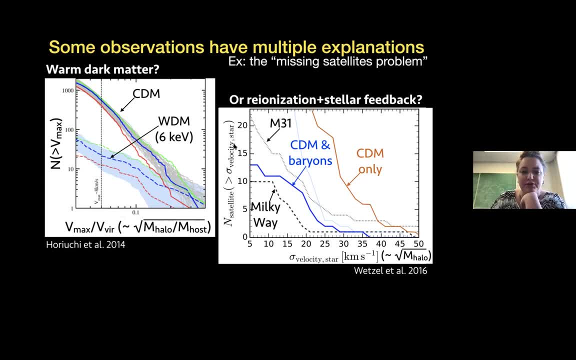 And then you end up with the same, with with a commensurate prediction for how many satellite galaxies you have. So the reason I bring this up is to illustrate how the process of galaxy formation is linking the dark and the star, linking the dark and the standard model sectors, here through gravity at least, if not more. 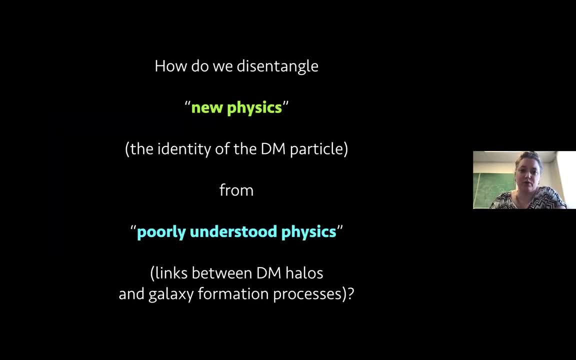 depending on your dark matter model, And so one of the big questions in this field is how we disentangle new physics from stuff that we should understand, like galaxy formation, but in many cases is still a work in progress, And both of these sides of this coin are interesting. 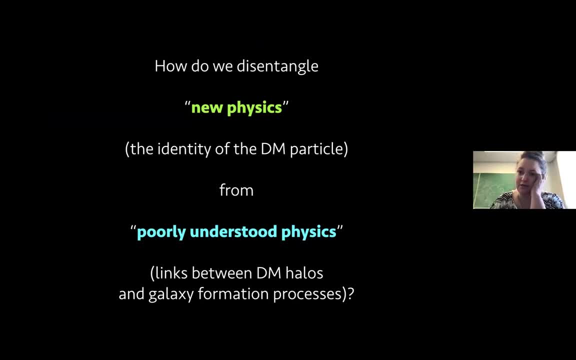 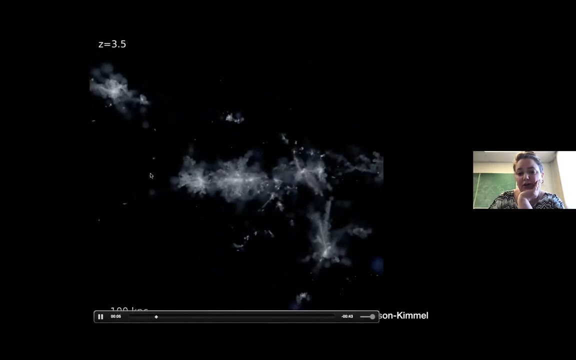 And so it's useful to try to construct tests that are isolating one from the other in whatever ways that we can. All of the stars that you see are relatively sparse compared to the dark matter, So the dark matter is driving the dynamics, rather than in the center of the galaxy. 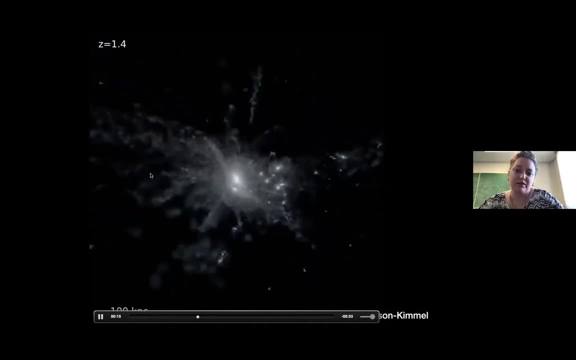 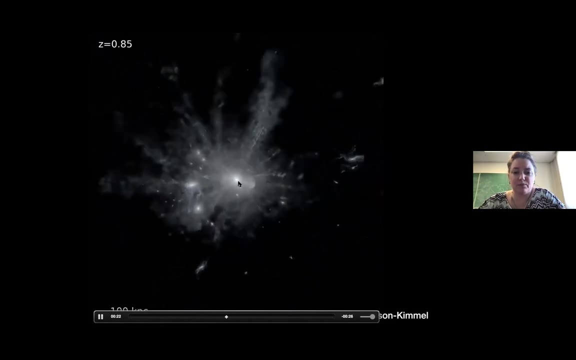 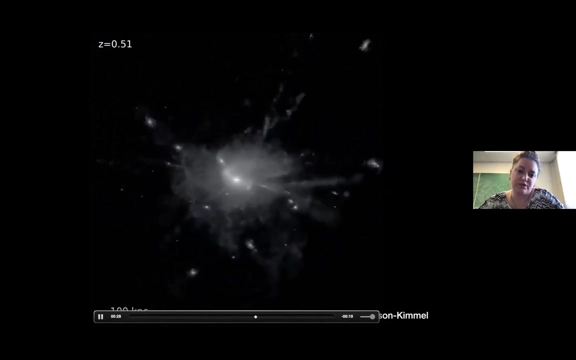 where it's competing with the process of galaxy formation on a regular basis. But you can also see other predictions, like the number of satellites, the rate at which they merge, in, the way in which they tidally disrupt to form tidal streams- All of those things also. 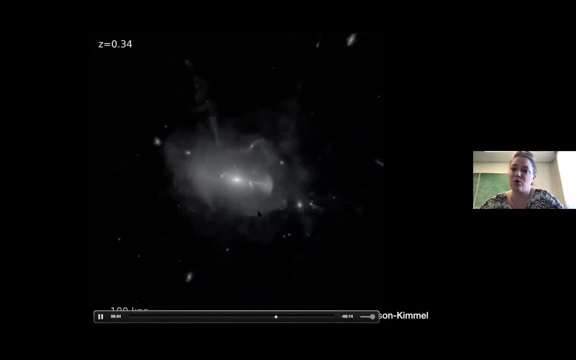 depend on the model of dark matter, because it shapes the whole process of hierarchical formation at every mass scale, And so there's not just one prediction of dark matter that you're going for here. It's not just the mass profile and the shape of the main halo, but also the population. 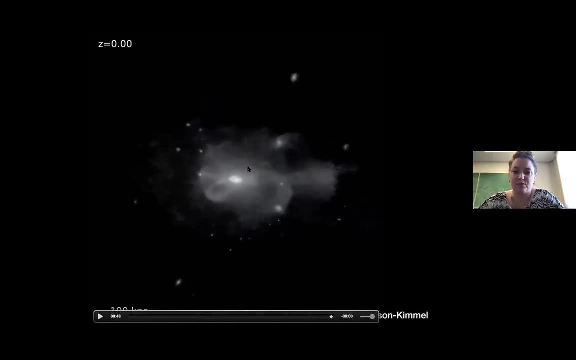 of dark matter, And so that's one of the main things that we're going to be discussing in this: galaxies around it, and the way in which and the number of tidal streams that are formed, and then what happens to those tidal streams and their interactions with whatever substructure. the 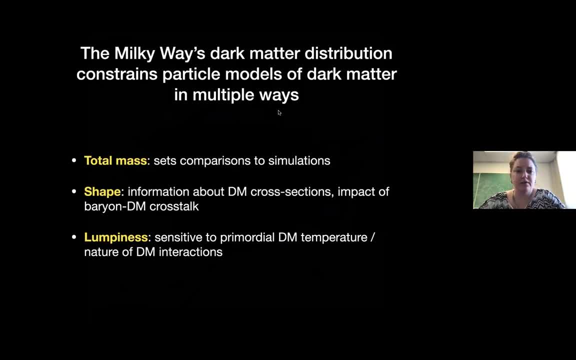 dark matter is making. So I'll talk about three of these things today: the total mass, the shape and the lumpiness, so to speak, of the dark matter halo. So let's deal with the mass first, because this is the zeroth order thing. Really, this is the galaxy we live in. we should get this. 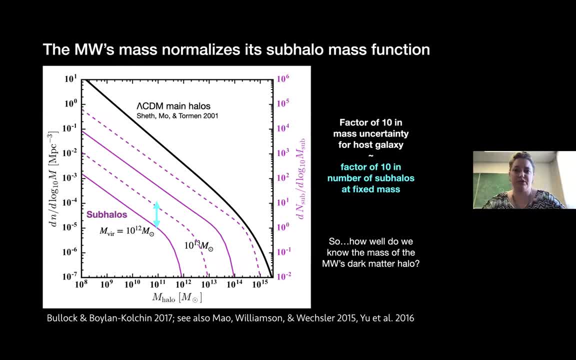 right. And it's especially important because, when you talk about the structures at smaller scales and what those predictions are in different dark matter models, in nearly every case they're normalized by the total mass of the main halo, the one that the Milky Way galaxy lives in. So here's. 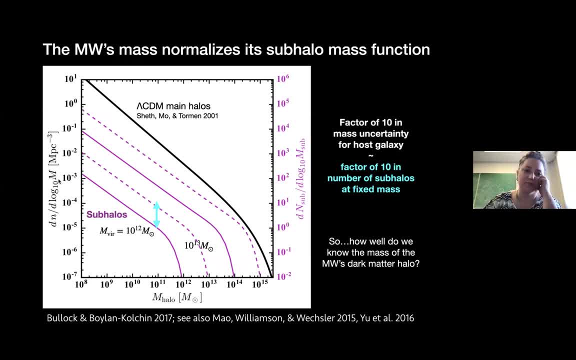 an example of the number of substructures you'd expect at a given mass scale for a different mass main halos And you can see that the difference in the number of subhalos you get is just a linear function of the mass. So if you have a 10 to the 12 solar mass main halo you get 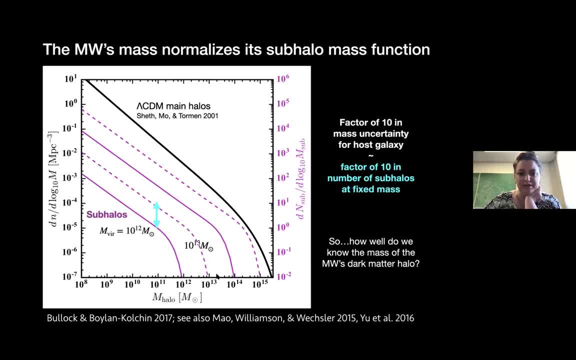 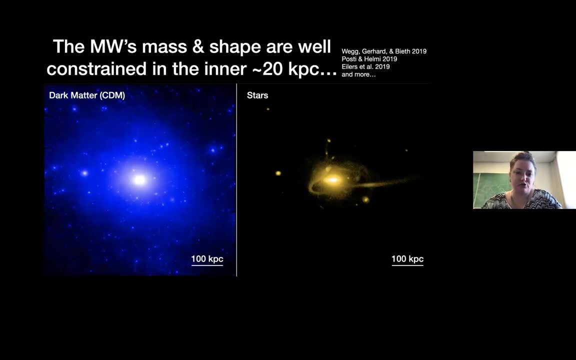 and then you increase the mass by a factor of 10, you get 10 times more substructures. So we have to know the Milky Way's total mass in order to know what simulations and what predictions to compare it with. in the first place, And because of Gaia, which has extreme 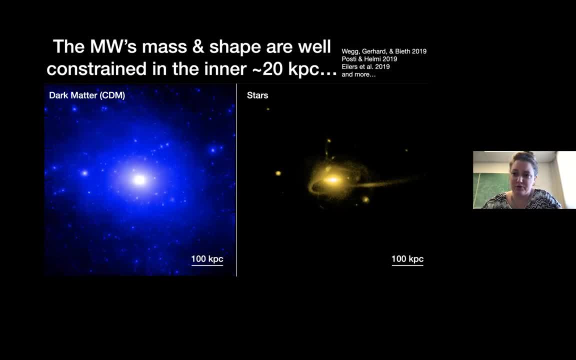 good data in the inner 20 kiloparsecs of our galaxy. we now know and agree on what the mass and shape are pretty well within that region. But if you go back to this example, that's like here. So we have a long way to go before we get out of the region where the process of galaxy formation 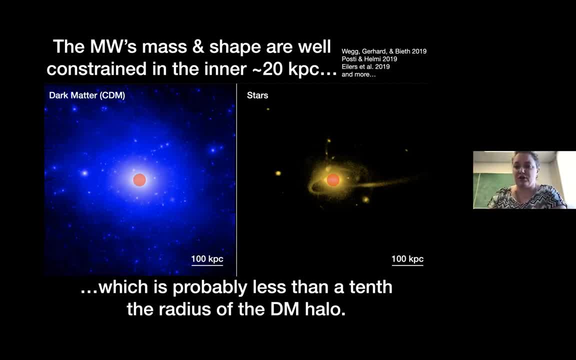 is significantly shaping what's happening in the dark matter, because there is similar mass in stars as dark matter And therefore they are sort of on equal footing as far as gravity is concerned. But then further out you have these nice tidal streams that exist in a place where most of the 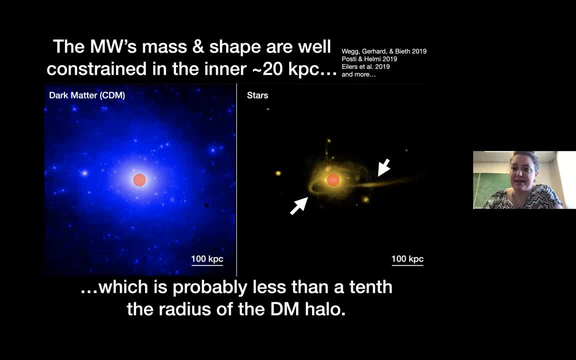 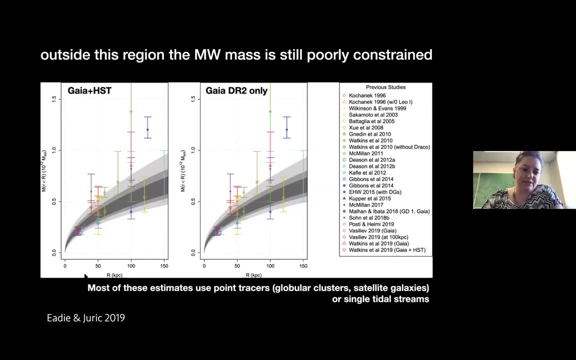 mass is dark matter, and so you don't have as much of a problem disentangling these two types of processes. But in this region, Gaia hasn't made much headway because it just doesn't have a lot of data. So if you look down here, these are two mass profiles derived from different sets of data. 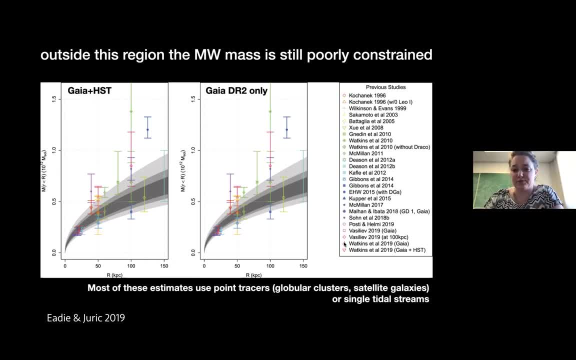 involving Gaia, And here's all the different people that have tried to do this measurement before, And so these are all the different people that have tried to do this measurement before, And the effect of Gaia has been this sort of agreement down here between all of these. 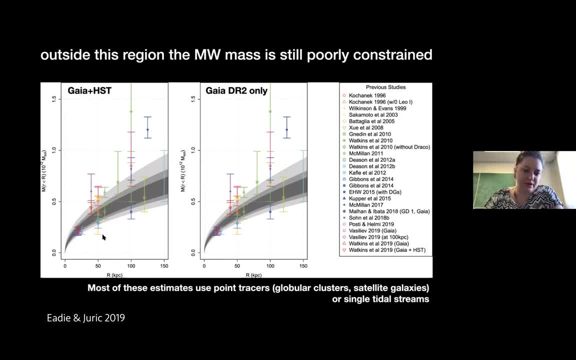 different bars here, And so that's the region where Gaia has data right now. But once you get out here, you see that there's like a factor of three difference between all these different estimates. Part of the reason for that is that most of them are either analyses of point tracers. 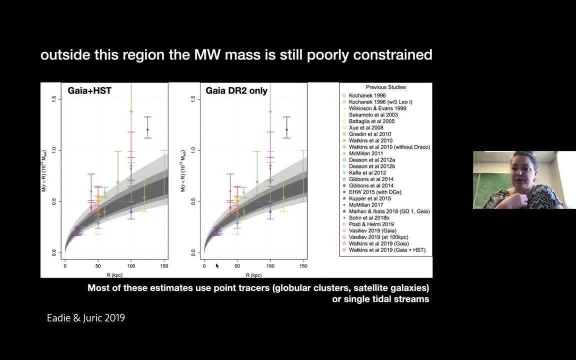 treating globular clusters or systems of satellite galaxies as one big genes model, Or they're fits to single tidal streams And both of those sets are subject to a lot of model degeneracies- In this case of tidal streams, because you're only seeing stars on one family of orbits, through the. 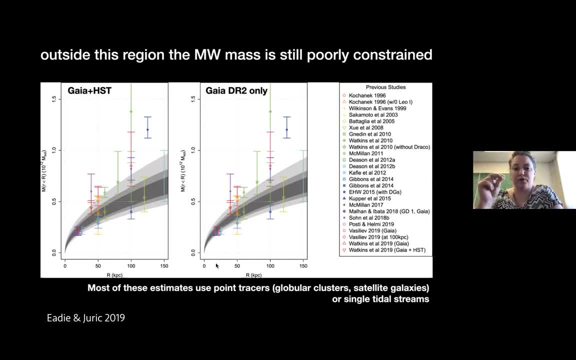 potential And, in the case of point tracers, because it's unclear how well the assumptions for genes modeling are suited to the actual dynamical state of those systems. So we can do a lot better now with Gaia, because we have much more phase-based information about many more tracers. So this is what we were able to do with. 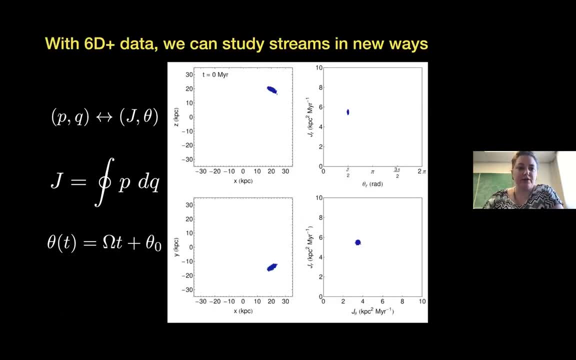 just the point tracers with Gaia, But with the six-dimensional data you can also revolutionize the study of tidal streams. So you can use theorist coordinates instead of observer's coordinates for one, which is where I came into this game. So ordinarily you observe the positions. 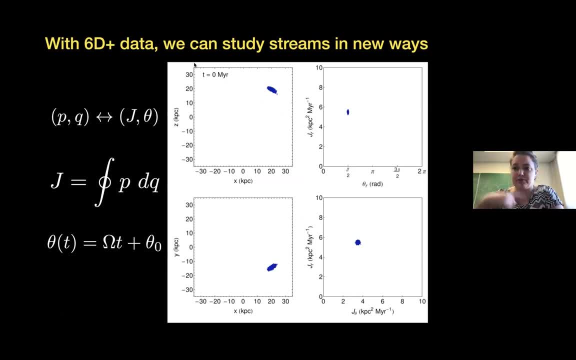 and velocities of stars in a tidal stream And you see that they wind through the galaxy over time. But if you know the potential of your galaxy and you convert those into actions and angles, using this sort of relationship, here for the actions, where p is essentially the stars velocities and q are their positions, This canonical transformation, 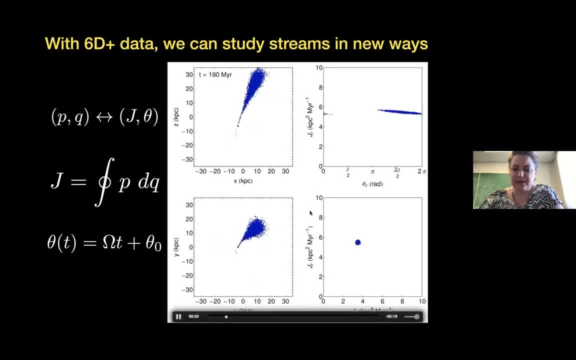 gives you a new view that is much more useful from a modeling standpoint. So in this little movie you're seeing the formation of a couple of tidal streams in different colors over here in position space And you can see that they're moving in different directions And you can see that they're 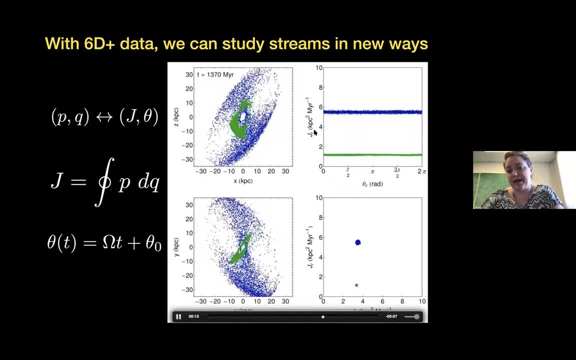 moving in different directions, And you can see that they're moving in different directions In this panel. you see them in one of the actions versus its conjugate angle, And down here you see two of the three actions And you can immediately see that this is a nice simple space to work in. 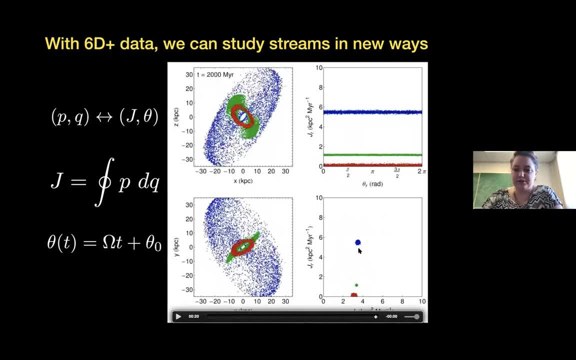 because each complicated mess over here is a nice tight little blob here, because the actions are adiabatically invariant. So even if the galaxy is just steadily growing, they'll continue to be in this nice little cluster. There's no as long as there's no major merger. So this is a nice space. 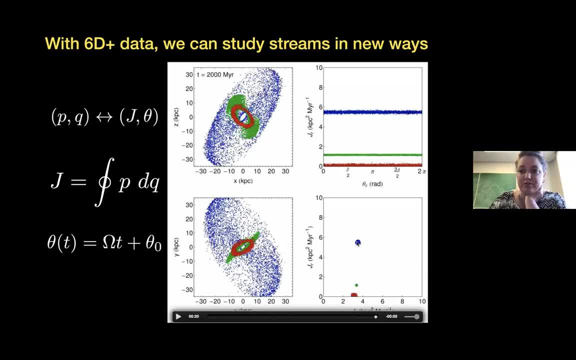 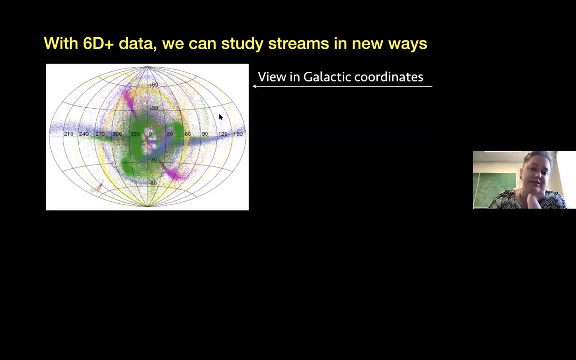 but in order to do this transformation, you need to know the potential, which is the thing that we were trying to measure. If you did know it, you could take all your streams that you see in the sky and then transform them into action space and see a lot of little blobs, Since we don't know. 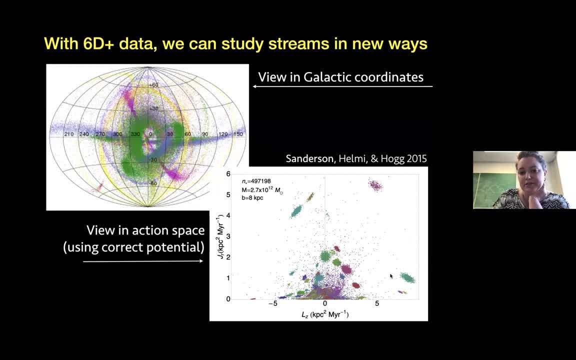 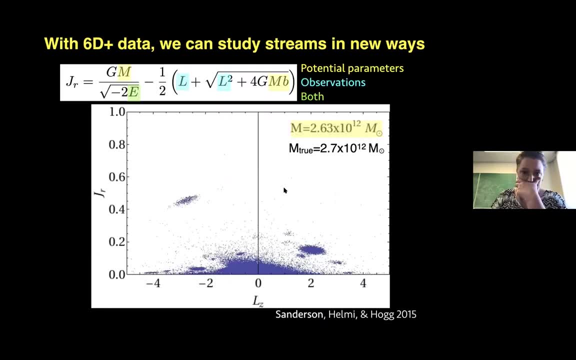 however, we can use the fact that we think the stars in the outskirts of the galaxy should have this form in action space in order to determine what the correct potential is. So, for instance, in this toy model, here's one of the actions, just to illustrate how the dependencies work. 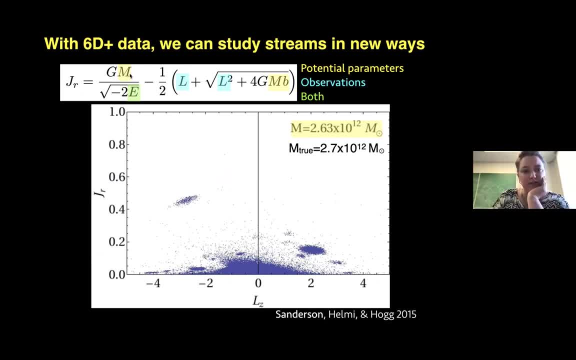 So the parameters of this model potential are its mass and its scale, radius m and b, And then you observe the positions and velocity of a bunch of stars. You use those to compute the angular momenta and the energies, along with the potential model. 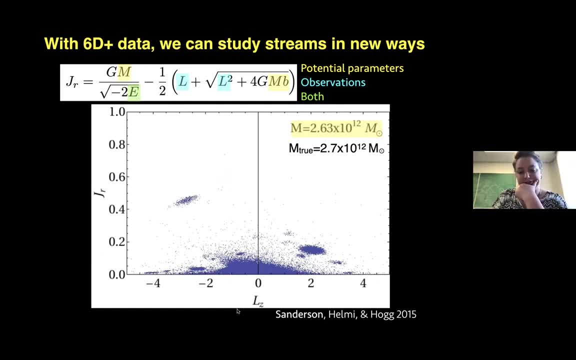 And then you can get this action And then another action. in the system which is very symmetric, is the z component of the angular momentum. So that's plotted here, And so if you guess something close to the right mass you'll get these little blobs. But if you just scroll, 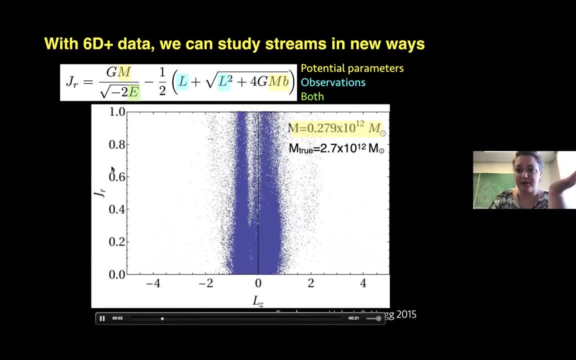 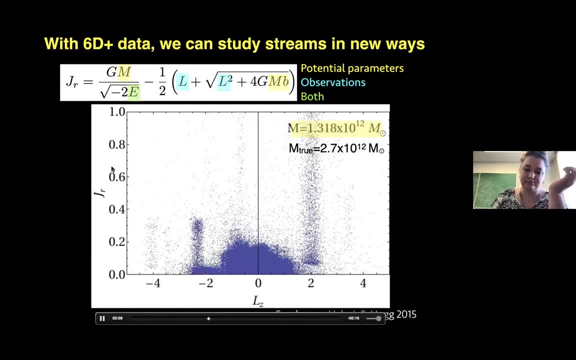 through, you'll be able to see when that happens. Wait for it, And then you can get this action. And then there's another action in the system which is very the right one, right? So you only get that clustering in your stellar halo from all the 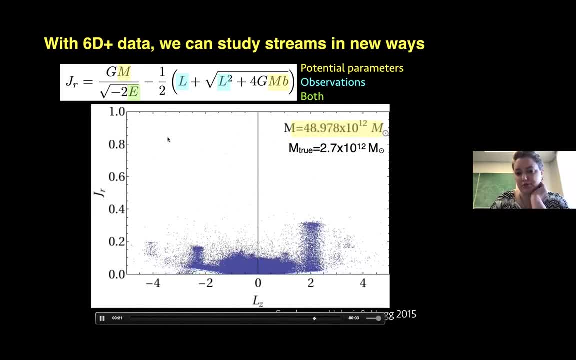 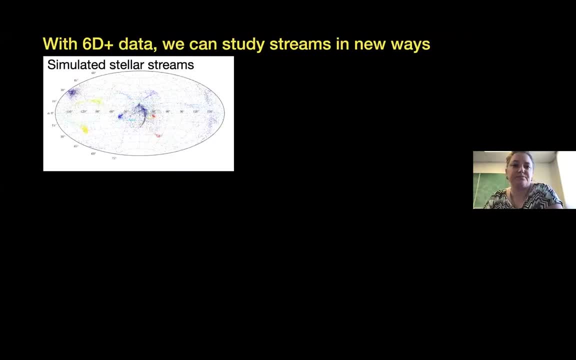 different tidal streams that built it up. if you're close to the right potential model, And so you can quantify the amount of clustering in this space and use that as your figure of merit for the fit, And so you might be wondering: okay, well, this was a toy model. What really happens? 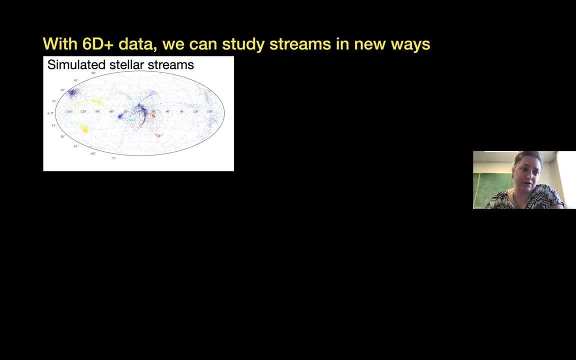 in like a cosmological halo. So a long time ago now, goodness, I did a test of that. Um, so these are simulated stellar streams that were made by tagging a dark, the dark matter only. simulation of a Milky Way galaxy that I showed you in the beginning, the one from Aquarius. 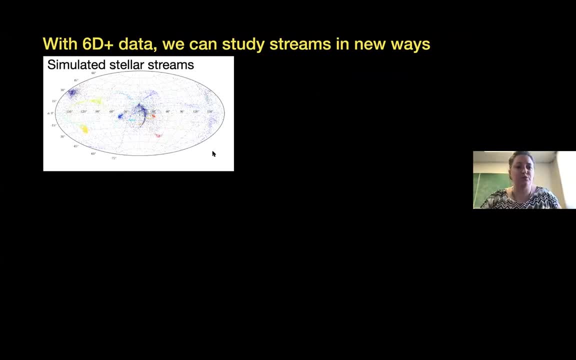 This is before a fire, Um, and so this is the best we could do. but the, the galaxy that these streams evolved in was time dependent. It was, it has lumps. It's not got any prescribed symmetries, So you might wonder whether the Anzac of action space still works in this, uh kind of situation. 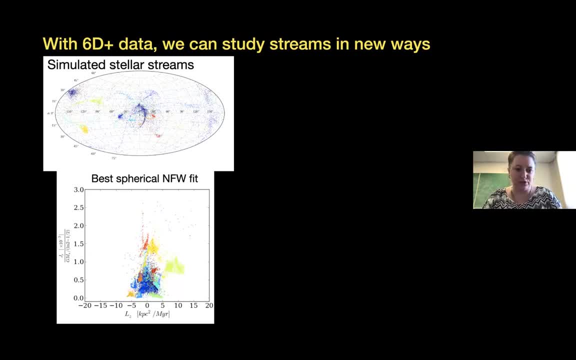 And in fact it does. So I painted all the streams here So you could tell which stars belong in which one, And indeed they form slightly more complicated looking clumps, but still clumps in action space, And in fact this, the potential that we use to calculate these actions, was an NFW profile fit to. 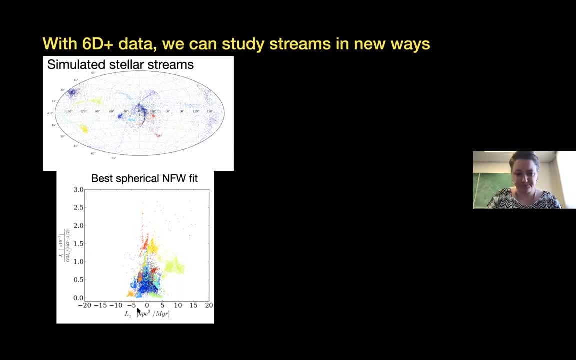 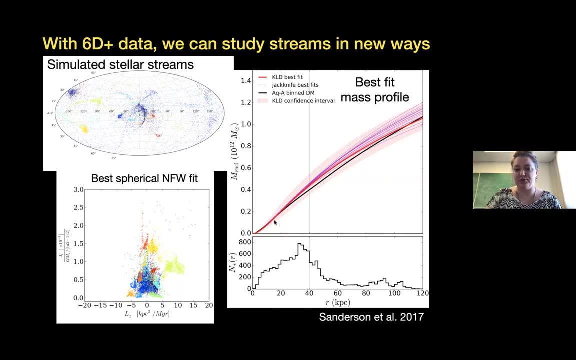 the halo by maximizing this clustering, And if you compare our best fit, which is in red, to the black line here, which is just the bin to dark matter distribution, you get pretty close. So the caveat is is that most of the stars that we use for this test, star particles um, are pretty far beyond. 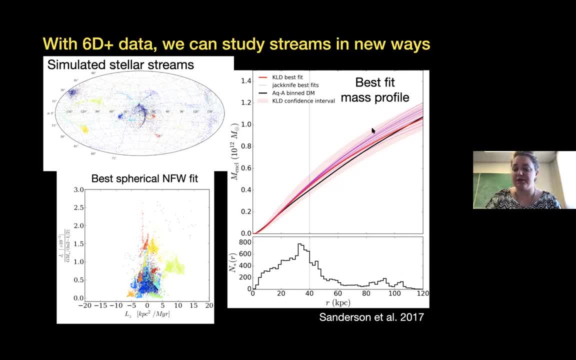 what Gaia can measure, And that has a lot to do with how well the fit converges, even at large distances, because basically you'll get a good fit within the range where you have data. So Gaia can get out to here- Again, we agree on that pretty well with all these four meter spectrographs. 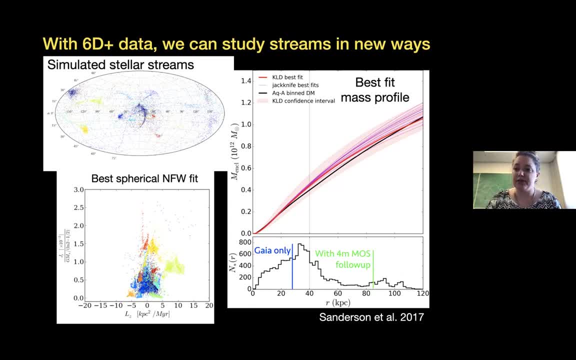 that are coming online. We'll be able to see a lot further because they'll complete the radial velocity information. And then we'll be able to see a lot further because they'll complete the radial velocity information that Gaia doesn't determine for stars at the faint end of its uh. 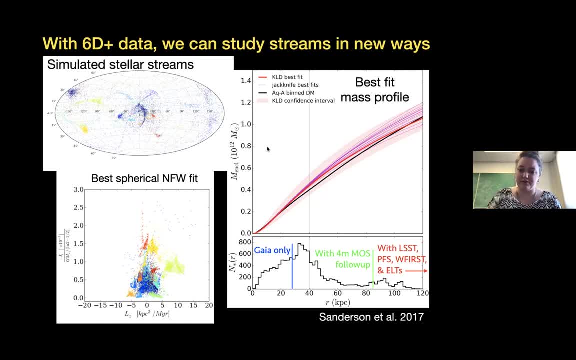 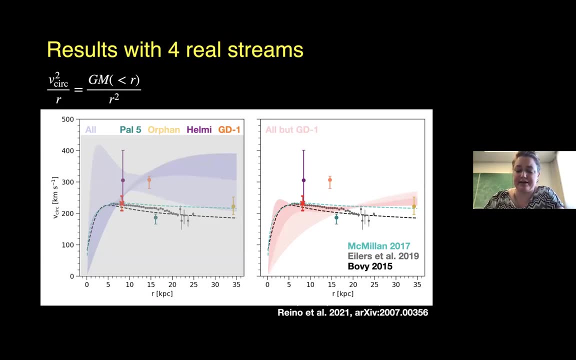 range And then beyond that we can sort of cobble together the last few things out to half the virulent radius or so, um, with the other missions that I mentioned earlier. But in the meantime here are some of our first results of applying this technique, uh, to actual data that we 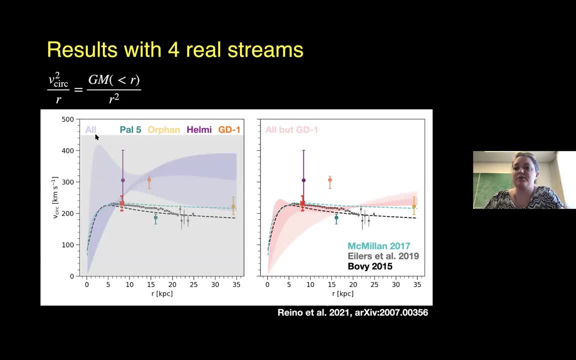 assembled partially from Gaia and partially from other sources, as we could um for a series of uh known streams with known membership, Um, and so these are the rotation curves that we get when we fit the phase-based distributions of these four streams by requiring them to be the most. 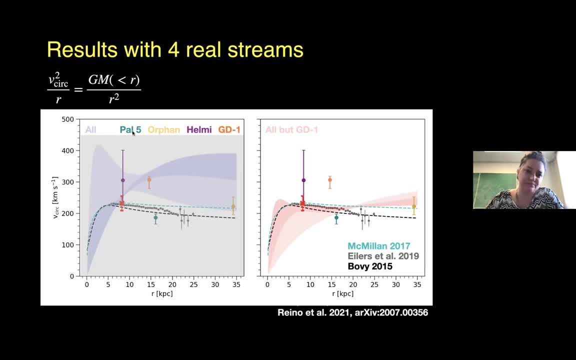 clustered in the action space of the best fit potential. Um, so this side is kind of grayed out because, uh, we're updating this plot at the moment, but if you don't, so GD1, the Grilmero-Dianatos. 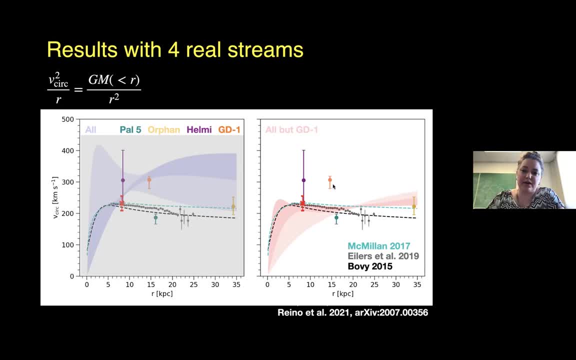 stream is somewhat of an outlier in terms of its uh best fit velocities, And so if you throw that one out, then you get this red uh set of constraints by using the other three, So the Orphan stream, PAL5, and the Helmi stream. Um, uh, a little uh with respect to other estimates. 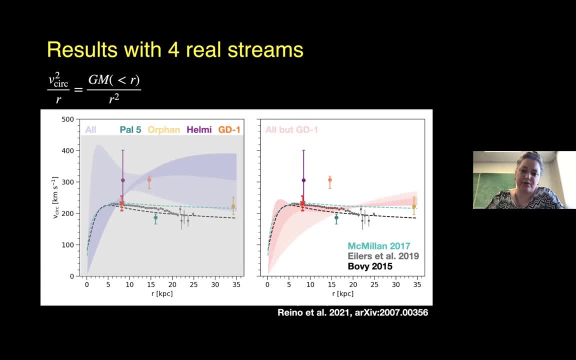 down here that you see, Um, and so we're now pretty convinced that this one is going to be going to work. This will work not only in in simulations, but also in the real galaxy. Here we had a lot more information than you necessarily need to have for this technique. 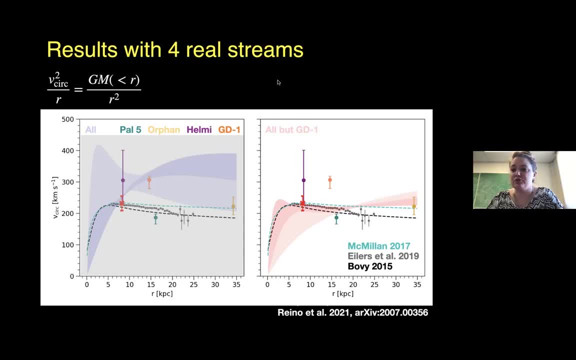 You don't always have to know membership, but if you do, it helps you because you can then um use the membership information as part of your uh, part of your fitting procedure. You know exactly which stars should belong in which clump, as well as how many clumps there are. 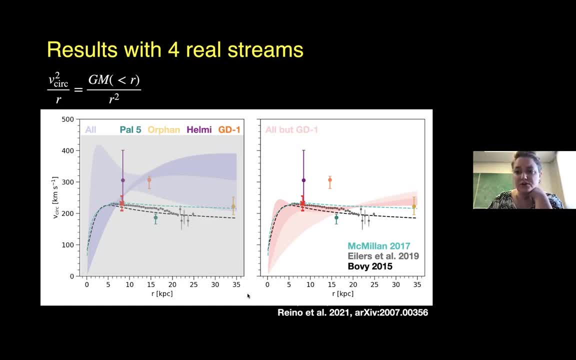 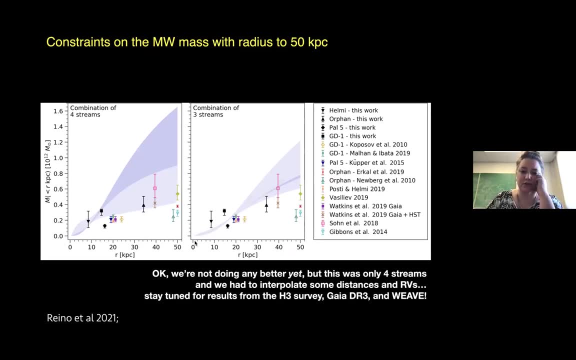 which helps you when it comes to the determination of the clustering. So we're not really doing that much better yet. in terms of uh constraining the mass, You can see this result here. uh is not been completely updated. The actual curve is a little lower. 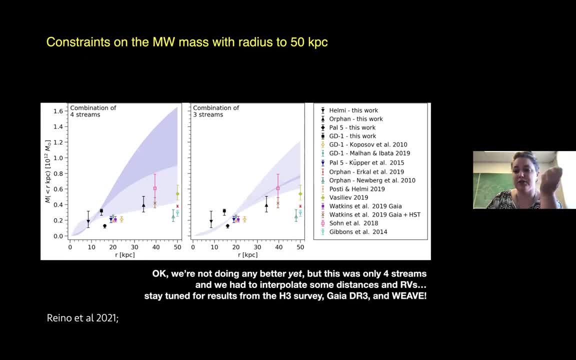 Um, but this was only four streams and we didn't have complete phase-based information for everything. Some of the quantities, like distances and radial velocities, were interpolated along the stream track from the numbers. Uh, what we're doing now is examining some of the biases in 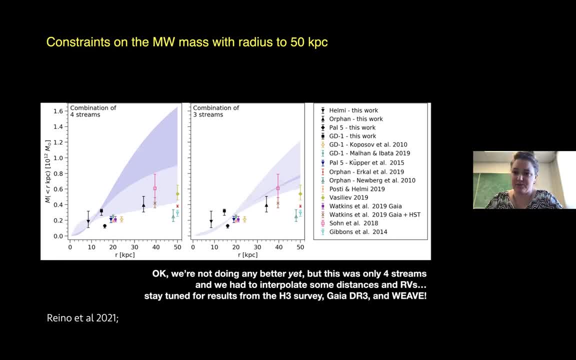 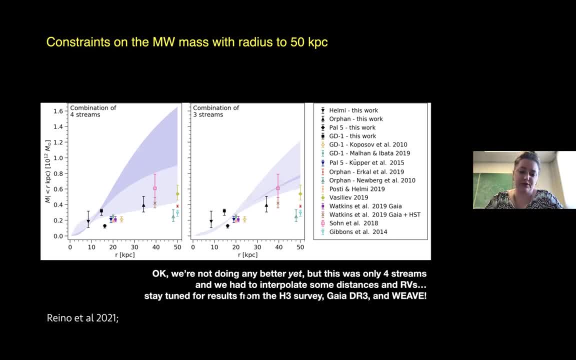 Um, and preparing to fit the data that the H3 survey run by Charlie Conroy and Dennis Ritzke and Ana Bonazza, um have got in the outer halo, Um, and there we don't necessarily know the membership of every star, uh, but we have a lot more streams in the set and should get a good 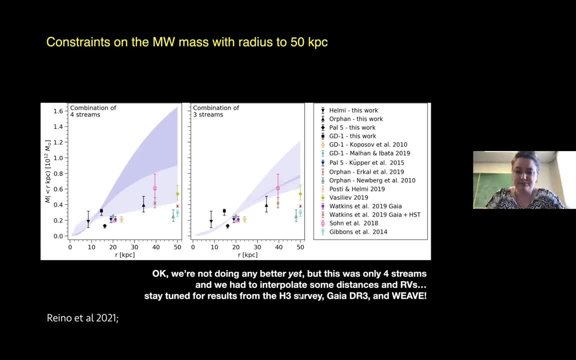 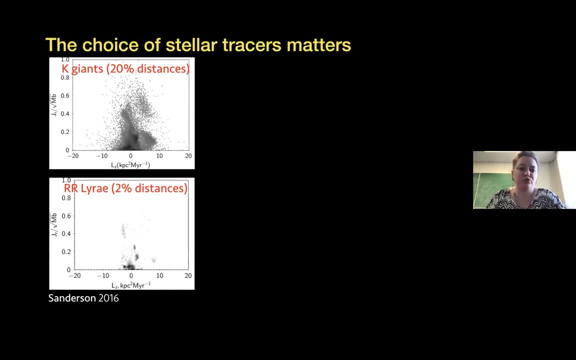 constraint out to much larger distances. Another point that I wanna come back to here is that, again, the choice of tracers matters not only for how far you can see them, but for how well you can measure their, their phase-based information. So if you 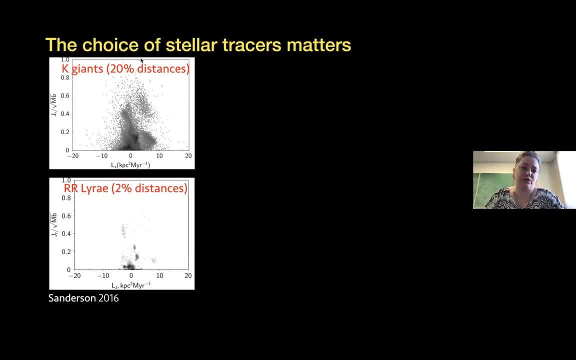 look at the actions based you get from giant stars where you can estimate the distance to 20%. you get a lot of blurring because the distance comes in everywhere when you're computing the actions. So it's, it's an interesting matrix, Um, so, um, I think that's. uh, you can see that. 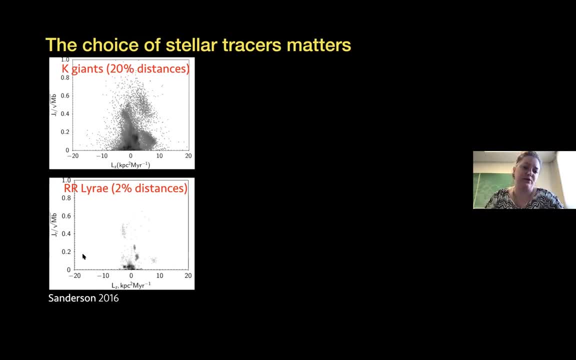 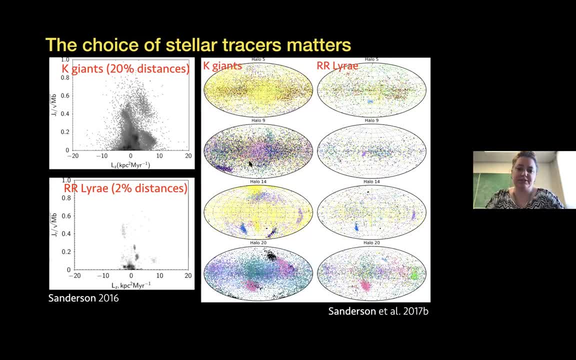 And you also sometimes see different streams. So on this side you see different colors for different streams in these different sample halos And the colors match over here for the same streams as seen in our library. And if you compare, sometimes you see a color in one panel but not in the other. that means that stream has a lot of one type of stellar population but not another. 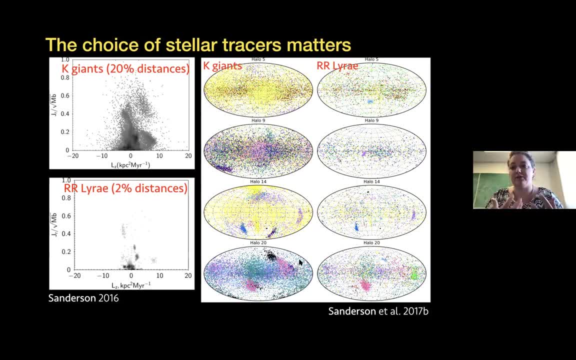 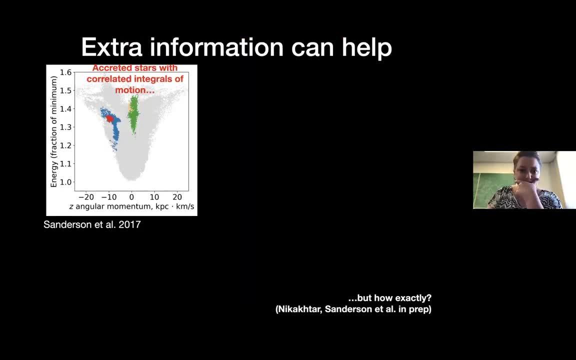 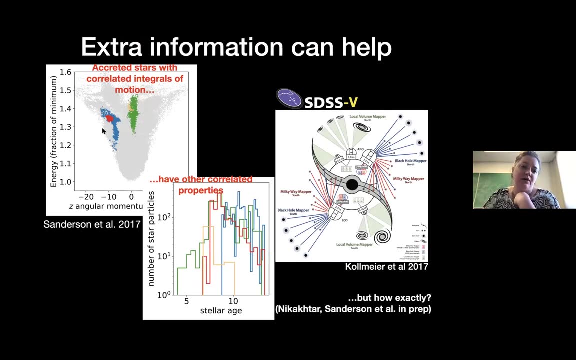 And so, to get the most complete view, you actually need to combine all these tracers, which means you need fairly sophisticated stellar population modeling in order to understand how to do this, And the extra information in ages or metallicities also helps you in this technique, because it's like fuzzy membership information. 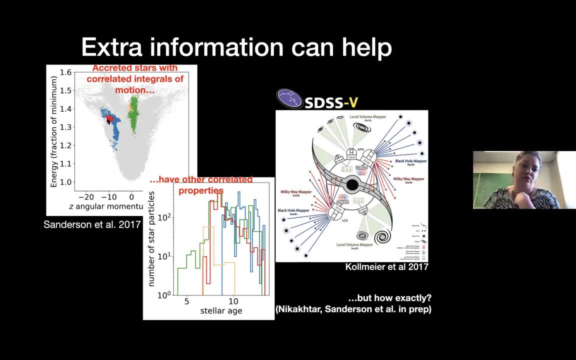 So the stars that are created from the same thing have correlated integrals of motion, but also correlated ages, correlated metallicities. They're not the same, They're not identically correlated, but they're close enough that you can disentangle things in extra dimensions and improve your estimates that way. 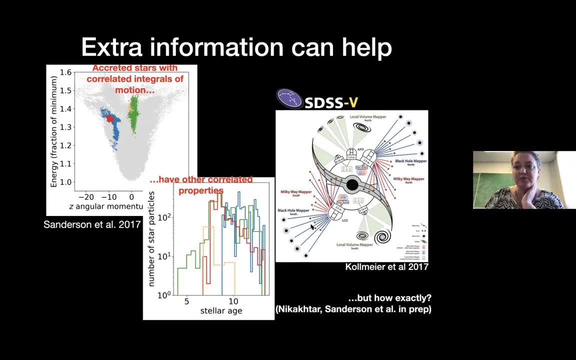 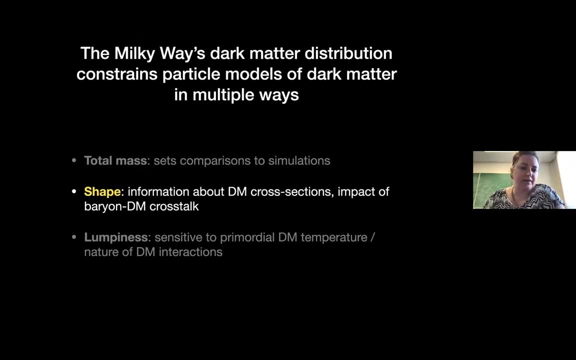 And that's where things like SDSS5 will really shine, because they give such a large dimensionality of extra information. So we're hopeful that, given the increased range of this high dimensional information about Milky Way stars in the stellar halo, we'll be able to 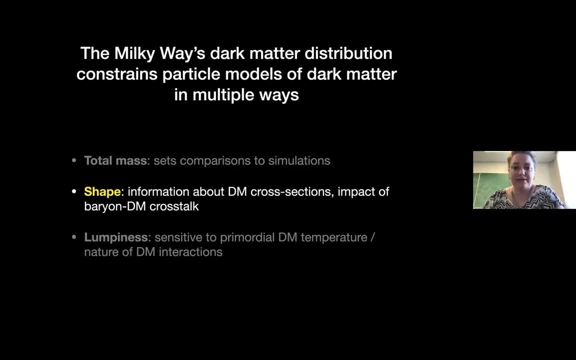 get a better handle in not too long on the total mass, And then we can start talking about the shape of the halo, Both the slope of its mass profile as a function of radius, and also whether it's axisymmetric, triaxial, how that changes with distance, and so forth. 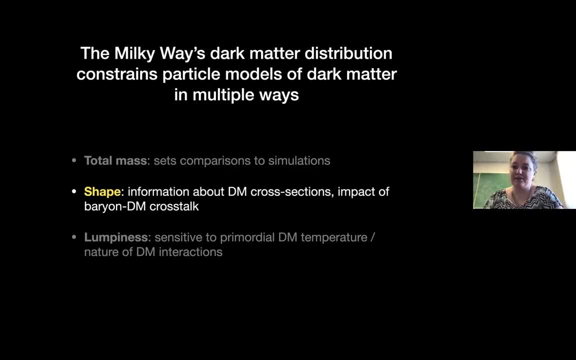 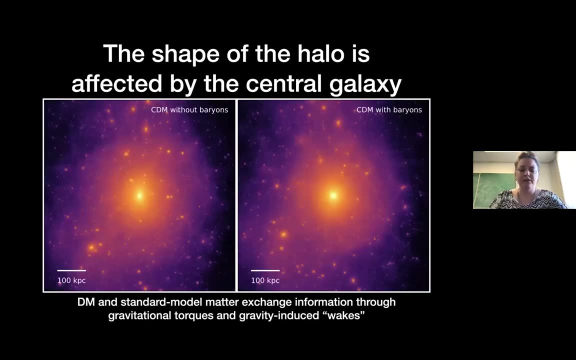 And in here there's a lot of information about the impact of the crosstalk between the baryonic component of the galaxy and its dark matter. But there's also information about the late time interaction cross section of dark matter. So this is something I've been digging into recently. 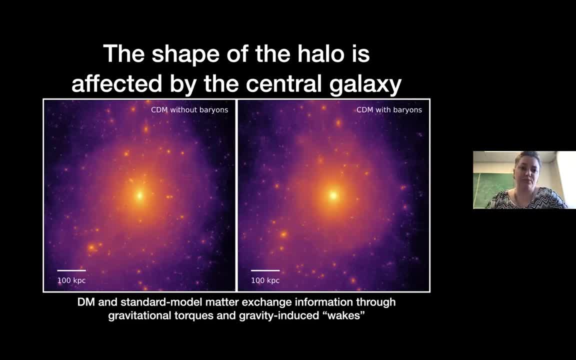 So the first thing to know is that the shape of the dark matter halo is significantly affected in the inner part by the formation of the central galaxy, Because the tides, wakes and torques of the dark matter on the forming disk of the galaxy, and vice versa. 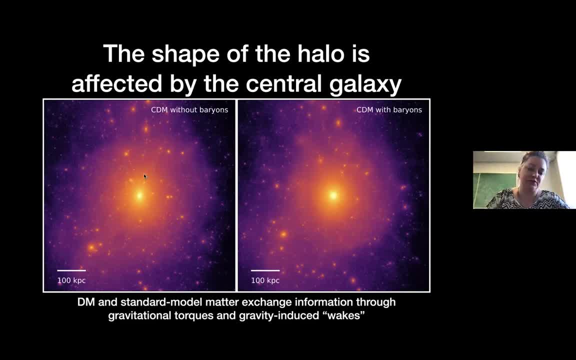 tend to average out the triaxiality that you see when you don't form a galaxy in the center of your dark matter halo, So you get something that's a lot closer to spherical in here But at the outskirts still sort of remembers the directions from which things are creating through the filaments connecting our galaxy to the cosmic web. 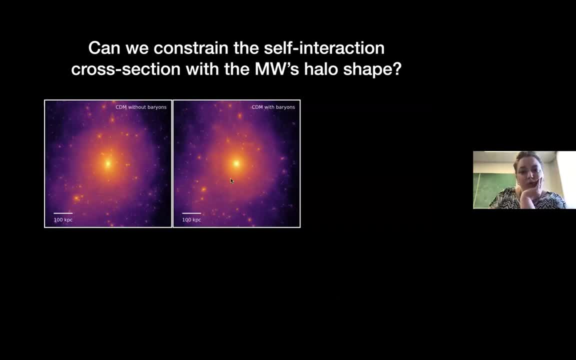 So what we were wondering, though, is that those processes, all sort of in this example, presumed that the dark matter is completely collisionless. That makes it difficult to lose angular momentum, exchange energy, and so forth, So it limits the ability of the dark matter halo to respond to the galaxy forming in the center. 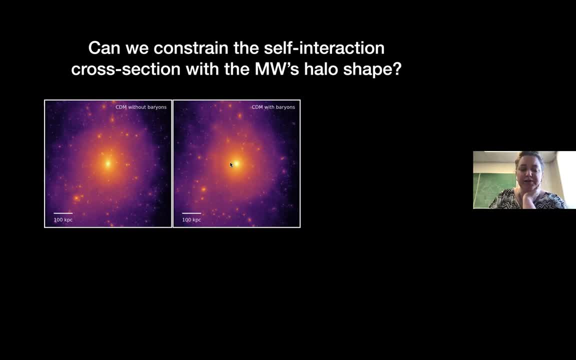 And we were wondering so what happens if the dark matter has a significant self-interaction cross section? This has been posited for a number of as a solution to a number of observations, A number of observational discrepancies recently. Does this affect the halo shape? 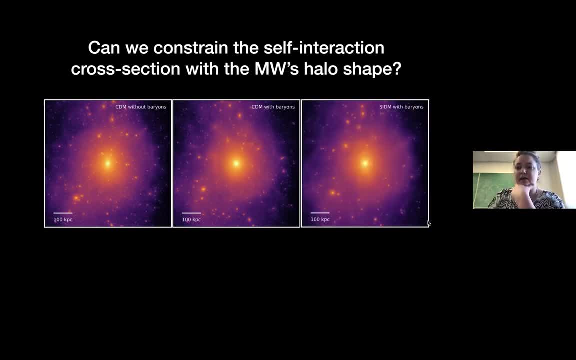 So if you use a model in which the dark matter does have some self-interactions in the late universe and you simulate a galaxy forming, you do see some differences in the from the cold dark matter case. They're subtle, But this, to me, pointed out something worth following up. 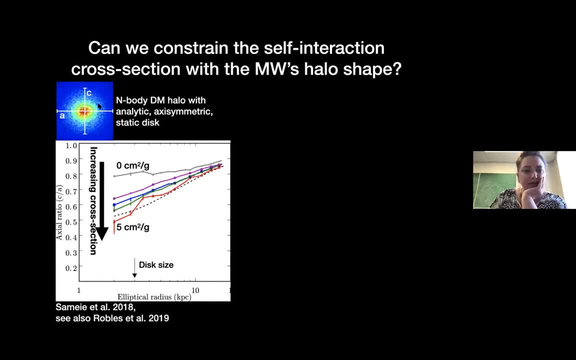 So we have a suite of these things now. There had been reason to think that, because a non-zero interaction cross section lets the dark matter respond more efficiently to the formation of the galaxy, you would expect, in particular, that the inner part of the dark matter distribution would be flatter as the cross section increases. 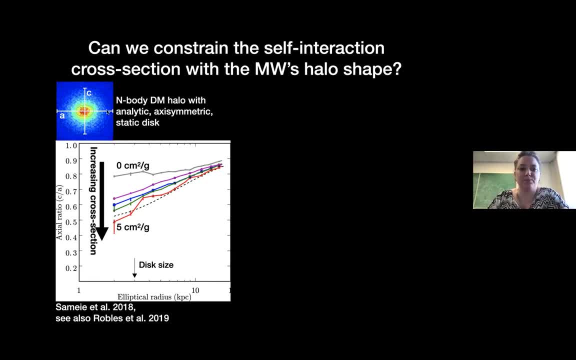 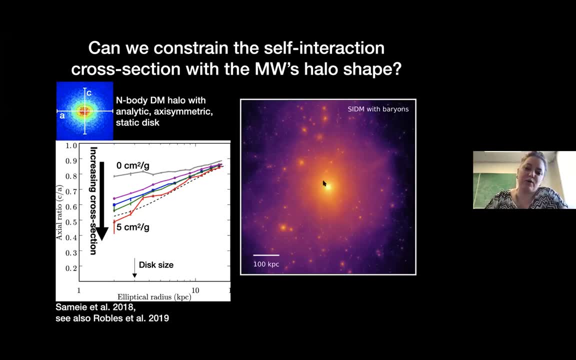 Because it will start to take on the shape of the disc distribution in the galaxy, And so we can check out whether this is actually the case by studying the shapes of the suite of simulations where we've run the same exact physics except for the interaction cross section of the dark matter particles. 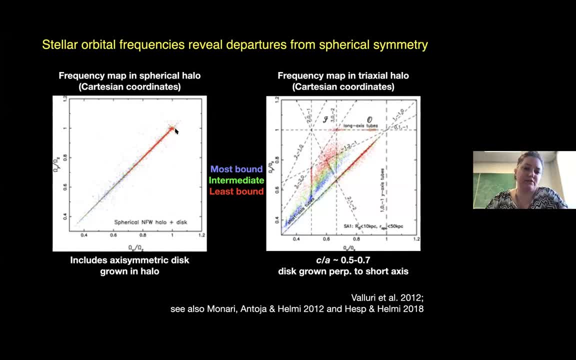 This maps back to dynamics in a couple of ways. The most interesting to me at the moment is that the orbital frequency ratios of stars in the galaxy can reveal departures from spherical symmetry. So as an example from a paper from nearly 10 years ago now, 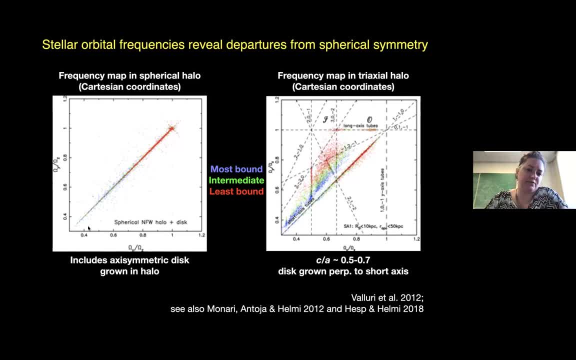 in a spherical halo you'll infer a lot of You won't have very much dimensionality in the frequencies of the stars. But in a spherical halo you'll infer a lot of You won't have very much dimensionality in the frequencies of the stars. 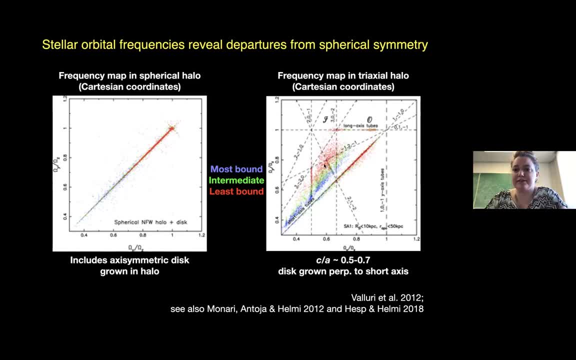 But if you make the same map in a triaxial halo, you'll see a lot of different resonances and structures in the map of the estimated frequencies for the different stellar orbits, And this is with a relatively reasonable degree of flattening. And so what I'm hoping eventually is to update some of this stuff using better models that are keyed to our 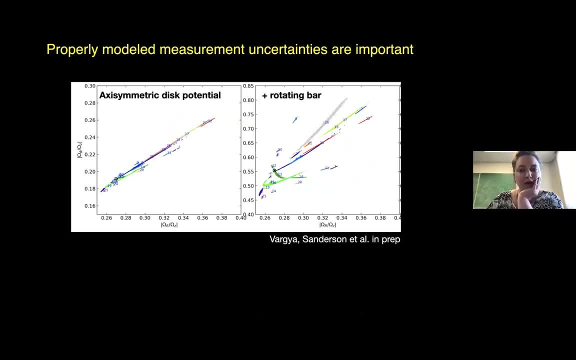 new simulated systems in the different dark matter models. It's also worth noting that modeling the uncertainties on your measurements are important, since the measurements that go in here are the phase-based components of the stars' positions and velocities, which all have uncertainties. And if you take a bunch of stars, for which we make these measurements with Gaia, and propagate those into this frame, 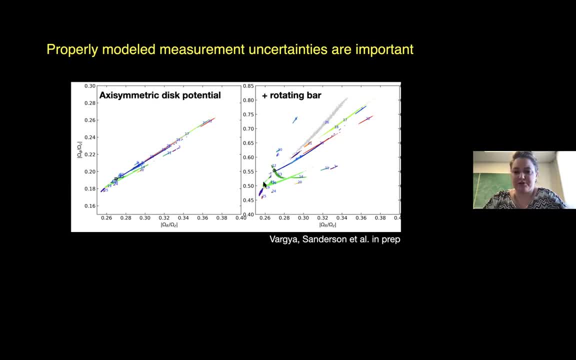 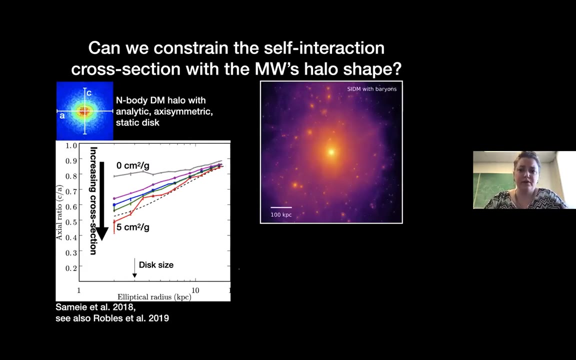 you can see that the resulting error bars are extremely non-trivial to deal with unless you Monte Carlo everything, And they can to some extent contribute to our ability to distinguish between potentials. So this is an interesting idea, but in reality we don't have an analytic growing disk in the center of the dark matter: halo. 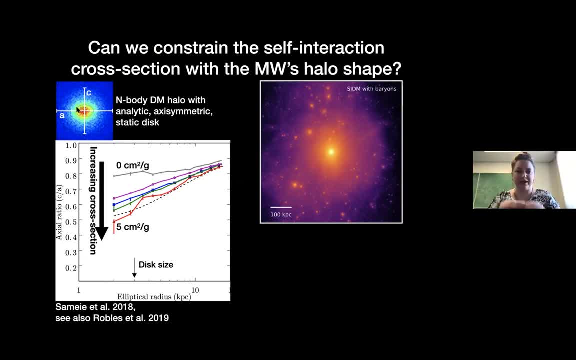 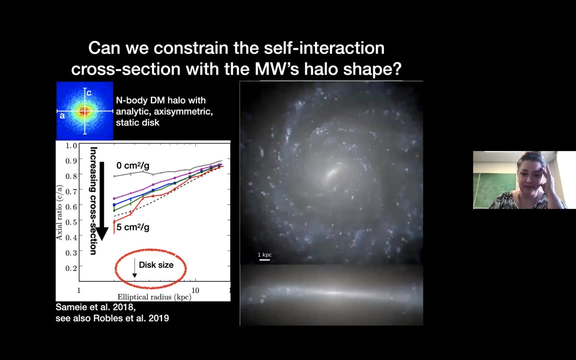 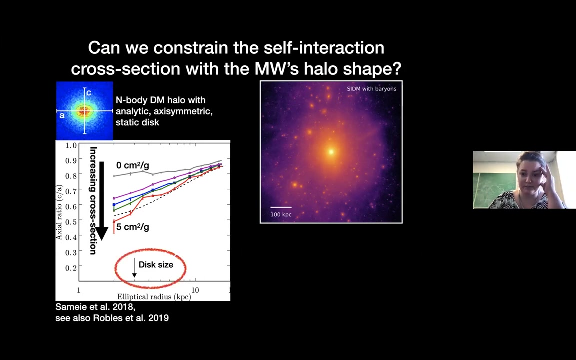 that stays in the same orientation all the time and has a well-shaped form. What we really have is a chaotically assembling galaxy. The region where we want to look for this is within the region where the disk is assembling, And this is what the disk looks like in the center of this dark matter, halo. 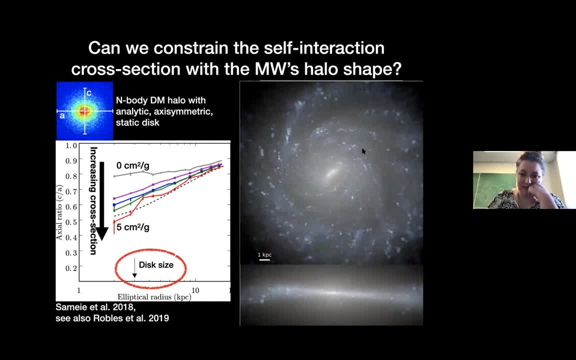 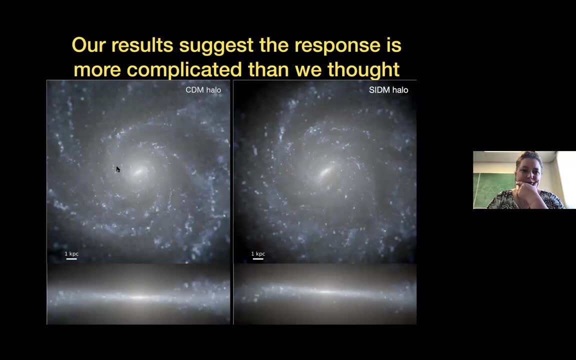 So it's not axi-symmetric, It's definitely not static. Look at that bar there And there's lots of spiral arms and all kinds of action. You can see a little bit of a loop here. So if you compare this to the same initial conditions run with the same baryonic physics- 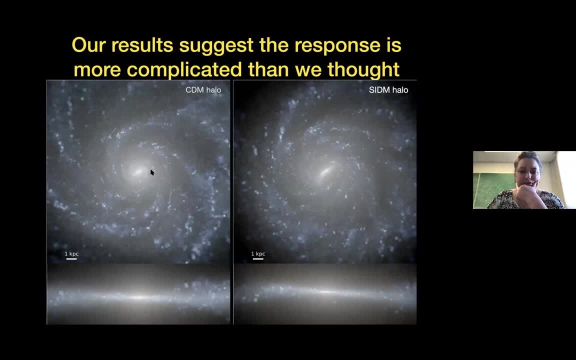 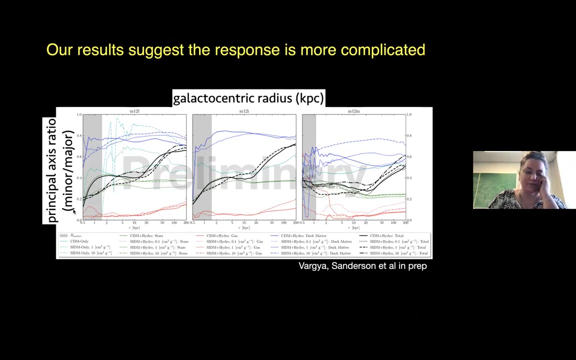 but in a cold dark matter halo with collisionless dark matter, you can see that there are also some differences here, but it's subtle and more complicated than we thought. So if you go through, if you map the shape of the galaxy, and by that I mean its principal minor to major axis ratio, 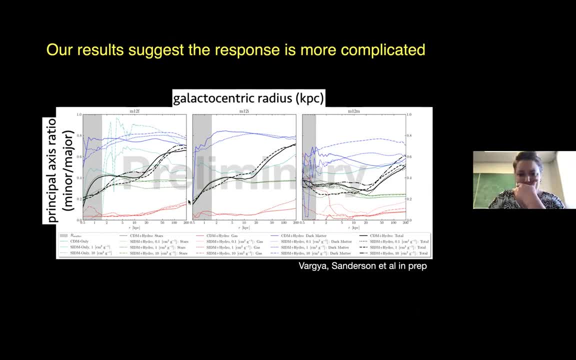 of the different components as a function of radius. what you find is that all the runs, no matter which simulated galaxy we're talking about or which kind of dark matter we're trying to simulate. you can create a galaxy with a thin, gaseous disk, that's these red things. 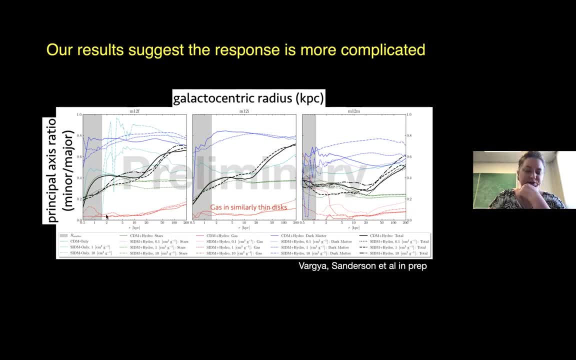 Down here. These are the shape profiles, And so the fact that this ratio is low means that the gas distribution is very flat. A ratio of one means the spherical system, And then there's a lot of variety in what happens in the inner part of the stellar distribution. 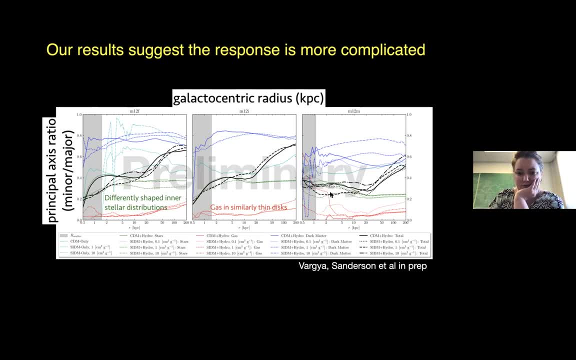 between the different runs with the same initial conditions in different dark matter physics. So each of these panels is a different suite of identical initial conditions And you can see. you can see that in most cases what you find is that the actually the CDM only galaxy is slightly rounder. 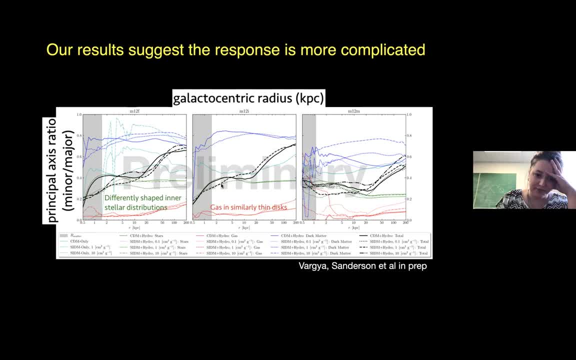 or the CDM version of the galaxy is slightly rounder in the middle than the ones with SIDM, And this suggests that there's indeed some feedback. And when you look at the dark matter which is subject to those effects in that region, 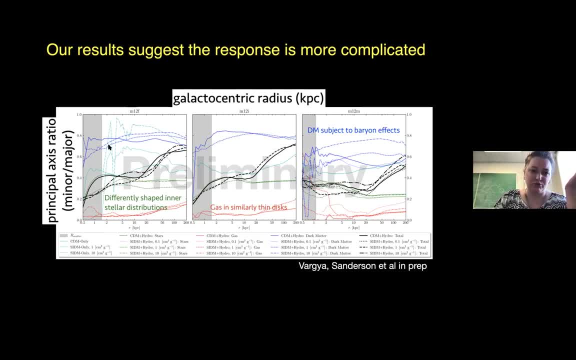 you see that it also pulls the dark matter distribution to be a little flatter, like you might expect. But there's a lot more stochastic variation, especially you can see in this case. There's more to the story than that, clearly, because the variation is not as clean as in the semi-analytic models. that had been done previously. 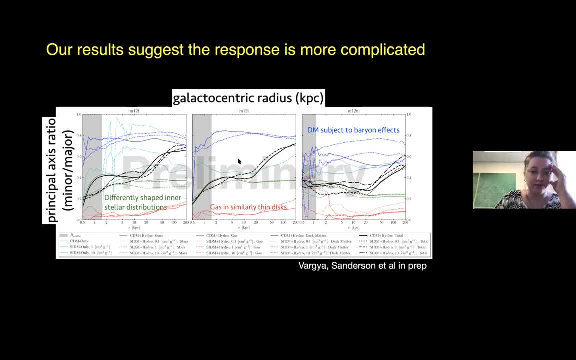 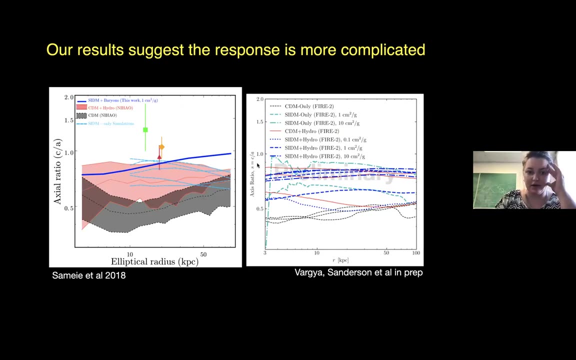 So it's clear that the introduction of an interaction cross section is changing the way that the dark matter responds to the baryons, and vice versa, But clearly this is a two way process, And so we're working on ways to figure this out. 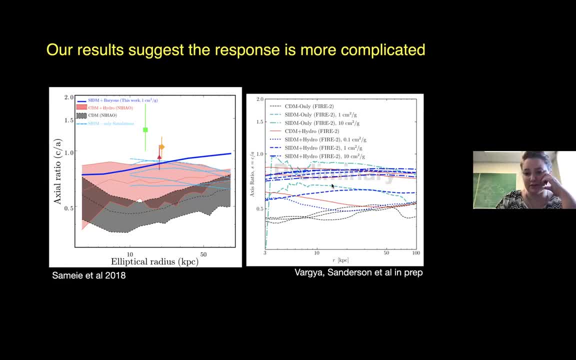 In the meantime, I'll give you the takeaway that just measuring the axis ratios doesn't go far enough to differentiate between these models. it looks like You can see here: these blue lines here on the on the right hand panel are the different runs that we did with different cross sections of dark matter. 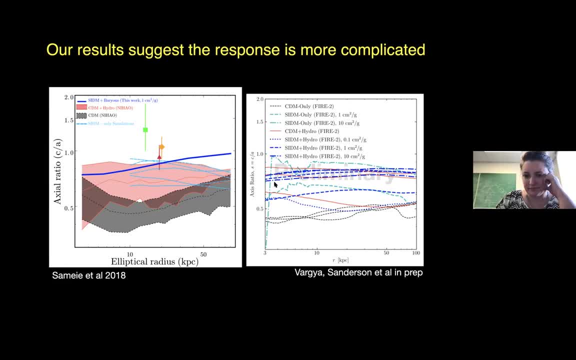 And the variation between them is comparable to these red lines which are the different galaxies simulated with CDM. So the variation from galaxy to galaxy, just by virtue of its formation, history gives a similar scatter and axis ratios and the shape of the dark matter, halo. 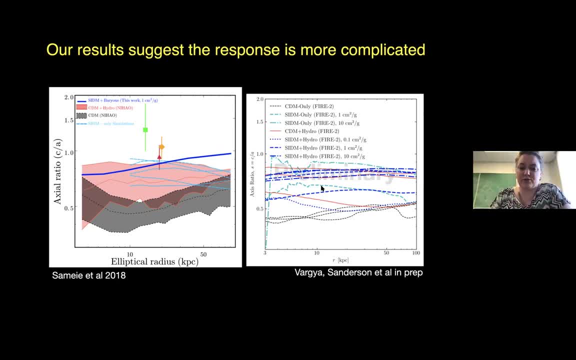 to the variation induced by fiddling with the dark matter cross section. So just measuring the cross section, or, sorry, the shape alone, is not enough to do it, which is probably good, because here's all the different attempts that I could find at measuring the shape of the Milky Way's halo. 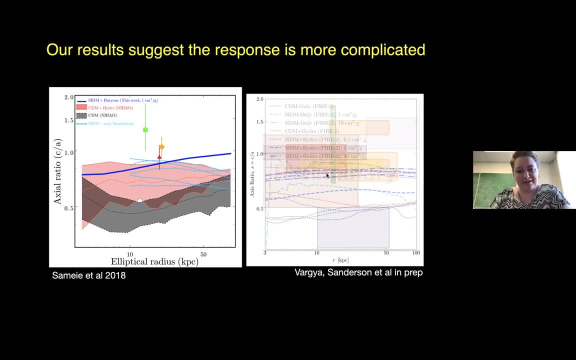 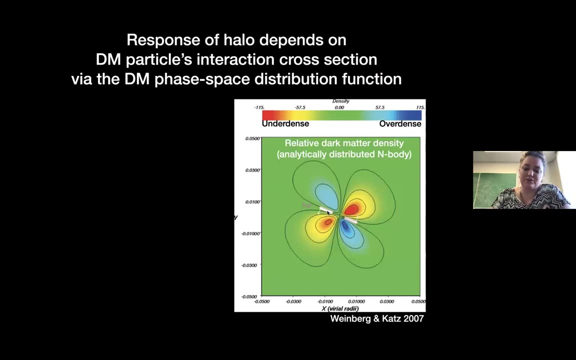 and the radii that you see here, And we're not very good at this yet, So it'll be useful to know where to direct our efforts in future. One place that we're looking now is at what happens in terms of the response to a bar evolving in the center of. 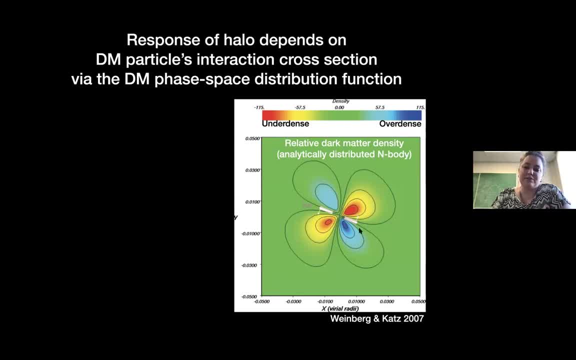 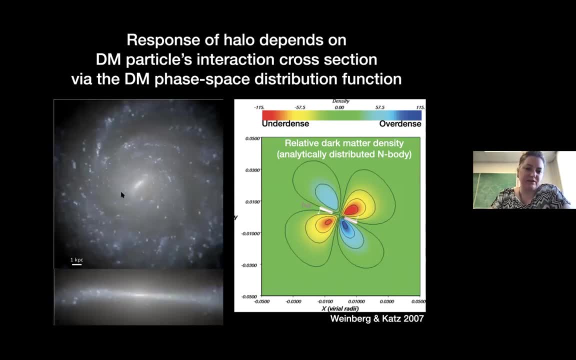 of a galaxy like this in different dark matter models. So even in CDM, a bar will stir up the dark matter just by virtue of dynamical friction, And we found that several of the simulated galaxies with different models of dark matter form a bar. 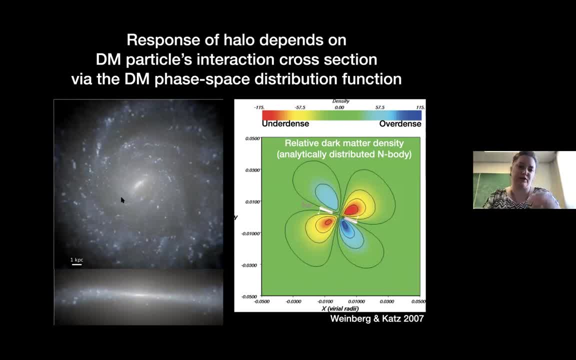 And so we can look at how this responds, And I'm a student who's working on an analytic model based on this paper by Weinberg to try to predict what happens to the evolution of the bar's pattern speed if you change the dark matter and therefore the phase-based distribution of the dark matter and 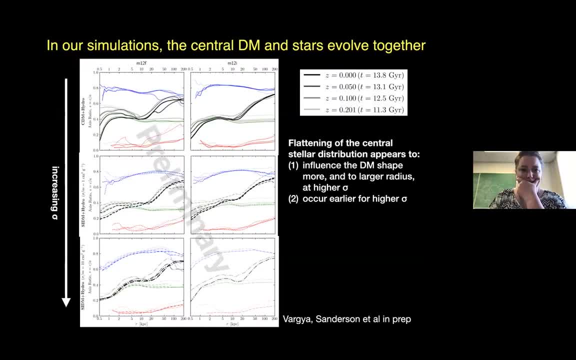 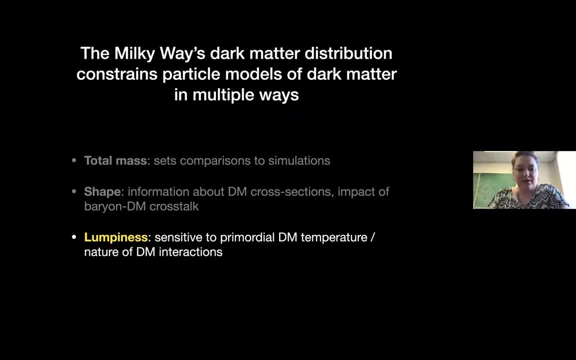 and therefore the dynamical friction that it exerts on the bar. I'll skip that for now, because I want to get to lumpiness, So I'm probably running out of time, Okay. So the last thing I'll talk about here is the way in which 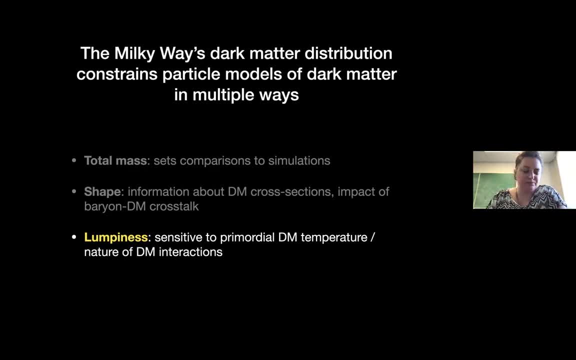 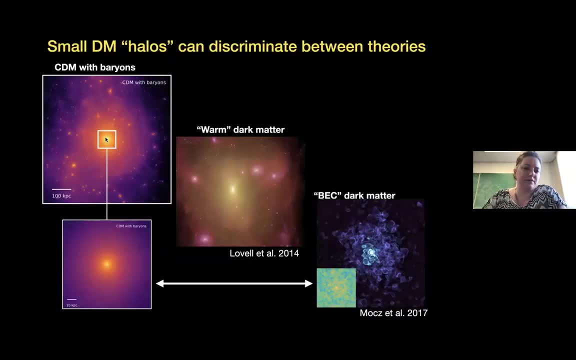 the Milky Way can be used to probe the primordial dark matter temperature, And that's through the degree of substructure. So the substructure in the dark matter of our galaxy has long been demonstrated to discriminate between different theories of dark matter. So in a cold dark matter system, 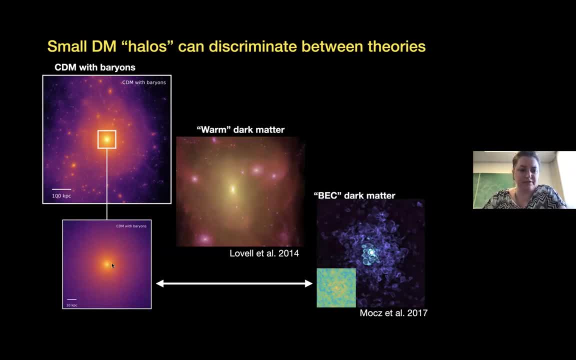 you have lots of structures, although the disk is efficient at depleting them in the inner part of the galaxy, In warm dark matter. like I mentioned at the beginning, you cut off the power spectrum of initial density perturbations at some point and damp out all the small scale structure below some cutoff. 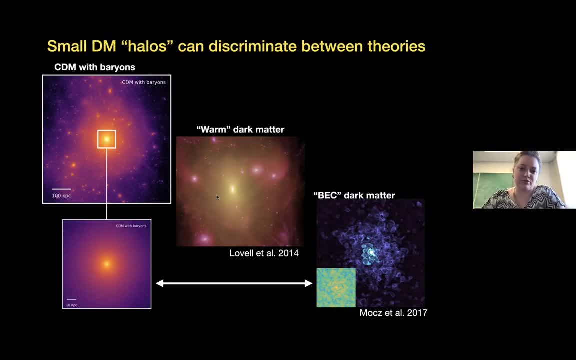 As you can see here, this halo looks a lot smoother, with just large lumps And in some of the models that are now popular for BEC-like dark matter, stuff made of like an ultralight axion or whatever- some of the substructures come. 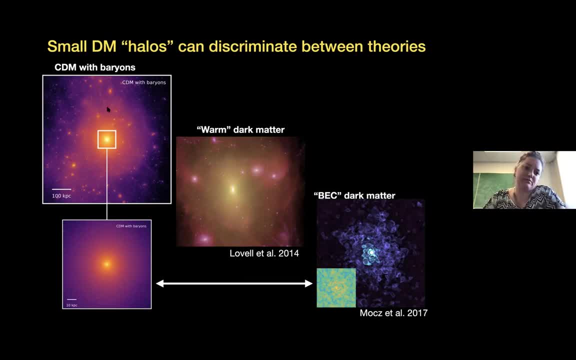 through the same channels as CDM, where you get, you know, lumps of things that behave like particles, but you also get sort of interference patterns that look completely different in terms of their distribution, And so being able to discriminate between these would be really useful, and tidal streams can really help us here. 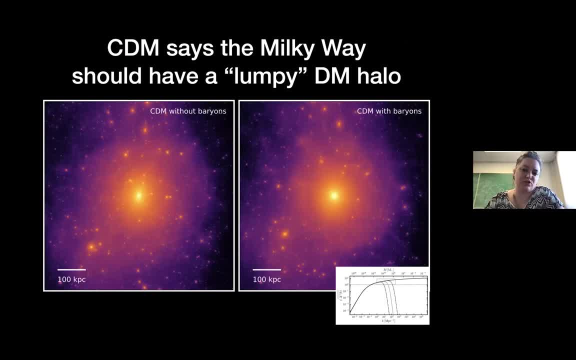 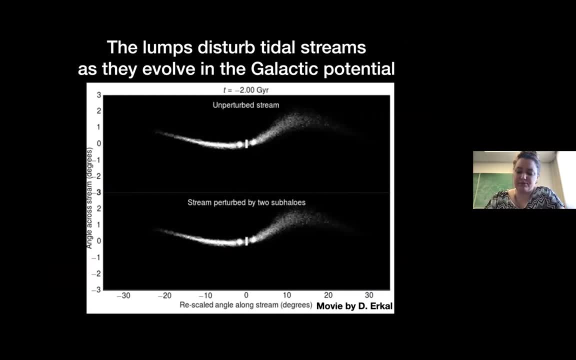 So, like I said, CDM says we should have a relatively lumpy halo compared to a lot of other, a lot of other dark matter models, and these lumps will disturb the careful ordering of stars by energy that happens during tidal disruption. So this movie from Dennis Urquhall is a good illustration of this. 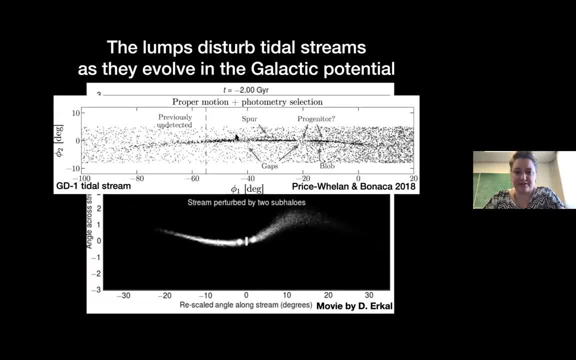 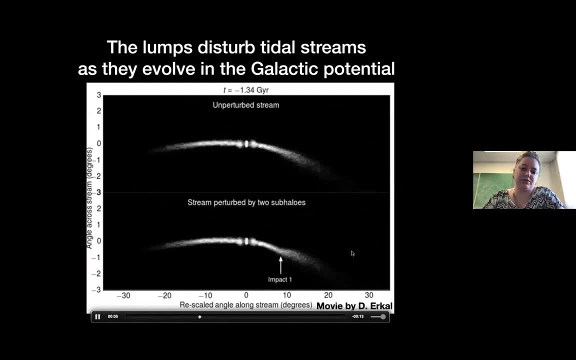 This is actually a model of a stream from a globular cluster, not a satellite galaxy. it's pretty thin, Sorry. And then in the bottom panel you'll see what happens when it passes by two relatively large substructures. so it sort of reorders the particles in terms of energy. 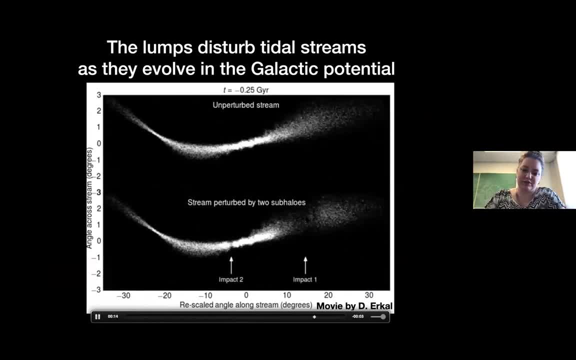 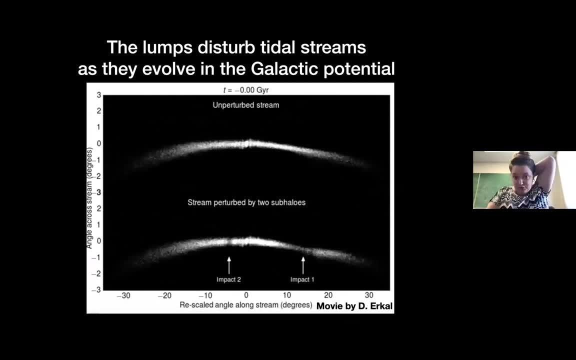 And since this is a pretty significant interaction, eventually a little gap opens up in the stream, and here's another one, And so these lumps should perturb the stream. This obviously is this, but in ways that we might be able to detect, since these stars all came from a relatively small part of phase-based volume to begin with. 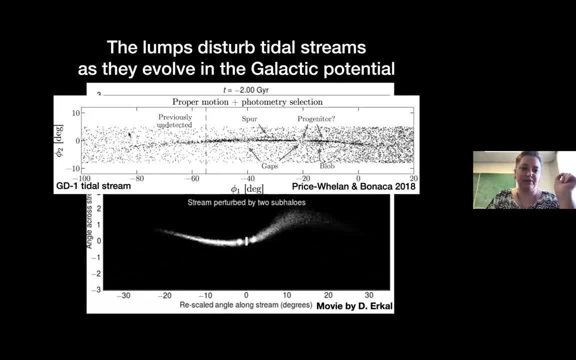 So there's some really tempting evidence now that we might be seeing things like this, For example in this view of the GD1 stream. But there's a relatively long way to go between the observation of individual gaps or perturbations And so we have a real tidal streams in our galaxy and an interpretation of this in the context of a particular dark matter model, and the intervening step in doing that is to simulate the cosmological predictions for the dark matter halo along. 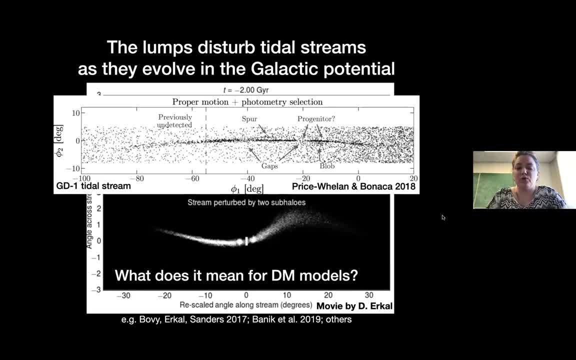 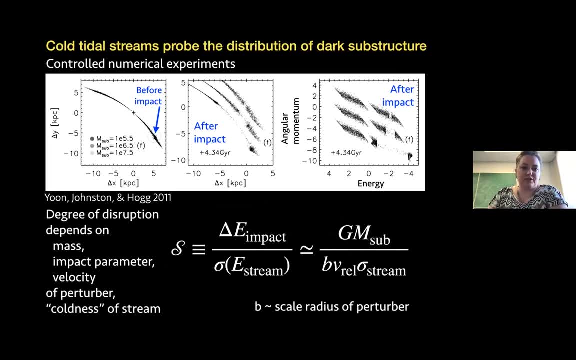 with the hierarchical assembly that cosmology predicts will form the tidal streams that you're talking about. So just a little bit of an introduction to this: The um, the um. if you have one of these impacts, uh, the effect after the same amount of time, which is 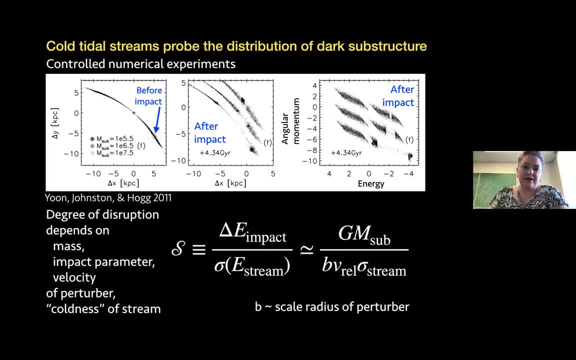 ambiguous in most cases. for real streams scales with the mass of the little substructure that passed by um and it's inversely proportional to the size or fluffiness of the perturber, because that sort of sets how close the or how small the impact parameter can be. 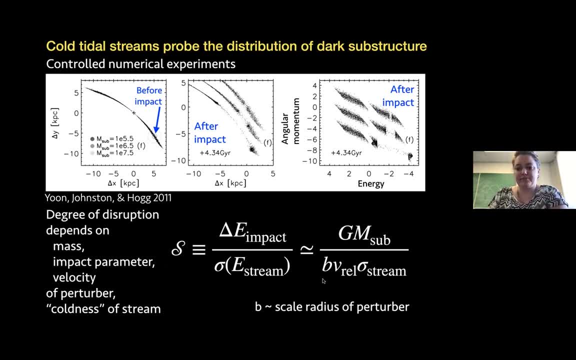 for one of these. if you have a big subhalo, um the, the scale radius is larger, and that's really the sweet spot for disturbing the stars. um, and the strength of one of these interactions is also inversely proportional to the relative velocity. so if something is on a slow relative speed, you'll 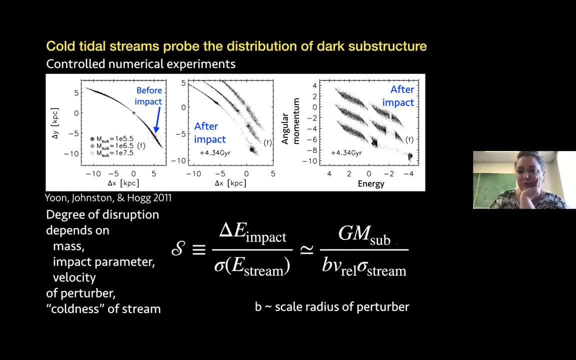 have a larger chance to destroy the impact parameter. and so that's really the sweet spot: the stars in the stream and reorder them um and inversely proportional to the intrinsic velocity dispersion. so a cold stream will show more of an impact. uh, because there's less random ordering. 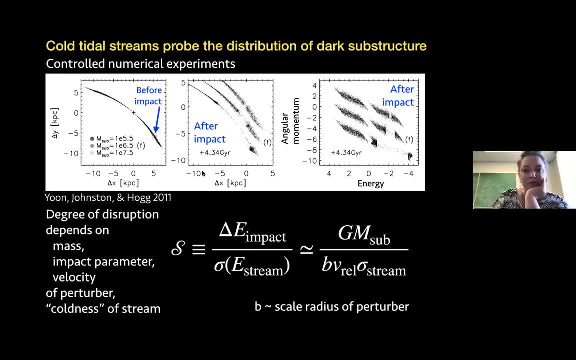 within the stream that would, over time, erase this um. so there's actually a lot of things going on here, a lot of different handles that we can have on both the population of substructures and the types of um and the population of tidal streams making up our halo um. unfortunately, it's not always so clean. so 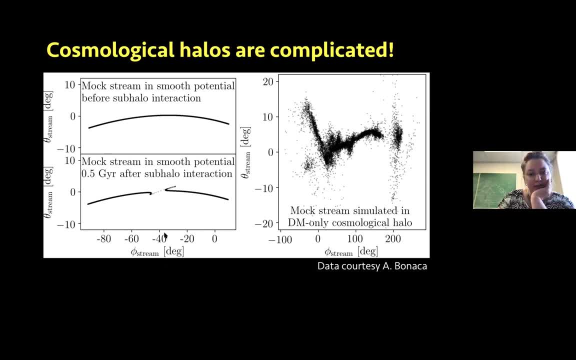 while this is sort of the sort of model that people like to fit, if you actually put one of these mock streams in a cosmological dark matter halo, you get something that looks more like this. some of this is because there are too many substructures. this was a dark matter only. 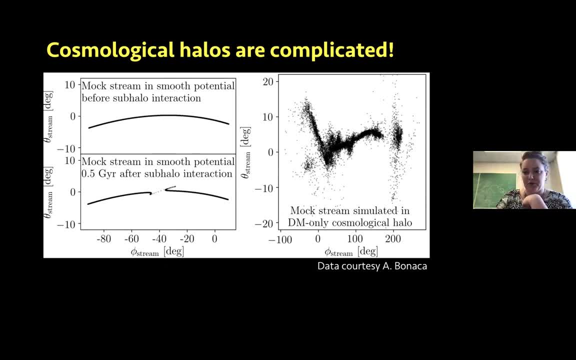 simulated halo. some of it might be numerical noise, um, from the differences in the in the masses of the halo, and some of it might be numerical noise from the differences in the particles. um, but still this is a lot more complicated system than individual substructures passing through, because the galaxy is a very busy place, um, and so another aspect that makes this 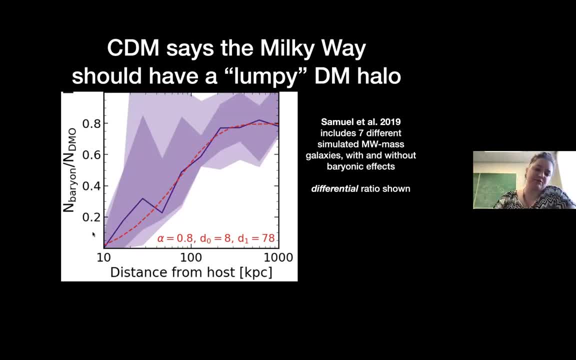 a challenging study is that the disk is very efficient at depleting um substructures in the inner part of the galaxy um. so this is the ratio between the number of substructures that you find when you add the galaxy into your cosmological simulation versus the number when you ignore it. 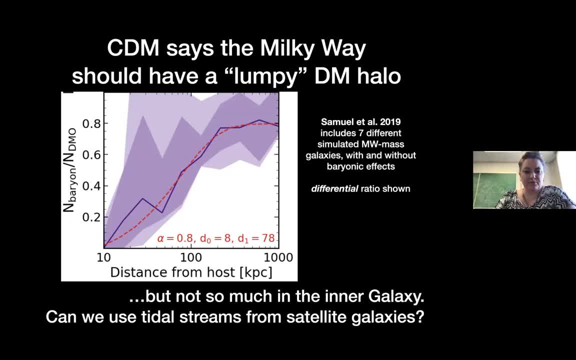 and just have dark matter For comparison. this is where the two most popular streams for doing these kinds of constraints are located. They're both streams that we think are from globular clusters. In the case of PAL-5, we see the cluster. 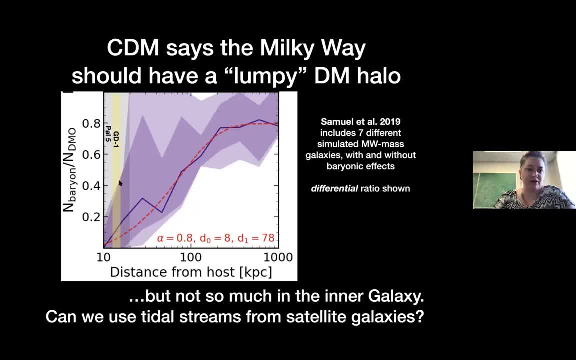 But they're in the region where the effect of baryonic physics is starting to be quite significant, And so really it'd be nice if we could work out here, But in order to do that, we need streams from satellite galaxies. Reassuringly, limits that people have tried to place. 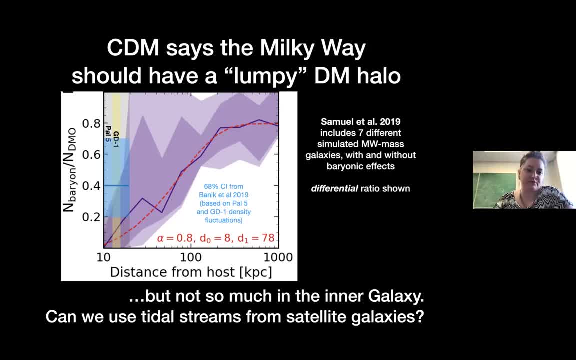 sort of look kind of like what you would expect if this was a plausible model. But again, because it's very hard to tell exactly how efficient the disk is at depleting substructures. there's a pretty big spread here between different galaxies, just by virtue. 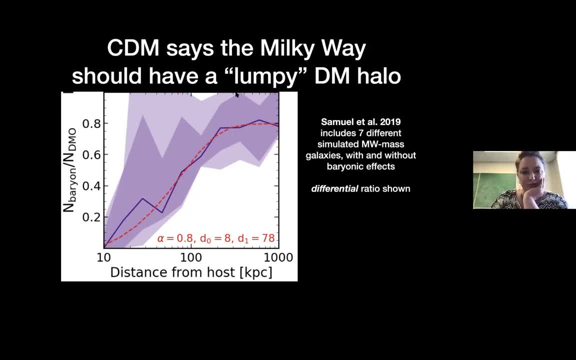 So if we were to look at the two of their assembly histories, it would be nice to get a little bit further away to where we think that that effect is minimized in order to really put some stronger constraints on the dark matter model. So what I've been doing is looking 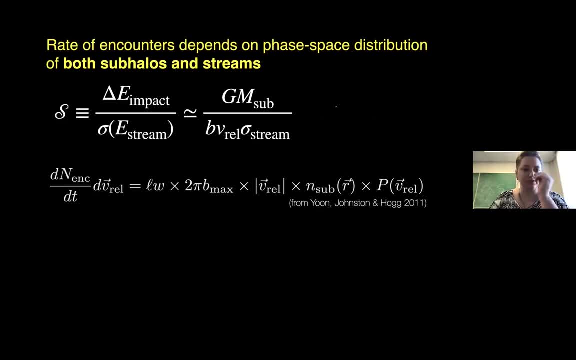 at whether you can use satellite galaxies and their tidal streams to do the same kinds of tests, possibly in a more statistical way. So what we're doing right now is just trying to figure out how many encounters a typical stream would experience, And that depends on both the number of subhalos. 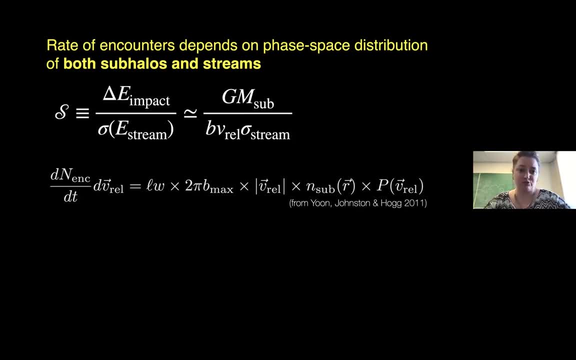 and their phase-based distribution, and the number of tidal streams and their phase-based distribution. So you have. so this big, long, horrible expression gives you sort of the number of encounters you expect as a function of time and relative velocity. It depends on the age of this tidal stream. 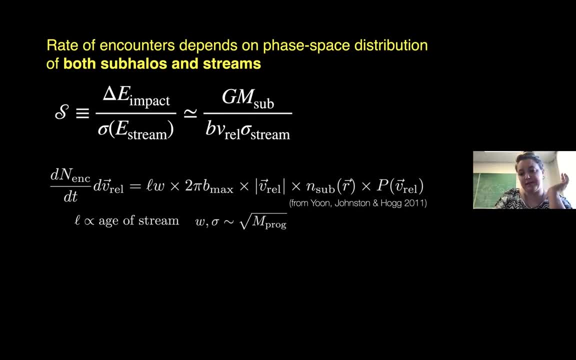 and the width which scales the square root roughly, of the mass of the progenitor. It depends on the scalar radius, which is a function of the subhalos, which is a function of their mass, and then on the relative velocity of these two distributions. 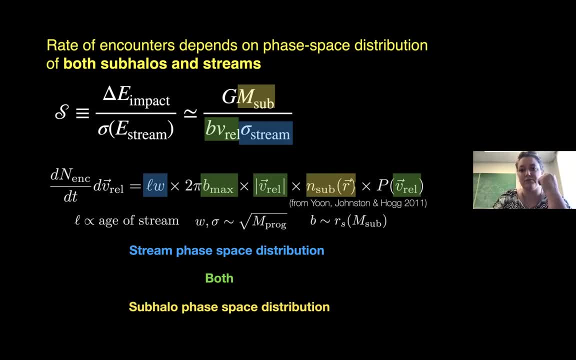 and on the number density of subhalos as a function of radius within the galaxy. So some of these things have to do with the phase-based distribution, Some have to do with the space-based distribution of the tidal streams, Some have to do with the space-based distribution of the subhalos. 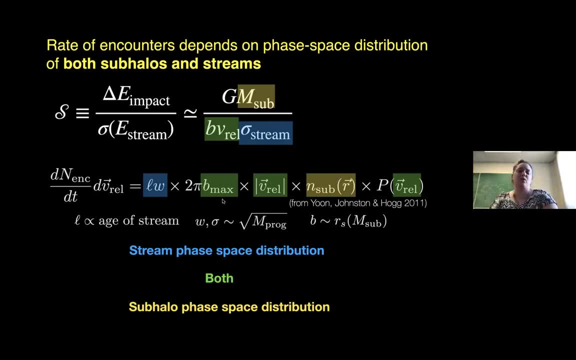 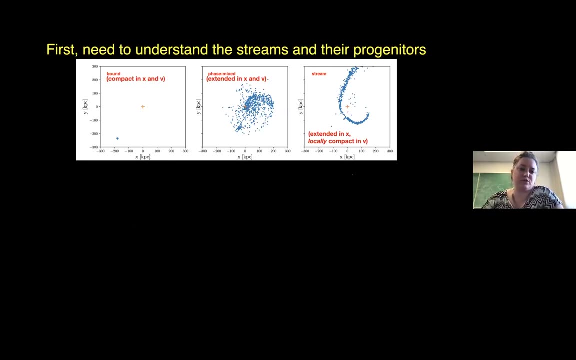 And some have to do with both together, And so quantifying this. people have made different assumptions about each of these properties in order to simplify this expression, And so what we're trying to do is to understand which of those assumptions are good and which are not. 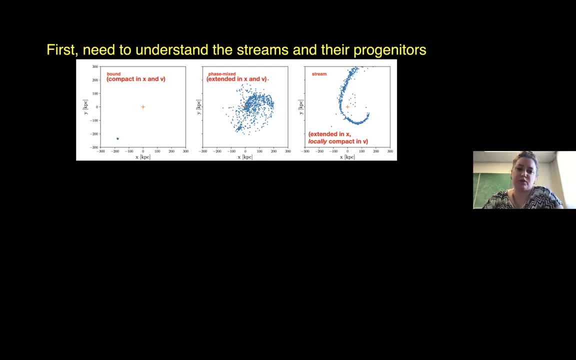 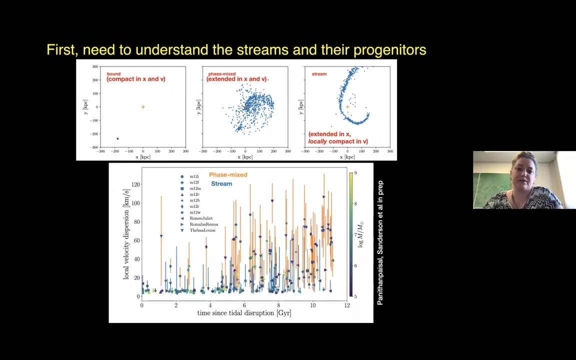 by using the tidal streams that we've isolated from the suite of cosmological Milky Way mass galaxies that we've simulated in the FIRE collaboration. So the first, zeroth order thing was just to be able to tell the difference between something that's bound, something that's phase-mixed and something that's a stream. 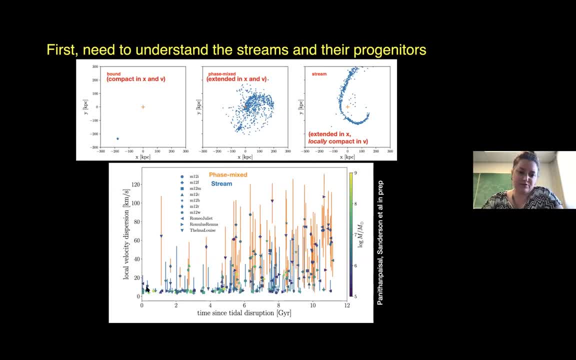 And if you look at the population of these things, you can see that all the blue error bars down here. those are all the things that are still coherent at the present day. The color indicates their mass in stellar mass, excuse me. And the y-axis here plots the local velocity dispersion. 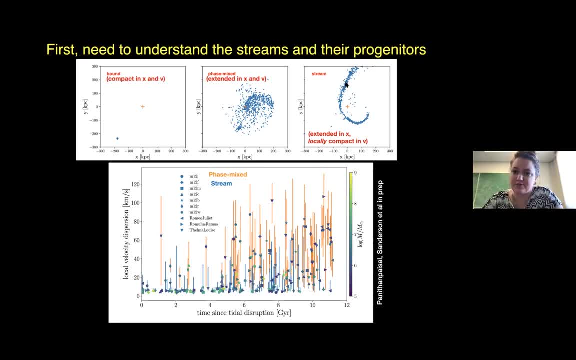 So what I talk about when I talk about sigma in the previous slide is just, if I pick some particles right around here in the stream, what's their velocity, dispersion? That's what's being measured here. So you can see that for the coherent streams, 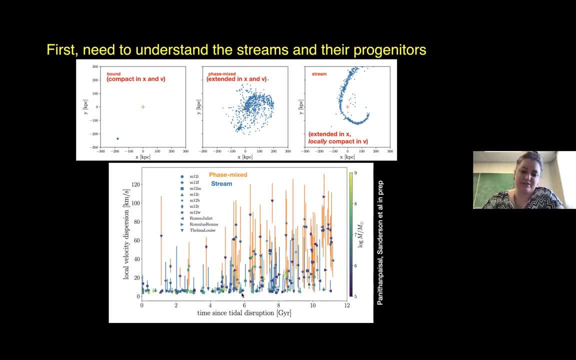 as you would hope, that local velocity dispersion is basically saturated down at the bottom of what we can measure with our resolution. But there's also a pretty abrupt transition between a period of time or a range of stream ages where you see mostly phase-mixed stuff. 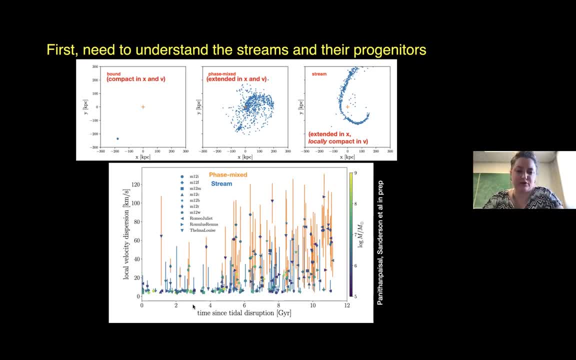 and where you see later on mostly coherent stuff. So younger streams tend to be coherent. older stuff tends to be phase-mixed, if that makes sense. But it turns out that this transition is not so much due to the mixing times but to the point where the galaxy forming. 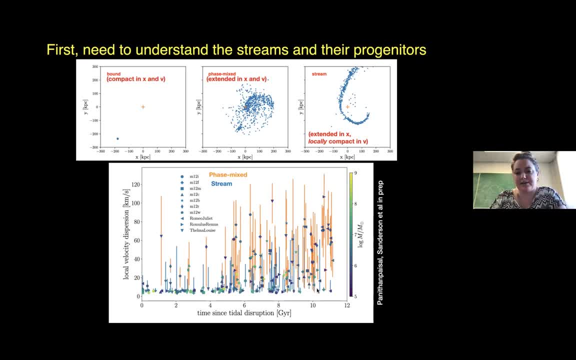 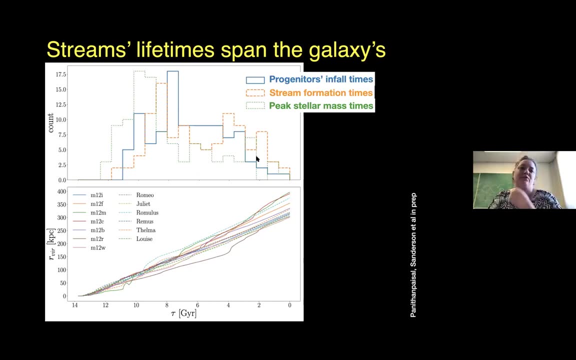 in the center makes a transition between a chaotic assembly phase at early times and a smoother growth of the disk in later times. The other thing to keep in mind here that is related is that the lifetimes of the coherent streams that you see in a galaxy today, basically 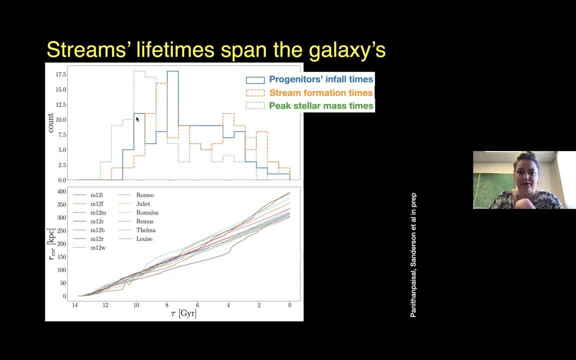 span the assembly history of the galaxy, And so if you look at the orange histogram here, that's the distribution of times since the different coherent streams were formed. This end over here is present day, and this end over here is the beginning of cosmic time. 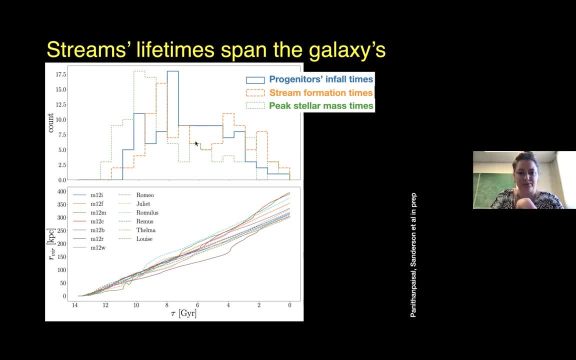 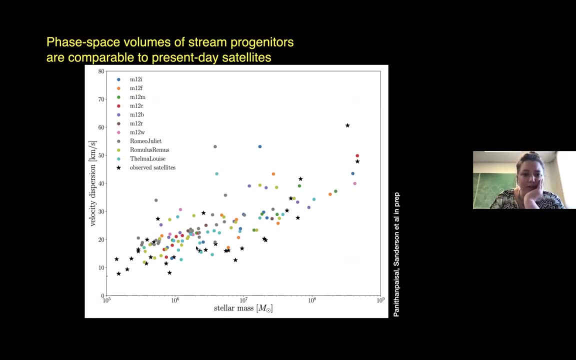 And you can see that the times that streams started to form that are still coherent at the present day range over nearly that entire period. I already talked about this. The other reassuring thing is that the progenitors that we find for the tidal streams in our simulations are representative. 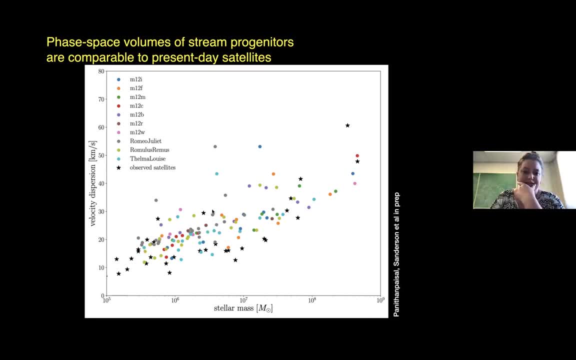 of the phase-based volumes that we see for present day satellites observed in the Milky Way. So this is a plot of velocity dispersion as a function of stellar mass. In the progenitors of the Milky Way these are called Milking waves. This is a plot of velocity dispersion as a function of stellar mass. 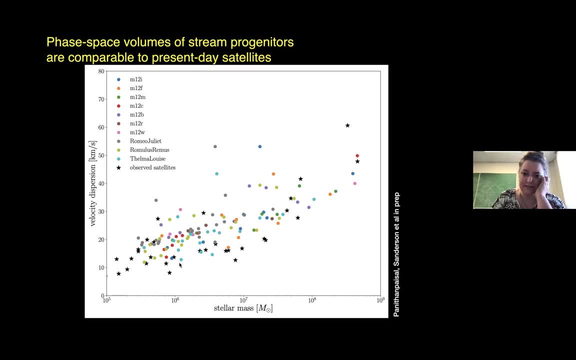 In the progenitors of the Milky Way. there is a probability of studying the weight of these massivestellar masses, which is 1.2 times the volume that the galaxy would see. that's right now the stellar streams, all the colored dots, And you can see that they match up with these stars. 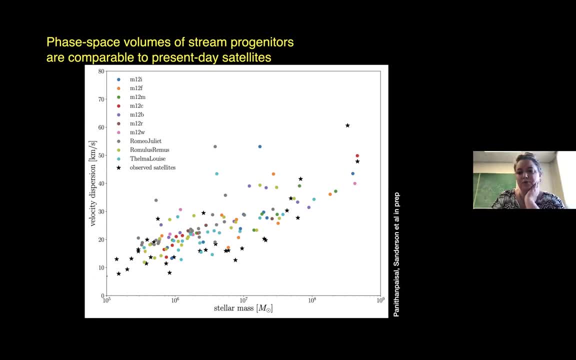 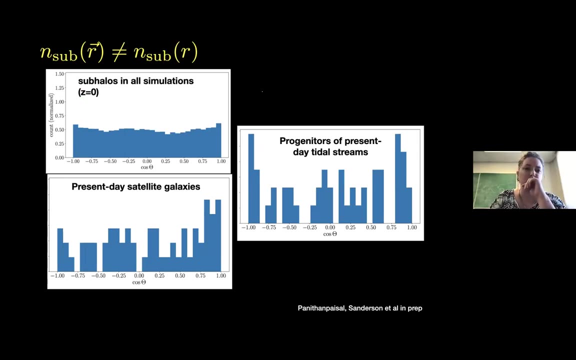 to the limit of our resolution down here. So we know that when we follow the evolution of these streams in the simulation, we are actually starting out with a size of in phase space that is comparable to what we would expect, which is an important So one of the basic assumptions that 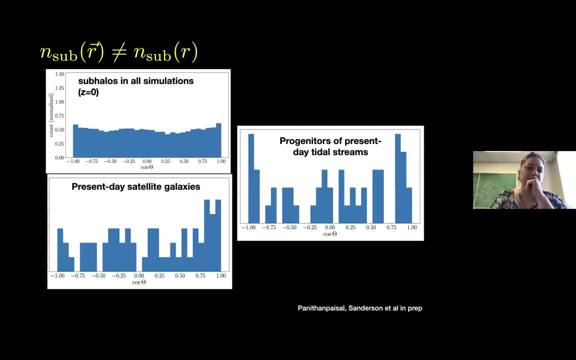 we tested first was whether the distribution of subhalos was isotropic. So most calculations that I've looked at of rates of encounters assume that this is the case, but in our simulations we find that it's not. So the distribution of subhalos relative to 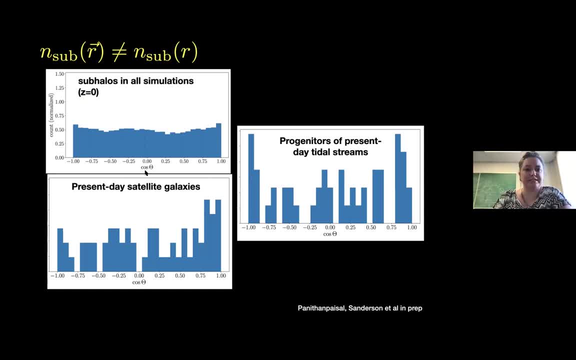 the plane of the disk at present day is pretty uniform, But present-day satellite galaxies and the progenitors of present-day tidal streams have orbits that prefer to be, in the case of the tidal stream, progenitors in the plane of the galaxy slightly relative to a polar orbit And present-day 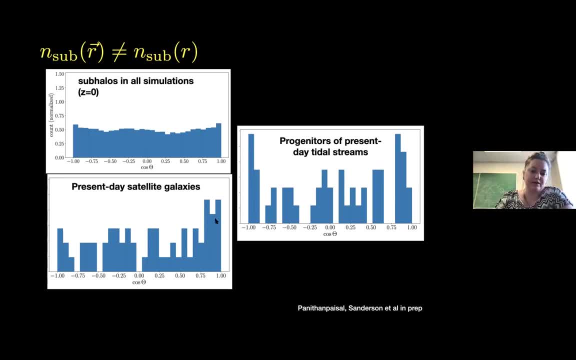 satellite galaxies tend to be depleted everywhere relative to prograde orbits, in the same sense as the disk, And so if you assume that this is not the case, or if you assume that the distribution of subhalos is isotropic, you're going to miss this preference And it's going to 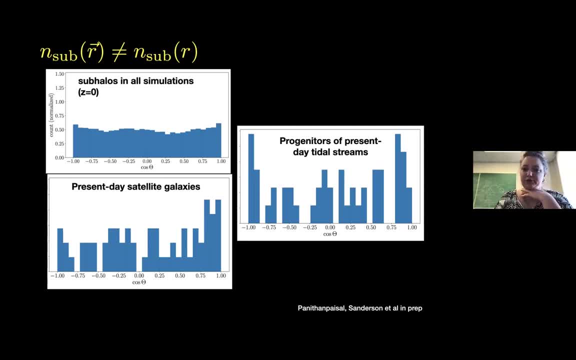 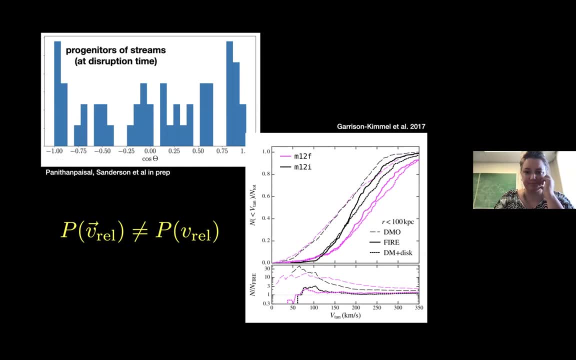 affect the rate at which you expect subhalos to be perturbing your streams. A related assumption that's often made is that the relative velocity distribution is isotropic, and we can see from the distribution of orbits of our progenitors that the distribution of subhalos is isotropic. 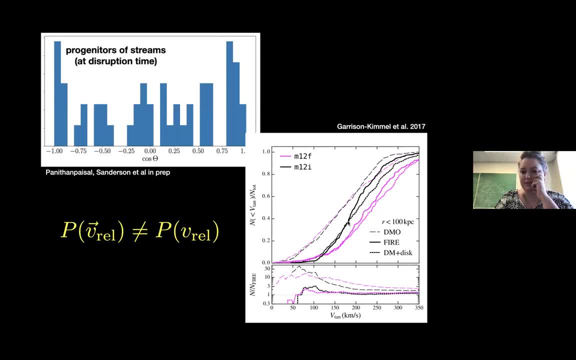 So in this case it just happens that the distribution of servitor orbits is actually the most effective because, basically, we can start to develop subhalos and we can start to get information through our subscribers. that this isn't the case, And I think this, 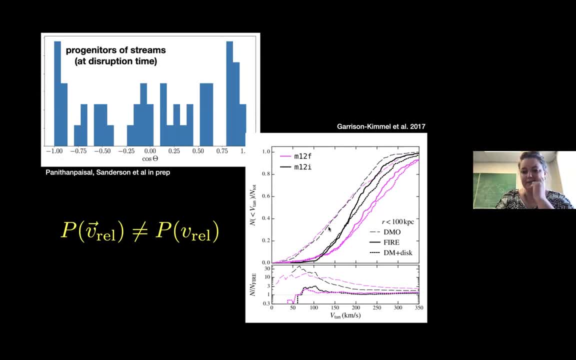 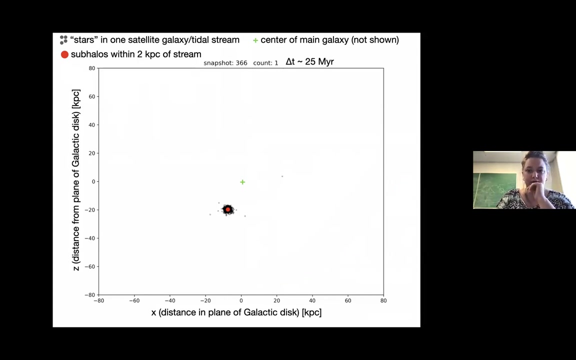 is a manifestation of the fact that the disk is effective at depleting subhalos preferentially on plunging orbits, And so there's a little bit of a bias towards subhalos on orbits with larger tangential velocity. And finally, let's go back to this business about the galaxy. 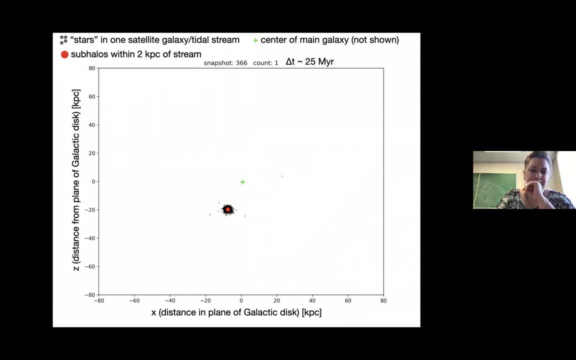 being a busy place. There's been a debate lately in the community over how much of the noise that I showed you when simulating these tidal streams comes from numerical effects as opposed to actual interactions with subhalos, And I think that a lot more of it comes from subhalo interactions. 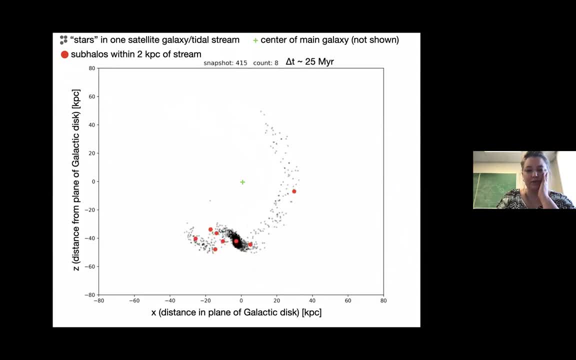 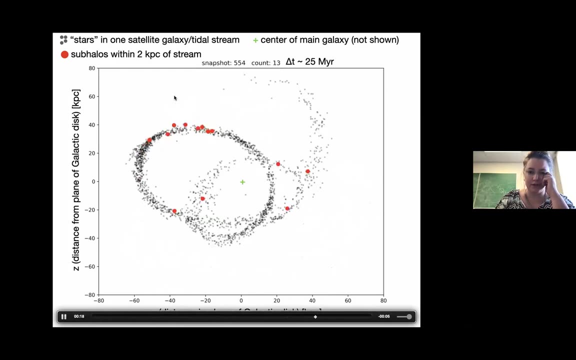 than people may want to admit. So these are all. these little red dots are all the subhalos that come within two kiloparsecs of this tidal stream, which is extracted from one of our cosmological simulations. Not all of these impacts are very strong, but there's definitely a diffusive element. 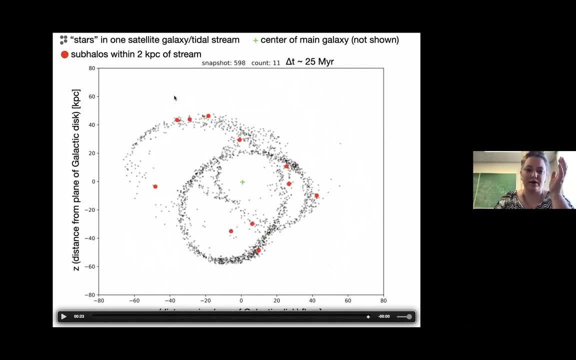 to this process that has so far been neglected in modeling, And I think it's important to understand that any particular interaction that might open a gap in this stream is going to be layered on top of By the many other interactions that might be less strong with subhalos as the stream evolves. 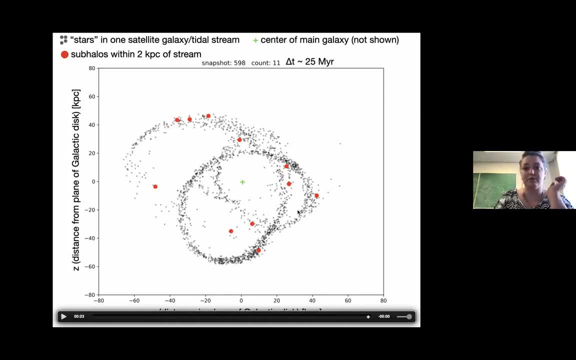 And in many cases, the stream has been around long enough for this to be a large number, So we're in the process of tracking this sort of interactions and quantifying them in terms of their ability to scramble the stars and cause perturbations in tidal streams for a suite of about 100 streams over. 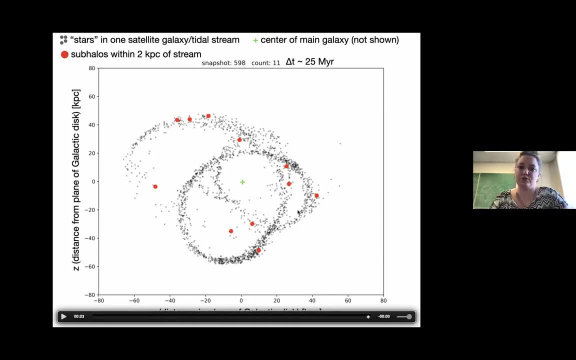 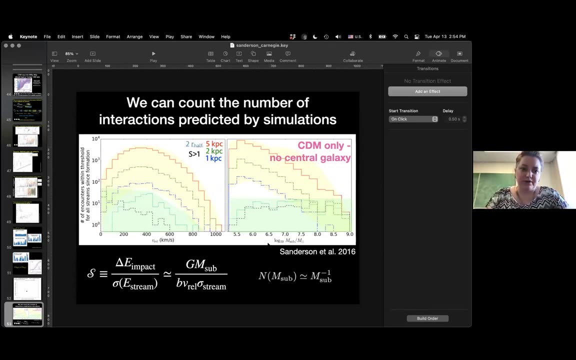 order 15 different galaxies, And so we're going to be doing a lot of simulations with different assembly histories, And this should give us some better and more realistic statistics on what to expect here. What we plan to do- these are some results from an old set of simulations- is to count the number of interactions. 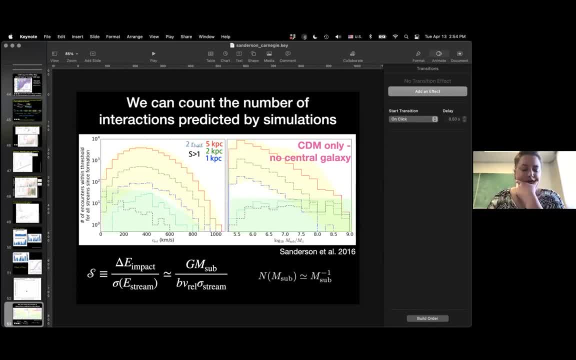 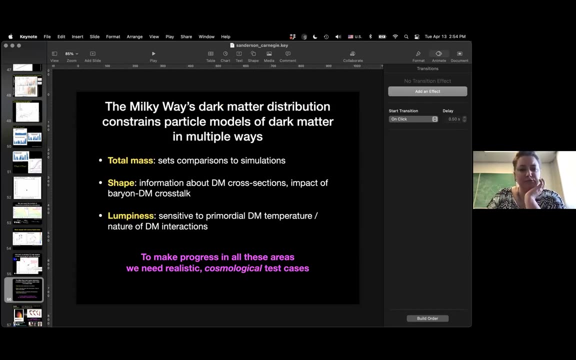 and see how they scale with the strength of the interaction which I talked about earlier, And so we're working on repeating this now. So, just to wind up, we talked about three ways in which you can test dark matter by looking at the galaxy. 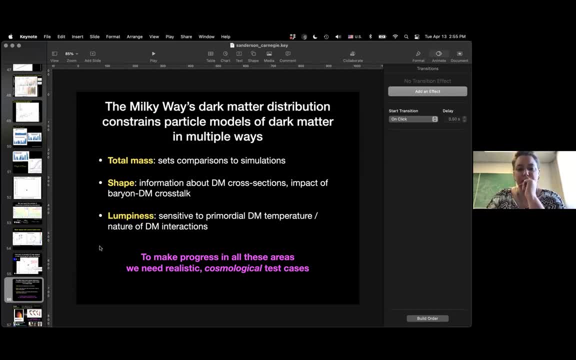 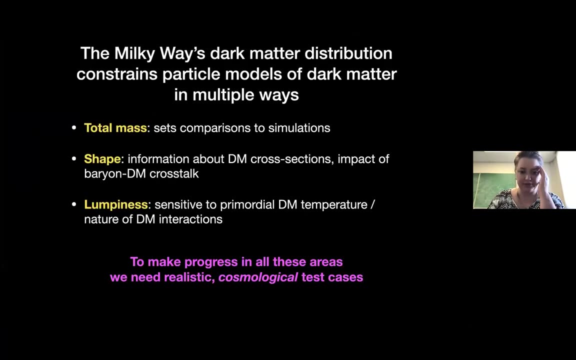 But in all of these areas, I think it's pretty clear that we need to use test cases and make comparisons with realistic, cosmologically motivated simulations of the Milky Way, which is what brought me to working with the FIRE Collaboration In the first place. 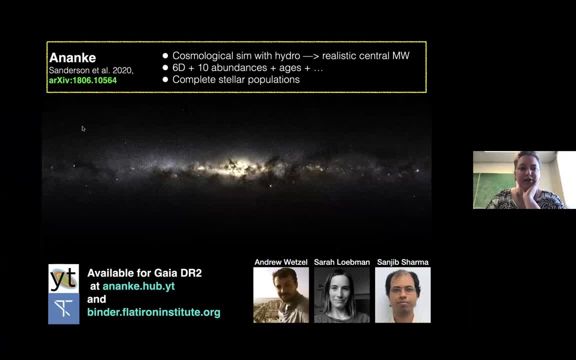 And so we've started to make some steps towards this. One that I didn't talk about a lot, but which you're free to ask me about, is to synthesize Gaia surveys of some of the simulations. So we chose three of the simulated systems and then put the sun at three different locations in each one of those, for a total of nine catalogs. 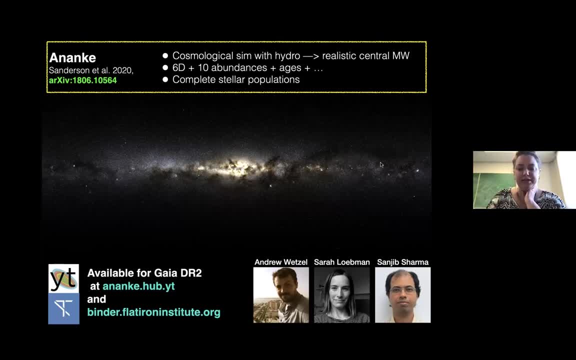 And then we simulated the complete stellar populations and then what Gaia would measure For their positions and proper motions and photometry and so forth, And these are available for Gaia-DR2 right now. We're working on an upgrade for Gaia-DR3, so stay tuned. 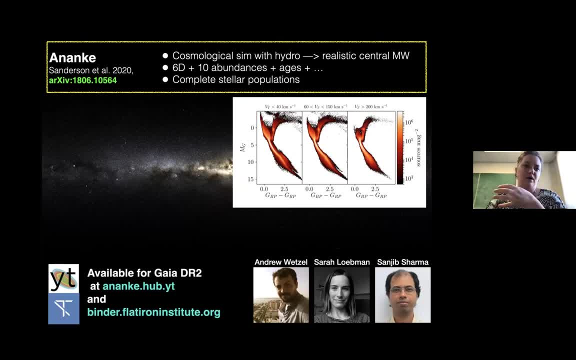 And we're about to release, as part of the next Sloan data release, a value-added catalog that includes an apogee error model for the Gaia-DR2 versions, which has been put together by my grad student, Farnik. 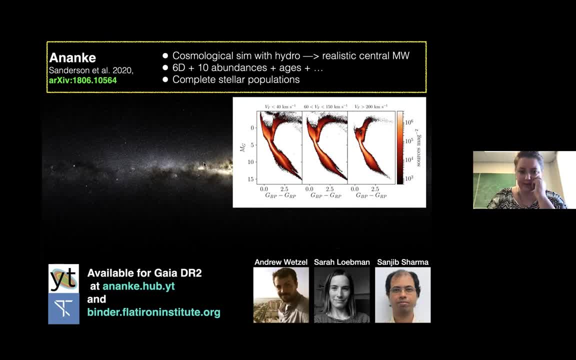 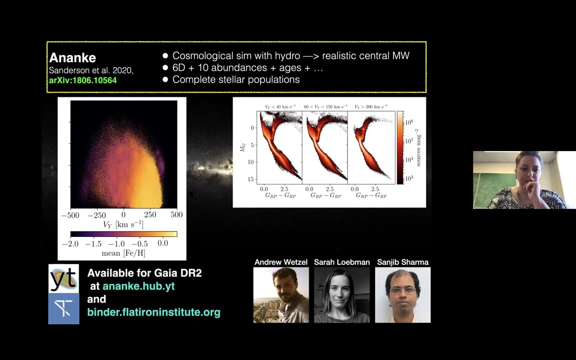 But the underlying contents include the magnitudes and colors of all of the synthetic stars in each of these galaxies, just as if they were Gaia, Plus abundance information and phase-based information, as if Gaia had observed these galaxies while living in them. 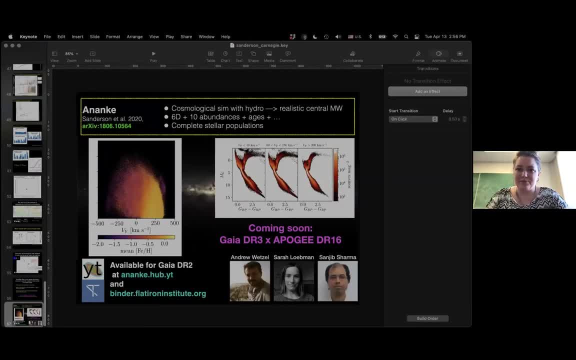 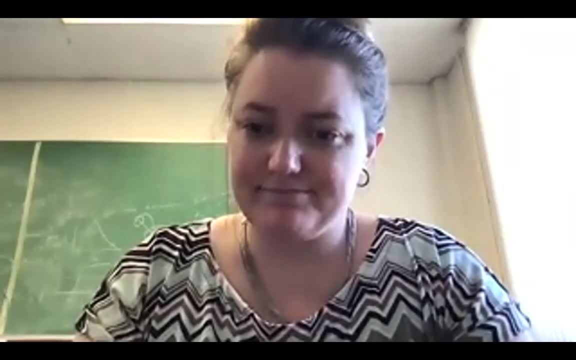 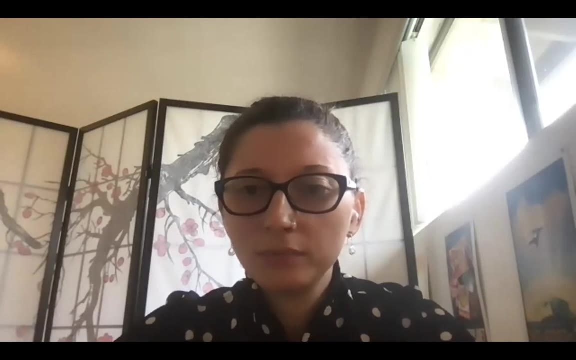 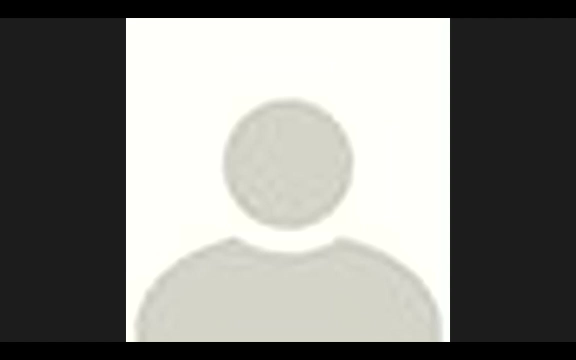 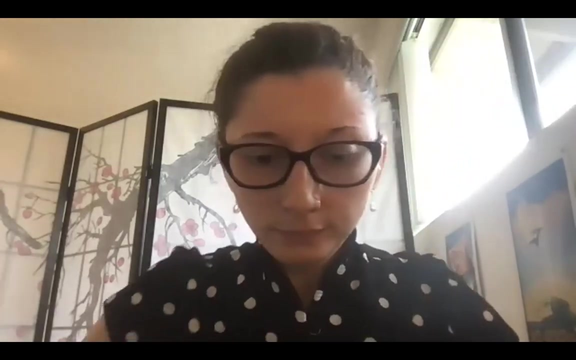 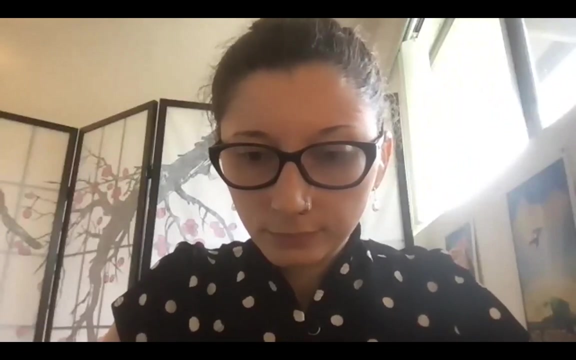 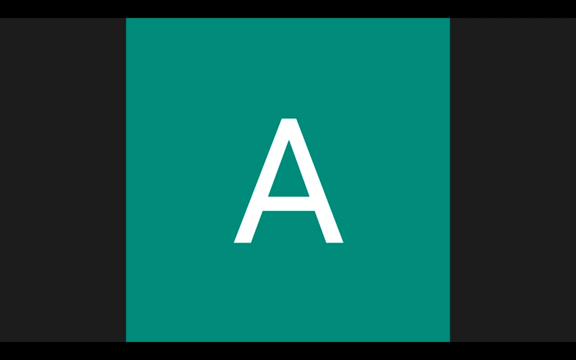 So with that advertisement, all wind up. thank you very much for your attention today. Thank you, Thank you. I'm just trying to get an idea of how to translate that into action space, because I think the two are related. Yes, here. 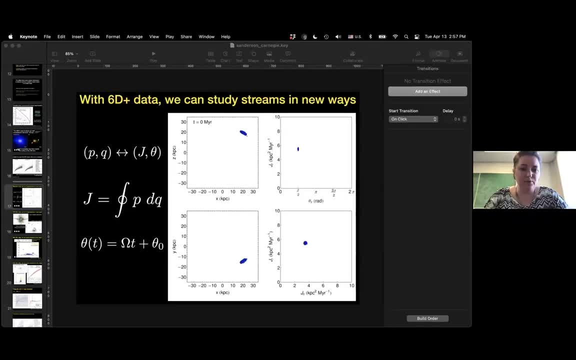 I'll do this real quickly. So the way that they're related is as follows. Here are the actions which are computed by integrating the momentum in each conjugate coordinate across its conjugate position through one cycle of its bound orbit per star. 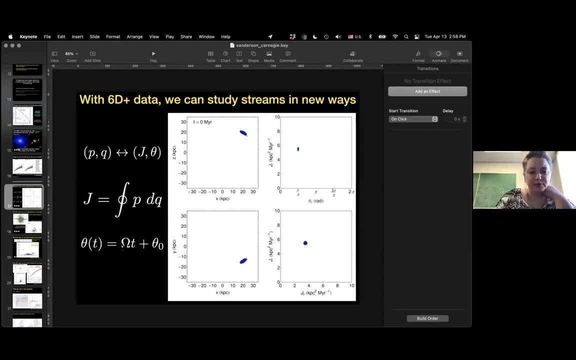 And then the frequencies which come in down here. formally are the derivatives of the Hamiltonian, The derivatives of the Hamiltonian with respect to the actions, But functionally, what they are is the rate at which the conjugate angles increase linearly with time. 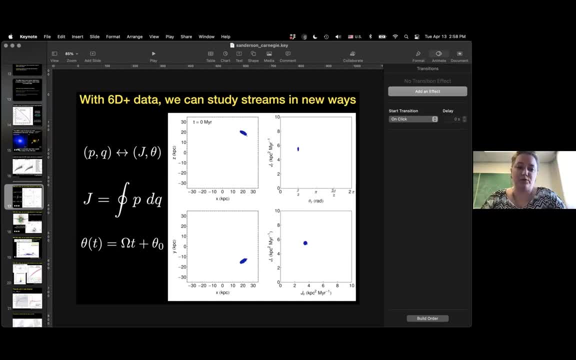 So you can think about them as, literally, the orbital frequencies of, or literally the frequencies of oscillation of the bound orbit in the coordinate system where the potential is close to separable. So, for instance, if you have a disk, you usually assume that the coordinates are axisymmetric. 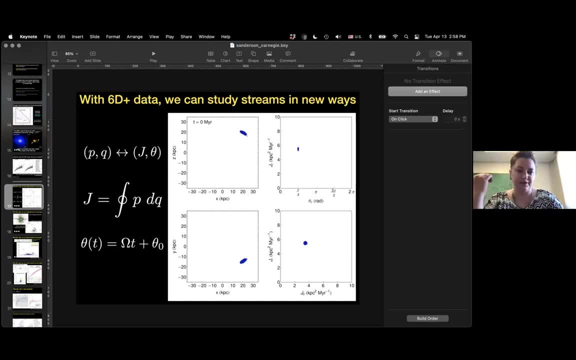 Or close to Or that. that's a good model for the symmetries of the potential. And then your orbital frequencies and your actions and your angles would all be couched in a sort of like cylindrical radius phi in the disk plane z coordinate system. 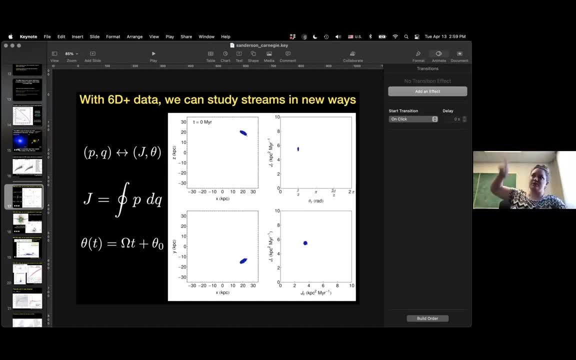 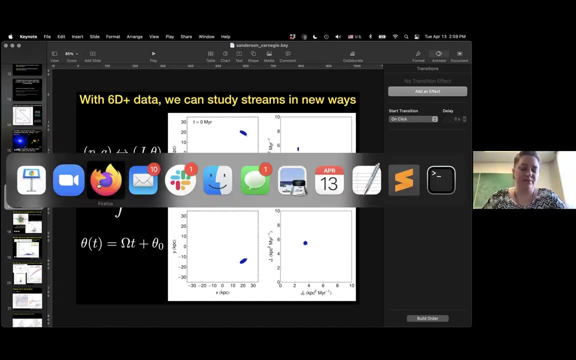 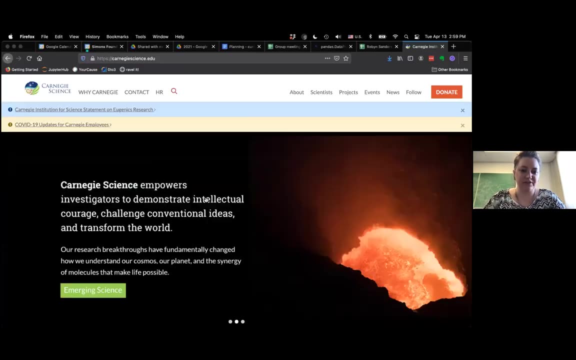 And so you'd have one frequency that was this frequency, one frequency that's this frequency, and one frequency that's this frequency for each star, And the sort of the size of those oscillations is what the actions are telling you. Does that clear things up a little bit? 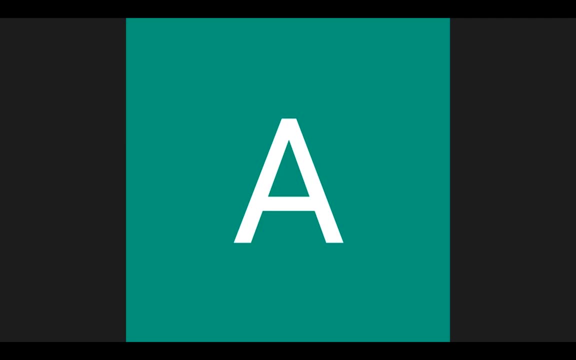 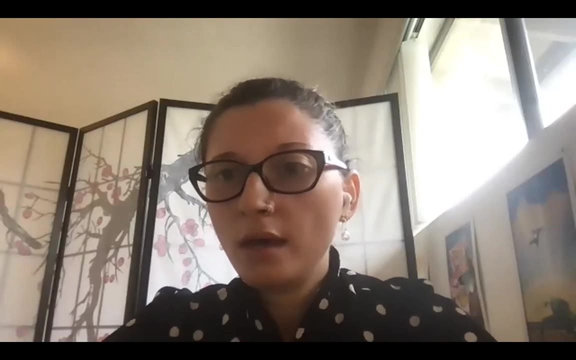 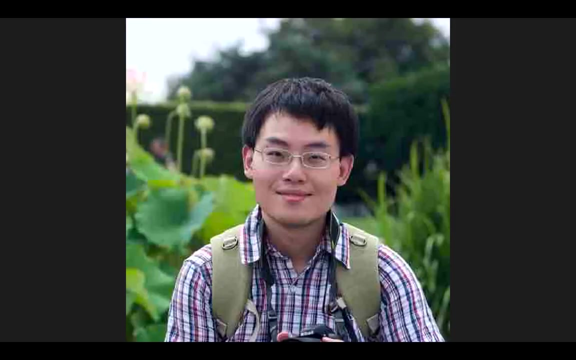 Yeah, I see That makes sense. Thanks, Okay, Can you hear me now, Robin? Yes, Okay, Good, It's fixed. So why don't? I think Feng Zhou has had his hand up for a while, so perhaps you can go next. 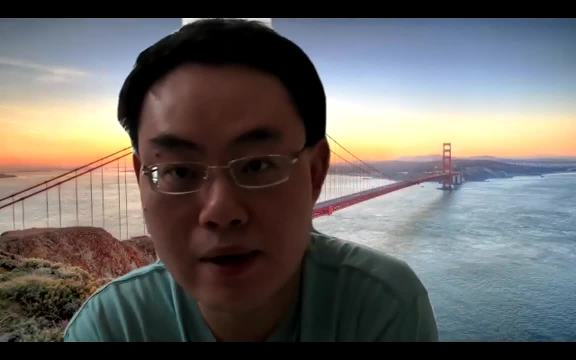 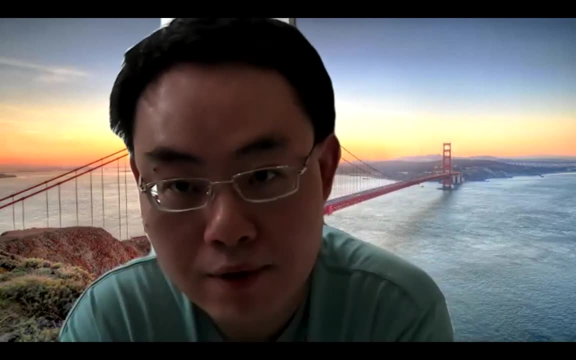 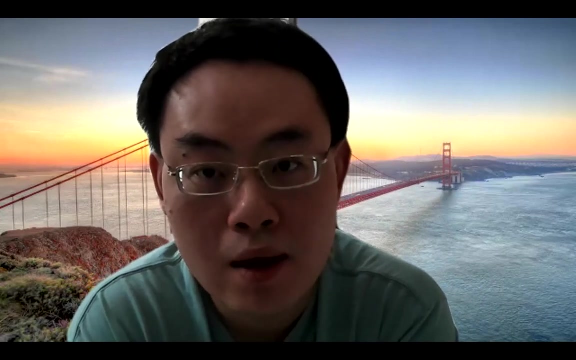 Sure Thanks. So I wonder, I think a very interesting point, which is that the encounter rate of cold streams and the substructure depend on both the phase-based distribution of subhalos and that of the streams. So I wonder: do you have intuition or preliminary results on how would ICIDM impact this encounter rate? Because, on one hand, I expect ICIDM subhalos to be more prone to disruption, so the phase-based density of subhalos would be lower, But the stellar stream phase-based density may be higher, right? Yeah, I think you're right that this is not going to like that. this is going to be competing effects. 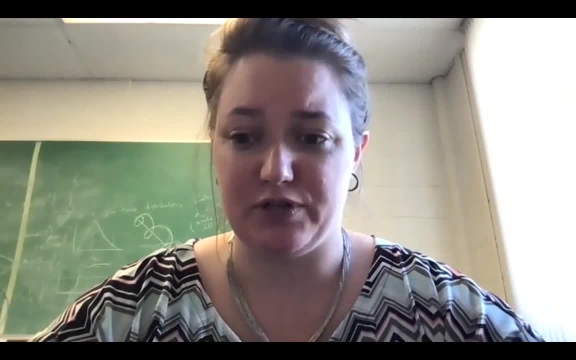 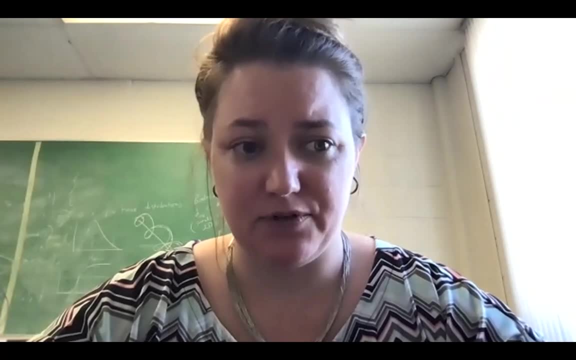 As we are classifying and following the streams in the CDM simulations, we're also, in parallel, doing the same thing for the SIDM runs, And so we'll be able to directly compare them for things that are otherwise identical, but for the thing. 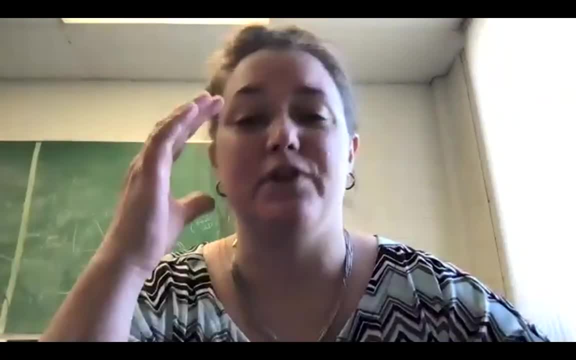 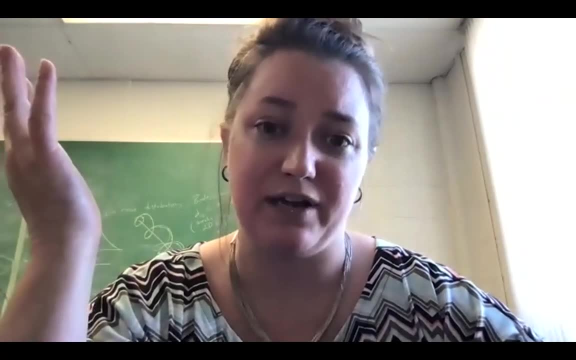 But there have been a number of different predictions that have come out that would come down on both of these sides, And I don't know which is the effect that's going to dominate, whether it's the fact that you get more tidal streams but then, like, dynamical friction might work a little differently. So I'm not sure about that. And then the cores aren't as much less dense in simulations with baryons as they are in the simulations without baryons, Because the like in the case of Milky Way mass stuff- you're going to have a lot more of that. And then, like with Milky Way mass stuff, you actually get a denser central dark matter density in an SIDM halo because the dark matter can respond to the deepening of the potential due to the formation of the galaxy better in SIDM than it can in CDM. 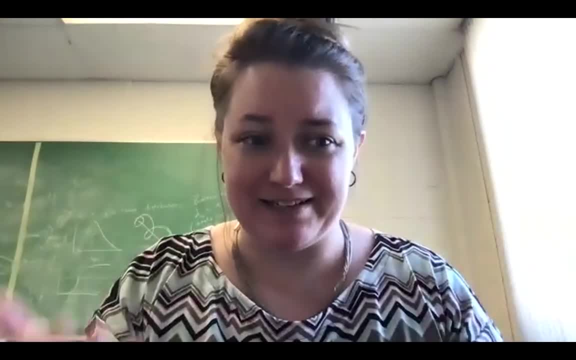 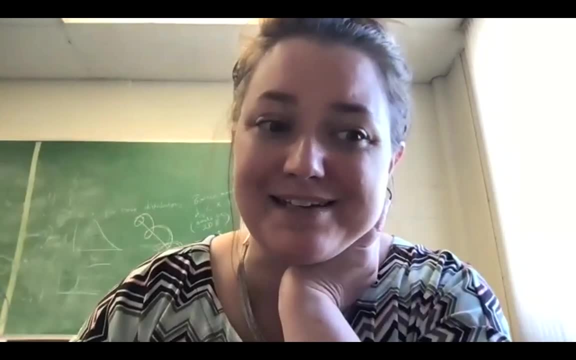 So I don't know which way this is going to fall, because there's a lot of different things that we just need to see which one is the one that dominates, or whether they all compete out. So I'll be fascinated to see what the answer to that question is, but we don't have it yet. 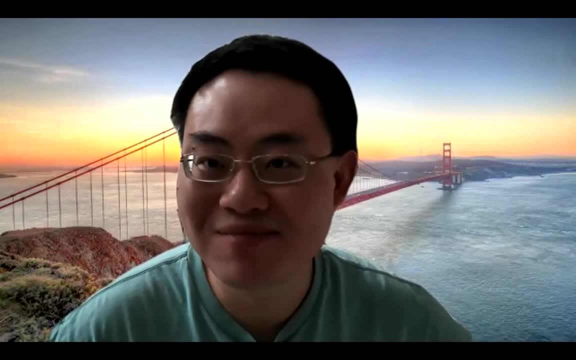 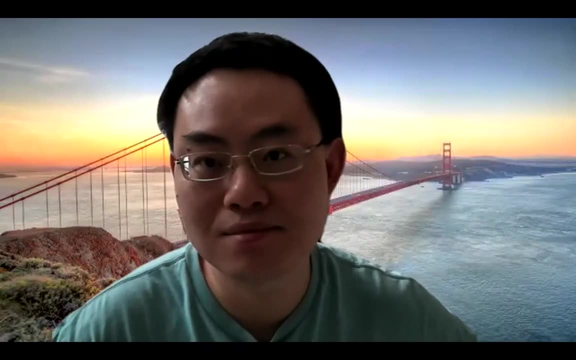 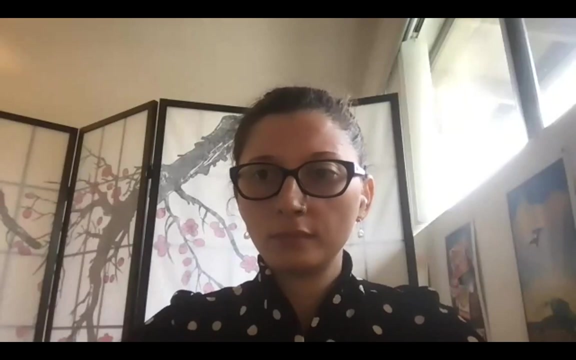 Yeah, me too. Yeah, It just seems to be a very interesting area. yeah, Yeah, Thanks. OK, so Josh also had a question. Yeah, so, Robin, in the first section of your talk you showed a nice little movie of how. 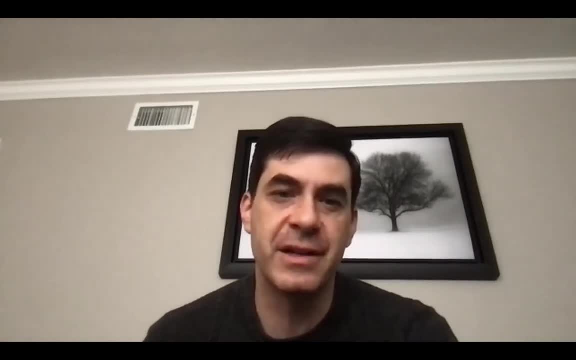 if you leave the shape, the functional form of the potential fix and change the mass, then it's easy to zero in on exactly what the correct mass is, And so what I was wondering is how much that changes if you don't know the functional form. 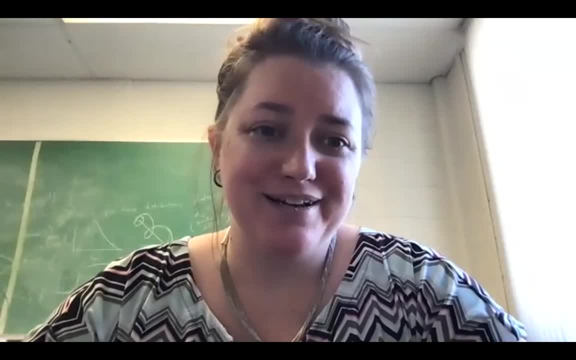 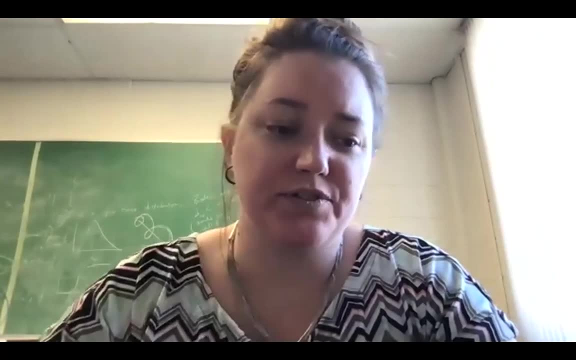 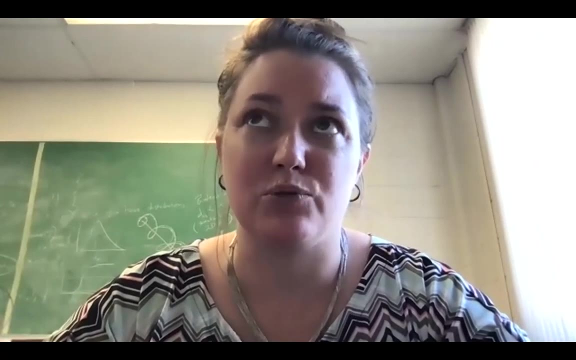 of the potential. That's a great question, Josh. I should have paid you to ask me that one, because this is actually something that I've been working on with Stella Reino, who's a finishing graduate student at Leiden, who is the one that did the work with the four actual streams. 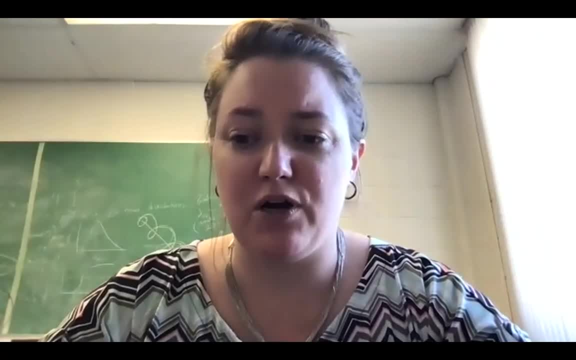 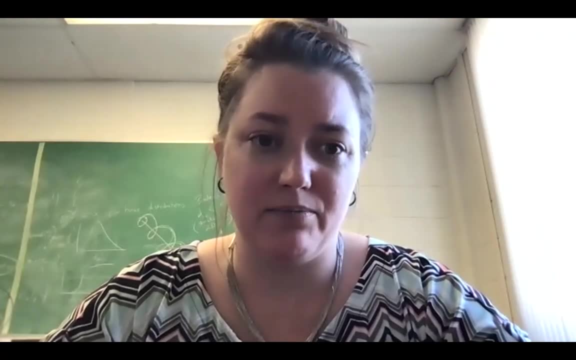 and applying this technique to those, And so for her, For her follow-up, we're actually trying to dig into this issue a little bit. In my initial tests with a cosmological halo, the model that we used was not a very good representation. 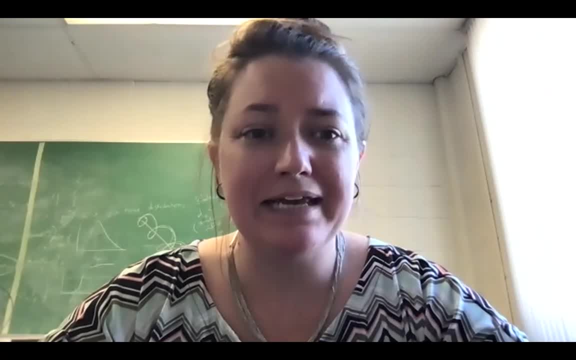 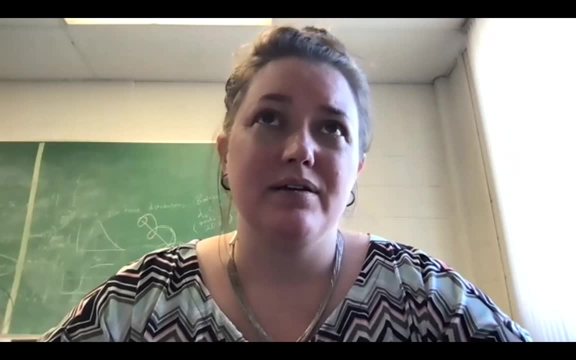 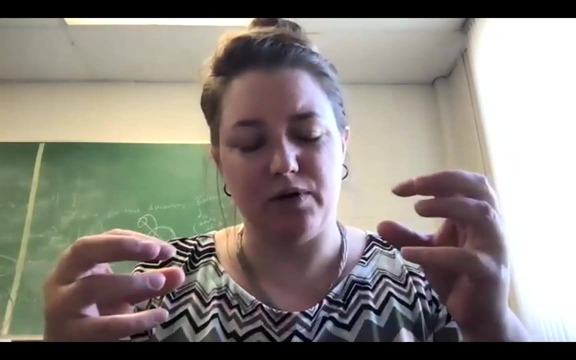 of the mass profile and it came out OK. The way that you found in that case, the way that the mismatch between the model and the actual profile manifested itself, was that there was a region where you could fiddle with it. You could fiddle with potential parameters a little bit. 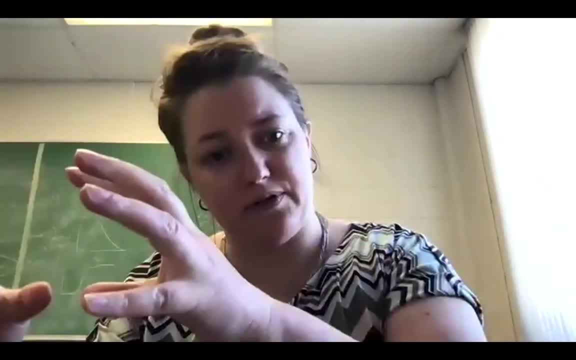 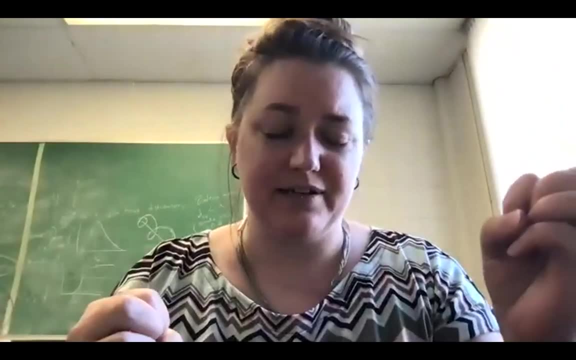 And for some combinations some of the clumps would get tighter, And for some of the other combinations other clumps would get tighter And there was no way to pick the parameters so that every single clump individually was the tightest, And that was kind of a clue that you needed some extra flexibility. 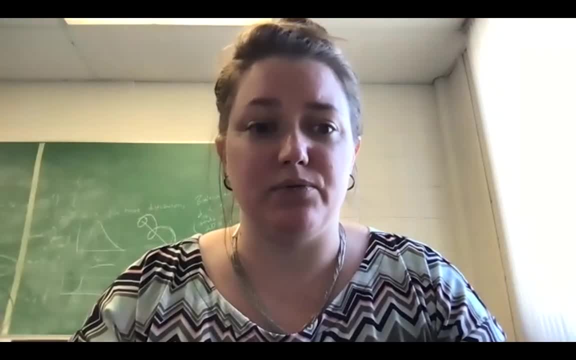 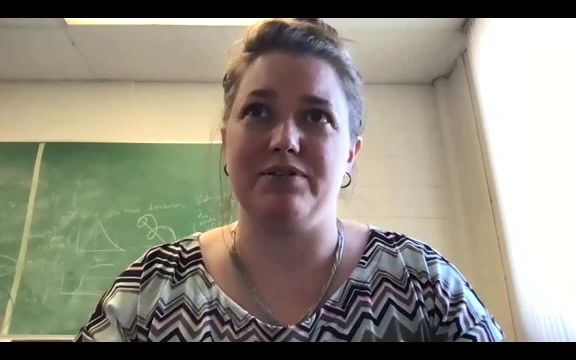 in your potential, And so, when we set out to do this in the real galaxy, Stella was working with this two-component Steckel model, which, despite what a lot of people seemed to think, is actually a pretty decent model for the galactic potential. 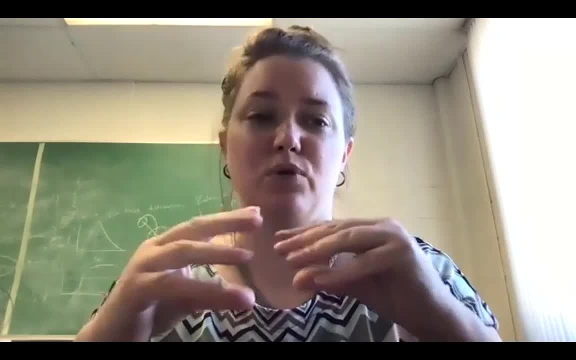 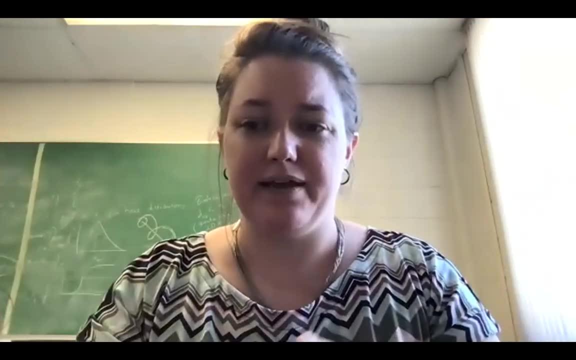 So one of the components ends up taking on mainly the role of the inner part of the galaxy, and then the other takes on the outer part, And this gives you a lot more flexibility. And in fact, when we first tried it with a single Steckel, which 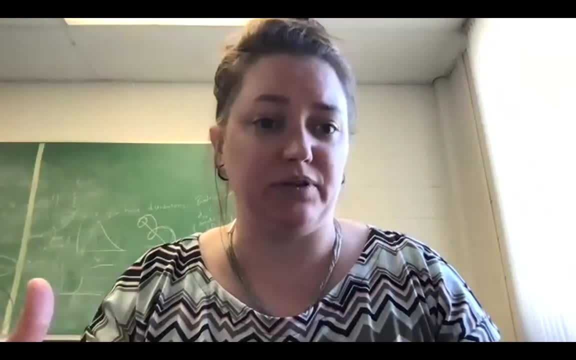 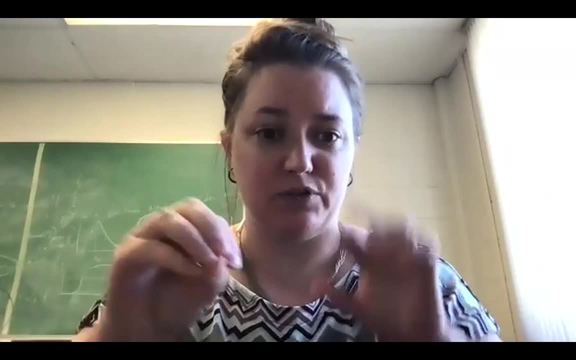 you know, has got to be a bad approximation, because you're completely ignoring the fact that the halo is mostly round and the disk is mostly flat, and you see a lot of that. It's a lot of this discrepancy between individual clumps, in that case to the point where they gave completely conflicting 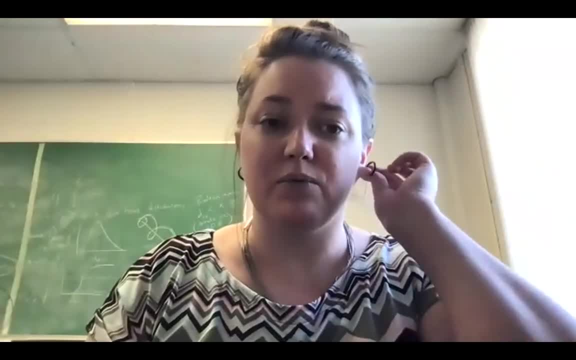 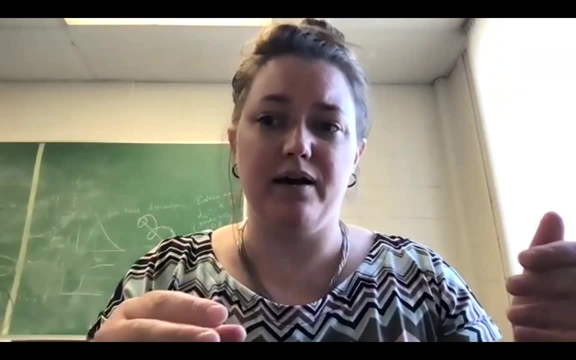 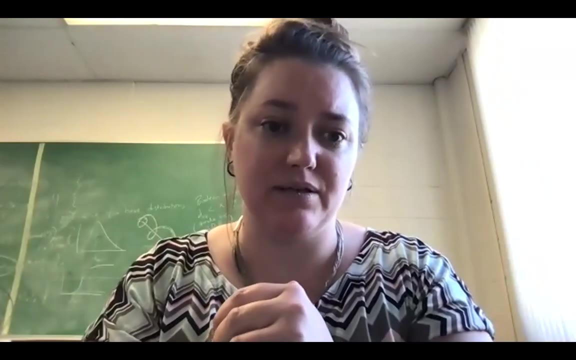 individual estimates of the mass of the parameters. And then when we introduced the flexibility of a second component, which is like loosening up the functional form, then you got much more agreement between the results from the individual streams, And when you combine them, you got something that made sense. 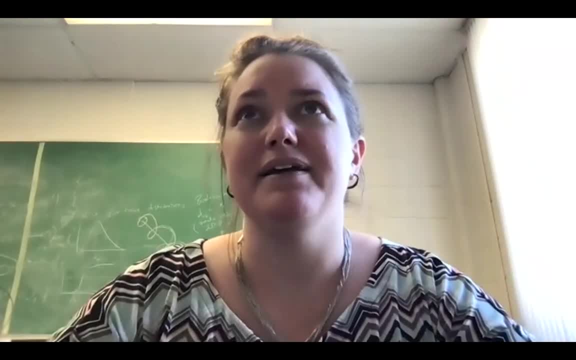 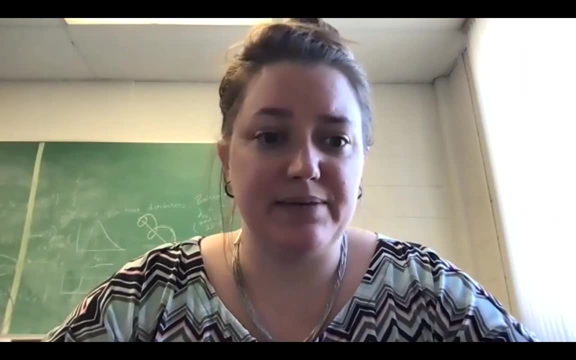 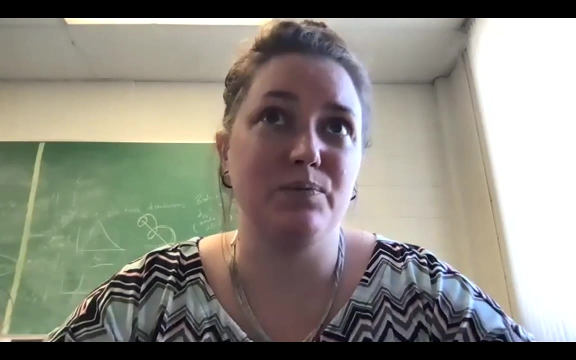 So you see your systematic- I don't know if systematics is the right way to put that, But so now what we're doing is we're trying the same thing out on some of the simulated streams in our galaxies And then playing also. what we found is just as important. 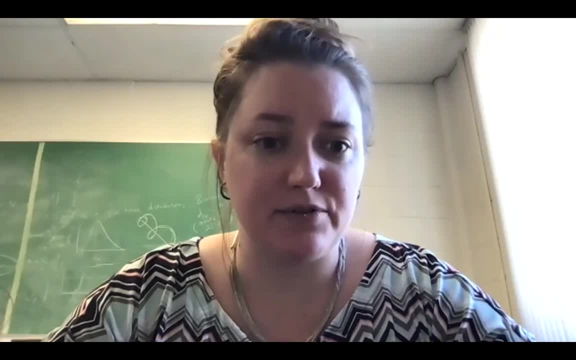 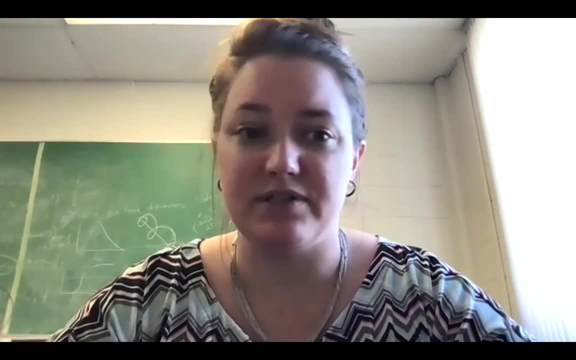 seems to be the orbital phase of the stars of each stream that you include in your sample. So if you were for some reason like, say you live in the center of the galaxy, to only get mostly stars and streams that are near pericenter. 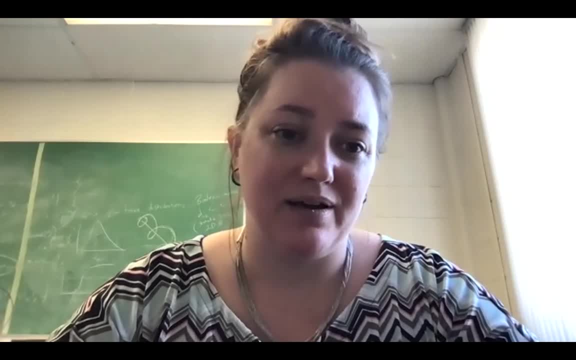 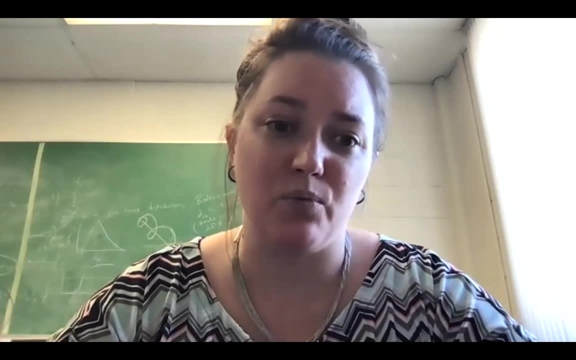 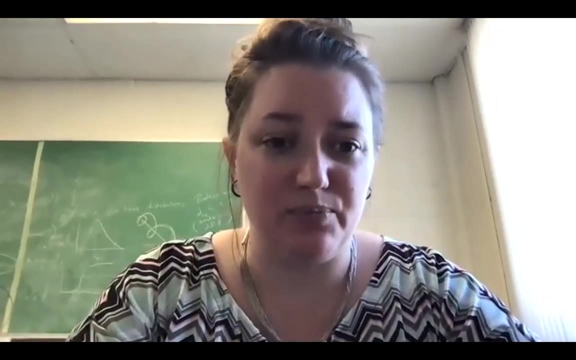 You actually get a pretty terrible mass estimate because they're relatively insensitive to what's happening at large distances And you have a lot of room to roam with your epicenter distances if you don't ever measure stars at epicenter, And so we've been playing with this a little bit. 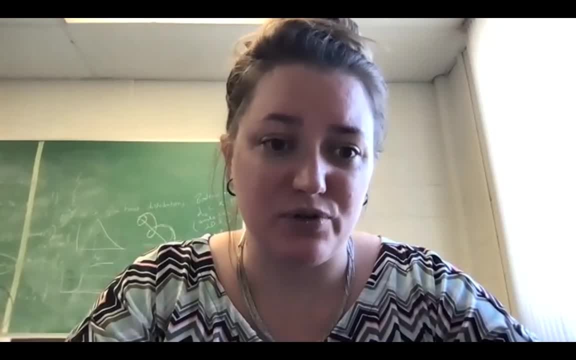 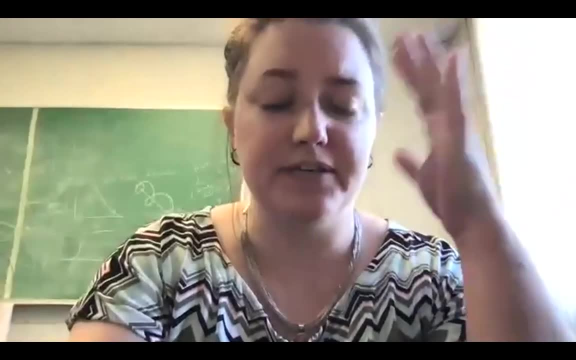 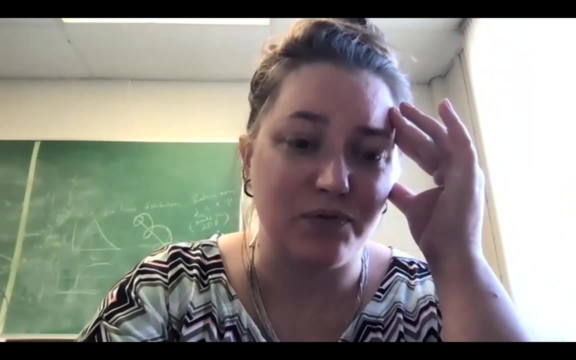 to see whether you can beat that down just by piling on more streams, Or do you actually need to be sensitive to what orbital phase everything is in, and so forth. But I think, Yeah, Yeah. So that's sort of the status to which we've. 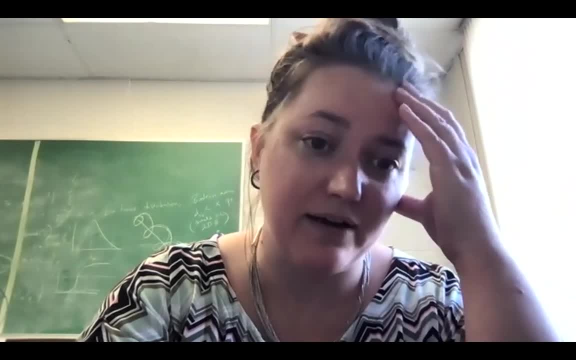 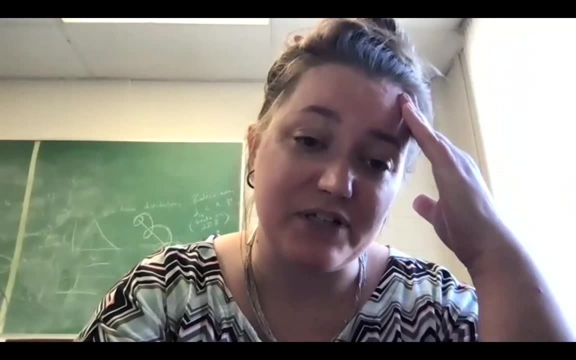 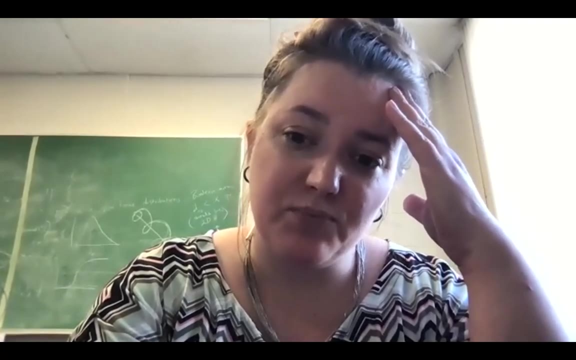 explored various sources of systematic error in this thing. The other thing that we've been working on, incidentally in the group that I didn't even talk about, is I have a student who's been studying how to build completely agnostic models by using low order of multiple basis function expansions. 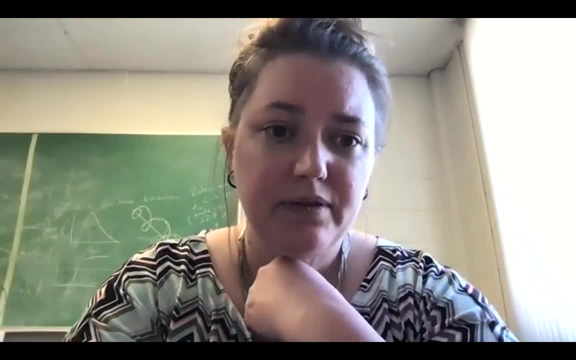 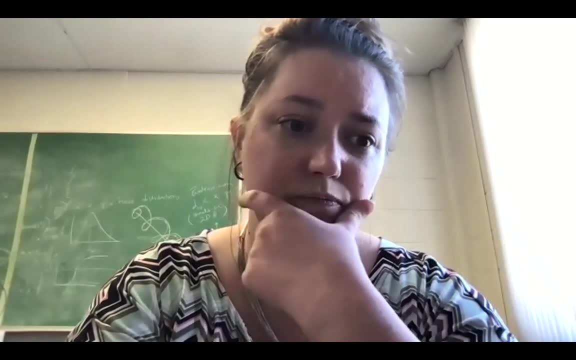 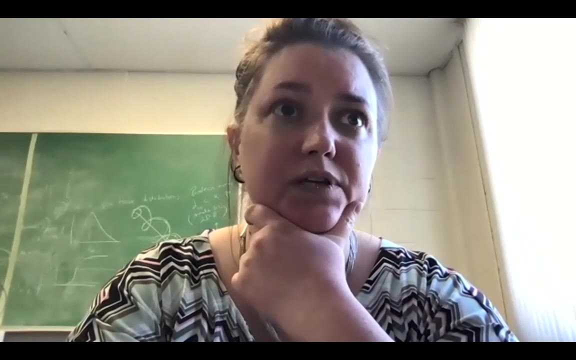 to represent the potential of the halo And then just treat the disk as we know. it is because we've pretty much modeled the mass distribution of the disk stars fairly well And that also seems to be a little more robust to the types of perturbations that people are pointing out. 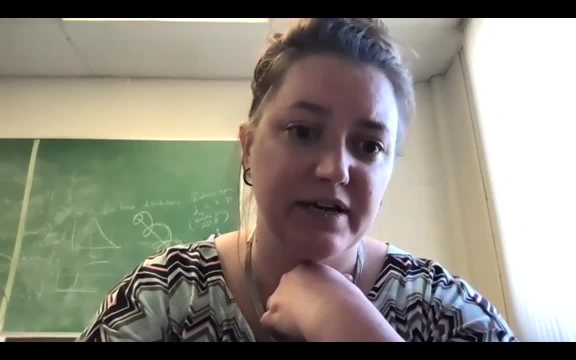 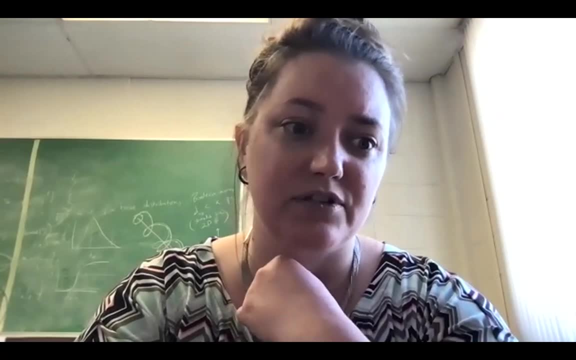 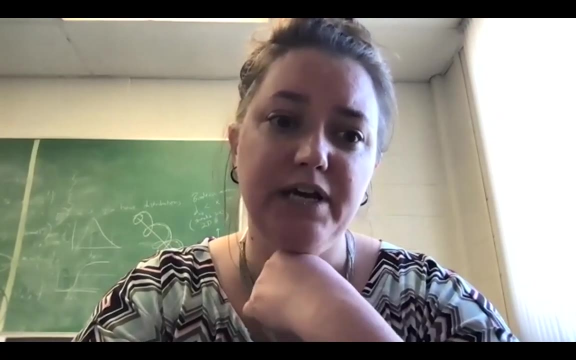 from mergers like the LMC and Sagittarius, where you expect some sort of wake from the mass distribution And the dark matter disturbances associated with the merger. It can absorb a little bit of that stuff if you give the potential model a little more flexibility. 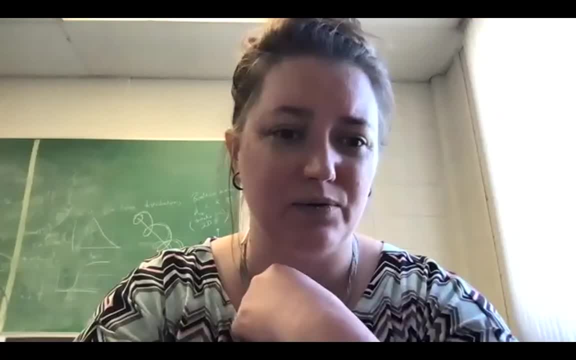 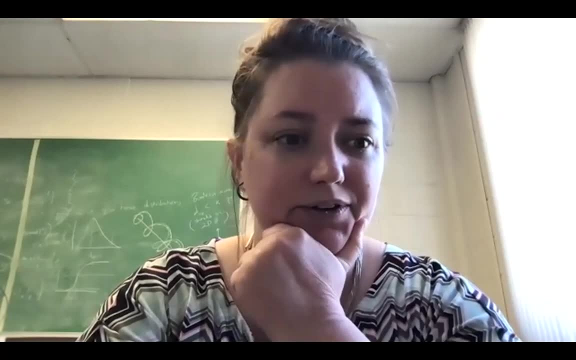 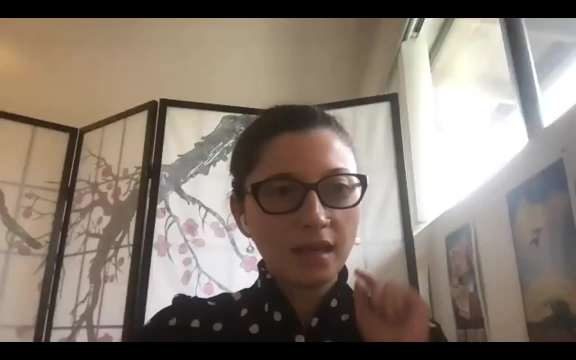 That's not necessarily a new conclusion, but it's one that I think people are starting to realize that we need to know more and more, given the direction things are going. Thanks, Perhaps Ting can ask Her question very quickly, and then I'm sorry, Alex. 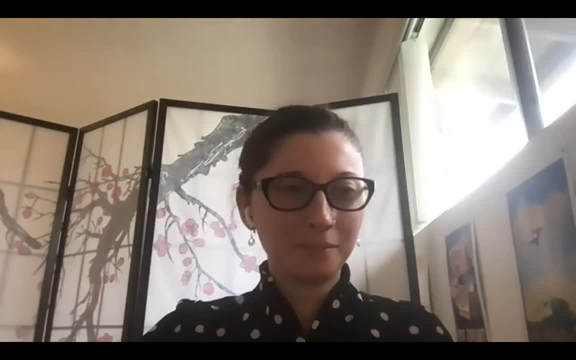 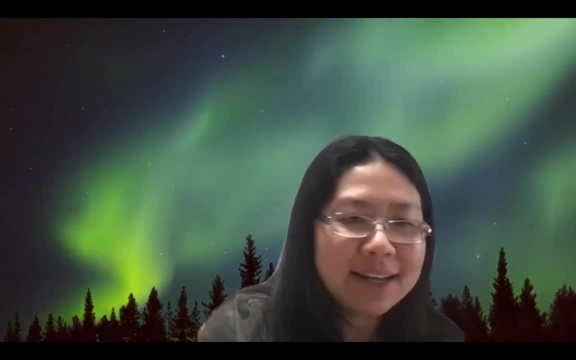 I think we should end after that. So I have two questions actually, But feel free which one you want to answer, because I think both are interesting to me. The first is related to the first part of your talk, So I understand that you are using the clustering action. 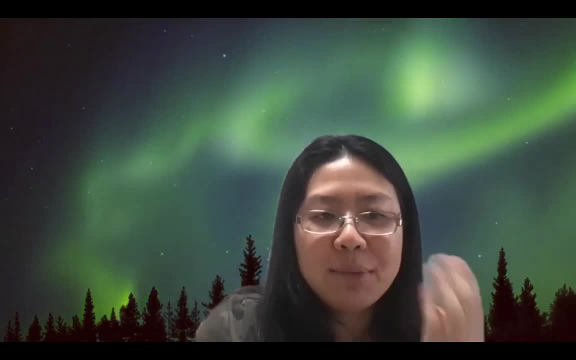 space to constrain the Milky Way mass. But we also know that the Milky Way has satellite galaxies like the LMC, which kind of perturb a lot of the space. So I'm going to ask her question very quickly And then- I'm sorry, Alex, I think we should end after that. 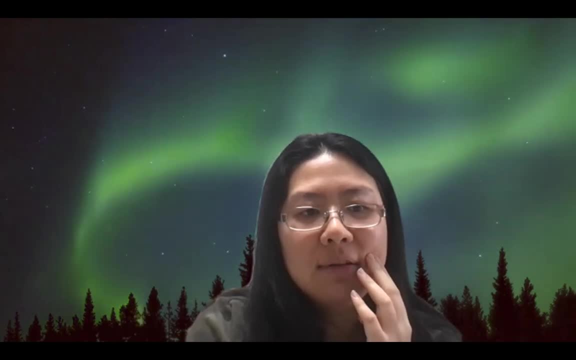 So I guess my question is so what you think the way to properly deal with this is that just to deal with the stream that we know has no significant perturbation from the LMC and use those to constrain the mass, Or, if you can also include a LMC model. 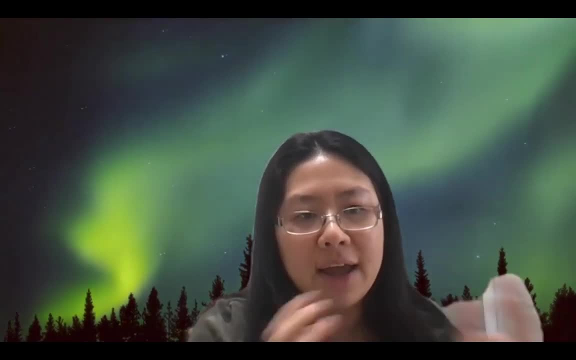 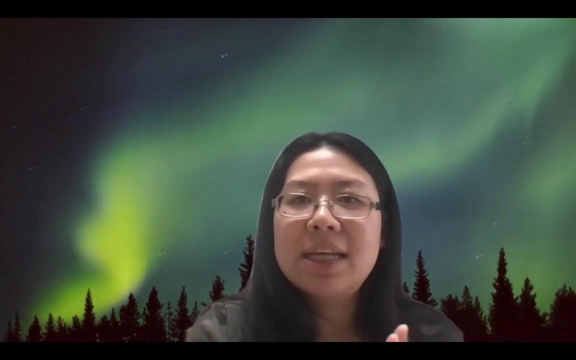 like in the whole kind of fitting and doing like a fitting with the LMC and the Milky Way mass and shape simultaneously. And the second question is So the third part of the talk you are talking about, like substructures using dwarf galaxy streams. 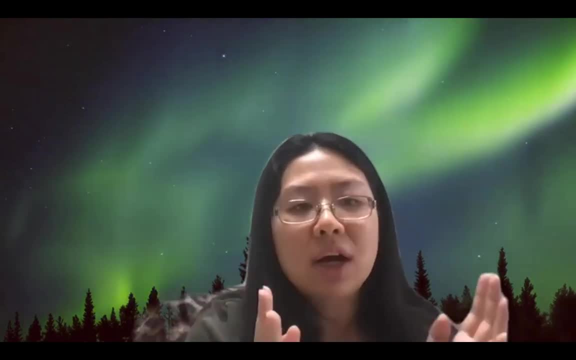 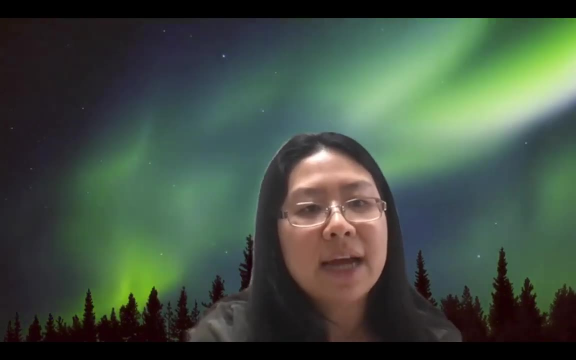 But my understanding, like a Sagittarius stream, like we always talk about saying, constrain the subhalos using cold streams, mostly from global cluster, because, like, if the stream is dynamically too hot, like a Sagittarius stream has like 10 to 15 kilometers, per second, then those stream. basically the gaps it formed will get just filled back after a few million years. So I don't know, like if this is a thing problem for you and that you have some certain kind of constraint for what is the minimal- sorry, what is a maximal velocity dispersion? 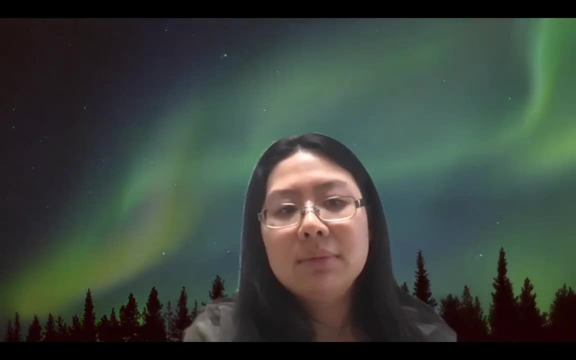 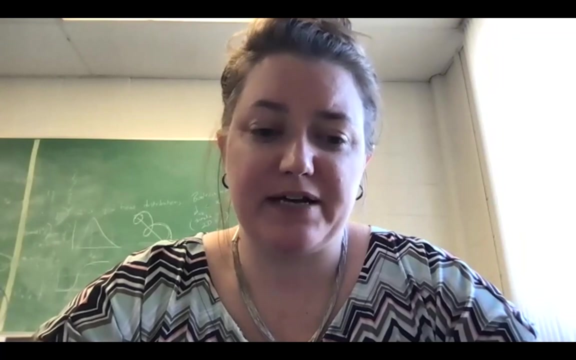 for the stream will be useful for the study you are talking about here. Yeah, All right, I'm going to tackle the second one and we can talk, because the first one is a shorter answer and I'll get back to it. So I think you're right that the Sagittarius stream is probably 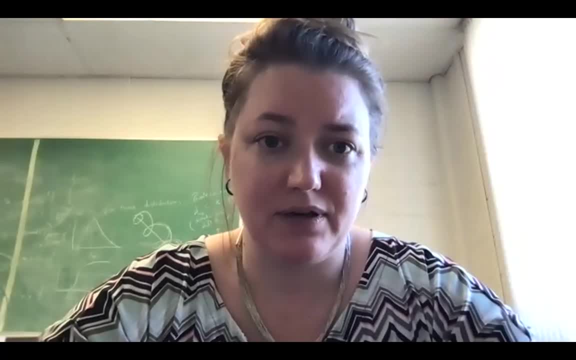 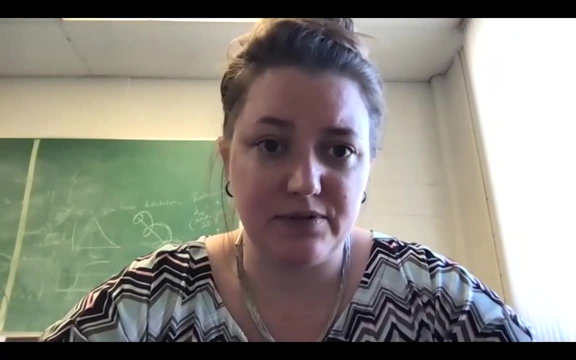 not the best one to use if you're trying to do this with satellite streams, But there's a long way to go between that and like a globular cluster, And some of the thinner streams from lower mass satellites are probably good candidates for this. There are two other aspects of this that I think have been neglected that we're trying to assess right now in the cosmological simulations. One is the fact that things like Sagittarius usually are part of a group in fall And they bring in a set of their own substructures on orbits. 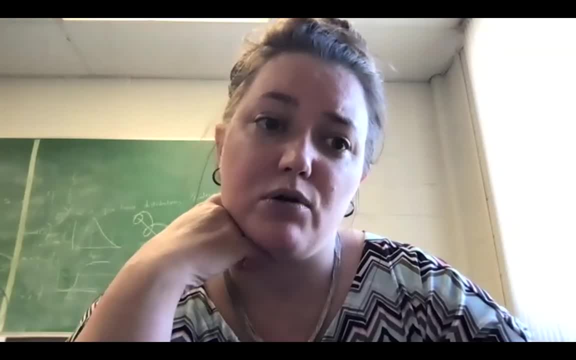 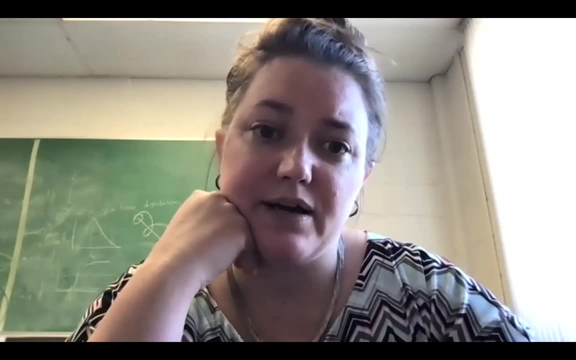 that make it possible that you could have repeated low velocity interactions with the stream over time And that may amplify the signal for larger streams like that. And I'm not sure how, to what extent that's the case, But I think it's an interesting thing. 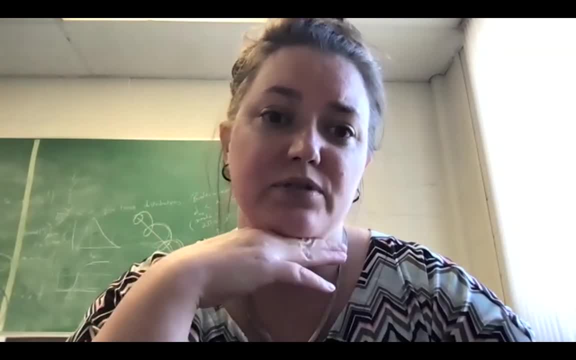 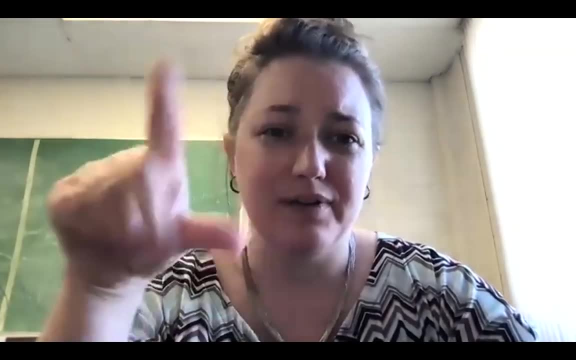 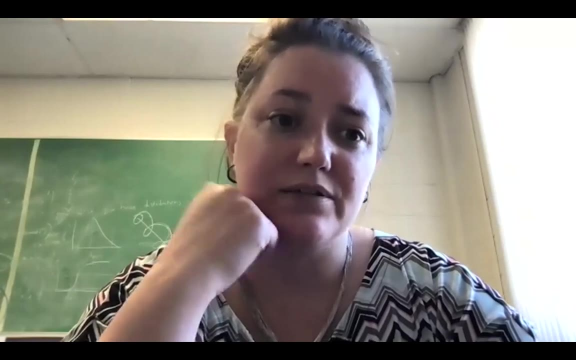 that we're trying to follow up is to see whether this kind of repeat encounter happens more frequently for stuff that is in a more massive stream, because it might be helpful in adding those to the population, because otherwise, you're right, The velocity dispersion is too big to really open up a gap. 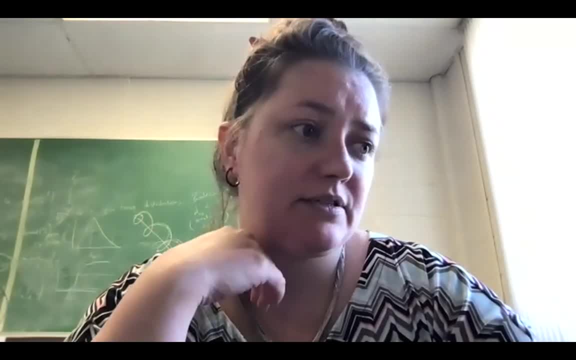 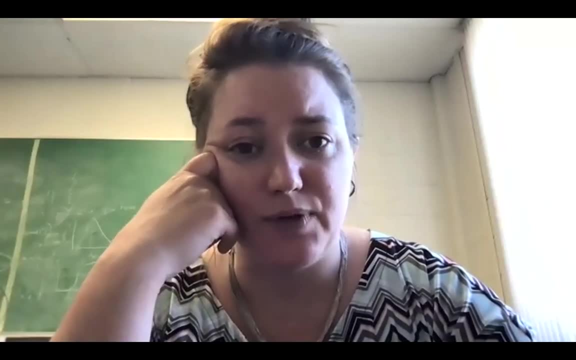 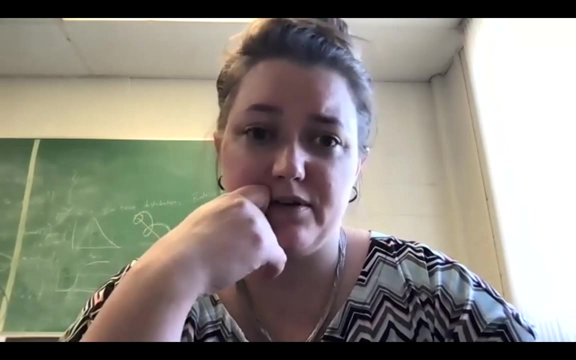 The other part of that that we're hoping to constrain is to get a better idea of the encounter rate of even weak encounters, and then be able to better estimate the floor in the velocity dispersion that you would expect given that encounter rate, Because the low mass interaction or the less strong interactions 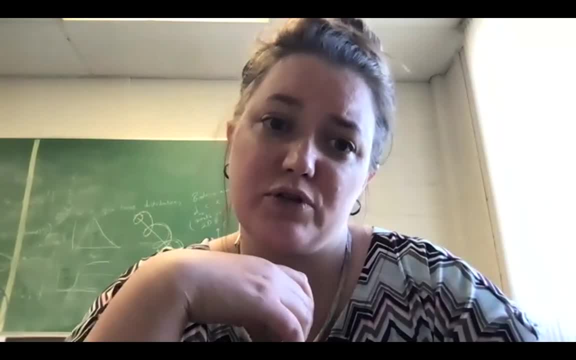 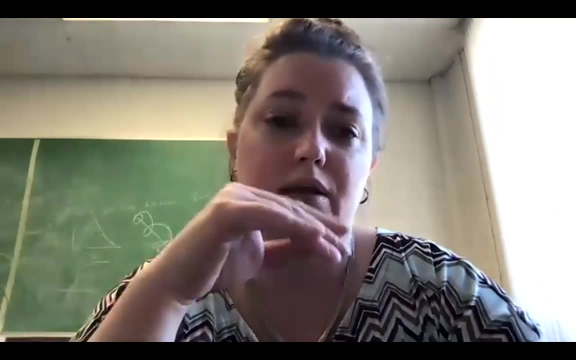 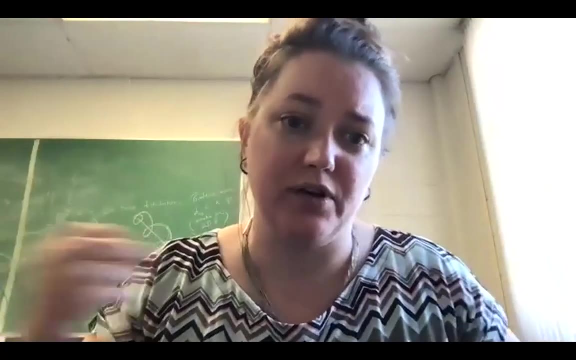 won't necessarily do anything to the structure of the stream and density, But they're going to be competing against. So that kind of diffusive heating is competing against what I would call gravitational cooling. Just like Louisville's theorem, the thing is spreading out and getting colder over time. 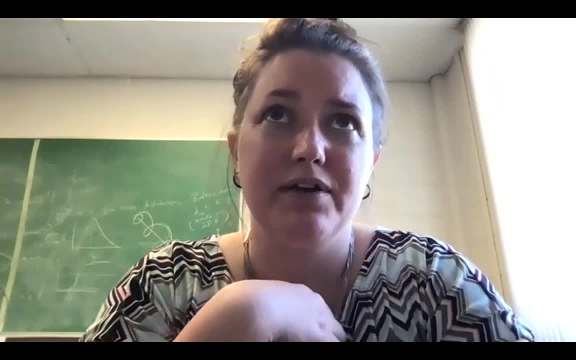 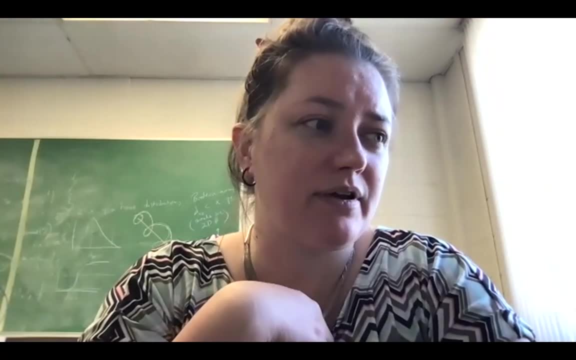 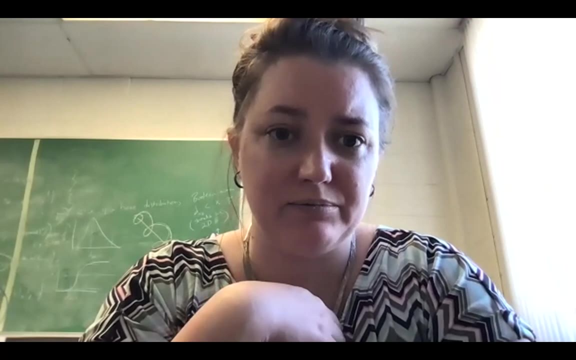 And it's not obvious to me that there have only been a few attempts to make that calculation, And they've all been with models that didn't account for things like the baryonic depletion of subhalos And all the anisotropies that we're finding. 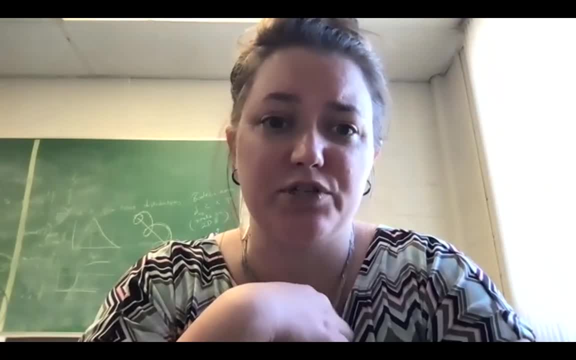 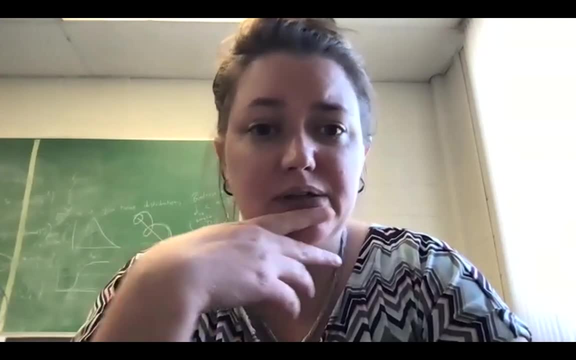 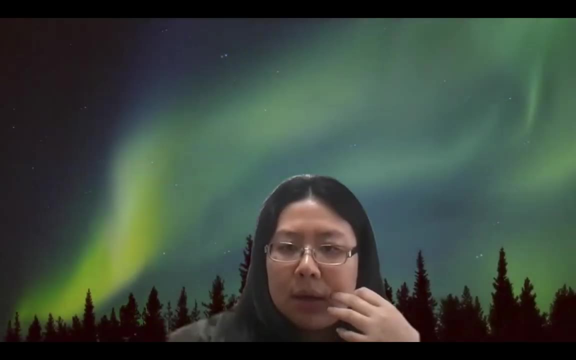 So what I'm hoping to do is update those estimates and see which of those processes actually wins in a realistic case. We'll see. So your first question, though, is about the LMC and taking that into account with models. We're just starting to look into this. 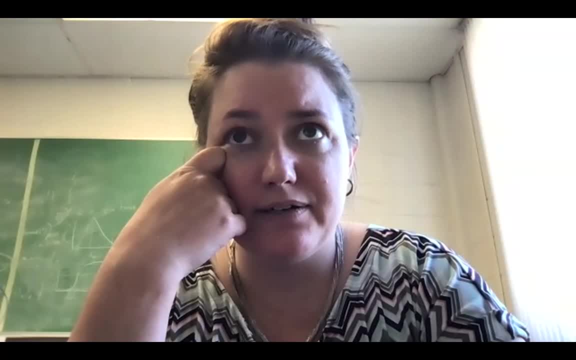 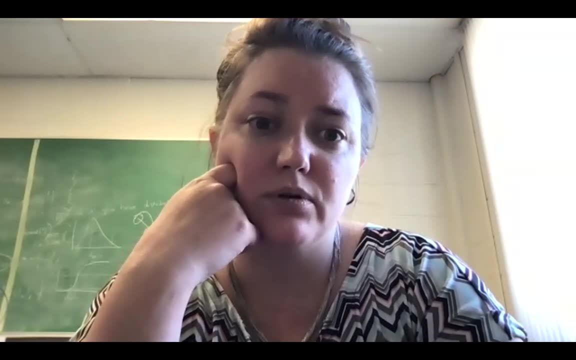 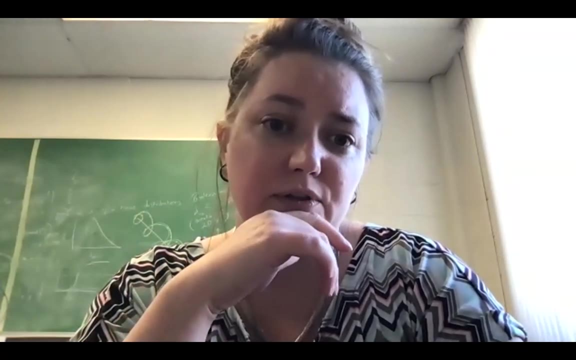 I think if you don't want to add an LMC, you can. Yeah, I think if you don't want to add an LMC to your model, you'll probably have to use a more flexible model, like the basis expansions that we're trying out right now. 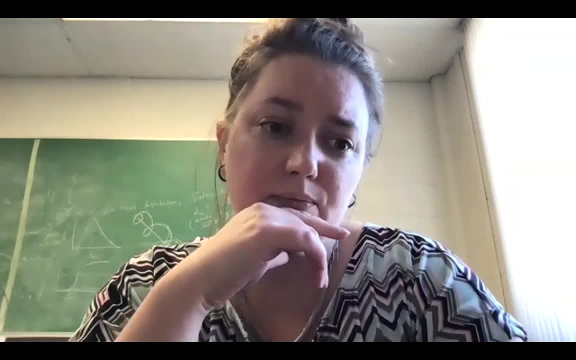 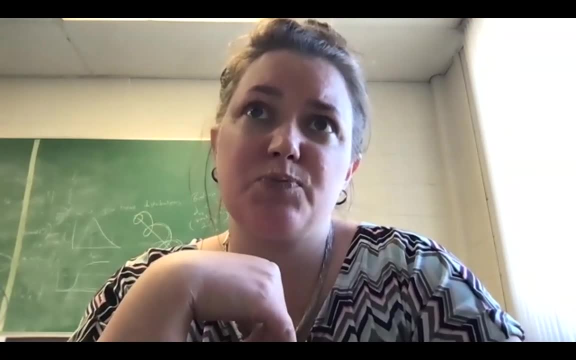 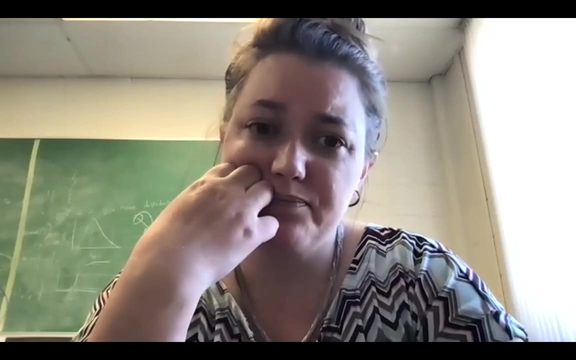 Those seem to do better with the presence of an LMC nearby. You can push them further with the actions-based modeling approach. What's interesting is that it doesn't really spread out the clumps so much as it moves them around to have. So you still maintain some of the features of action space.